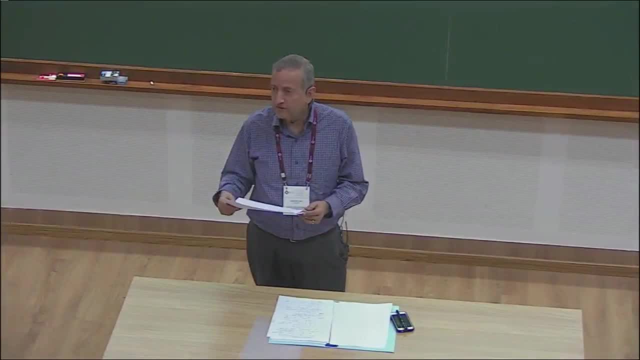 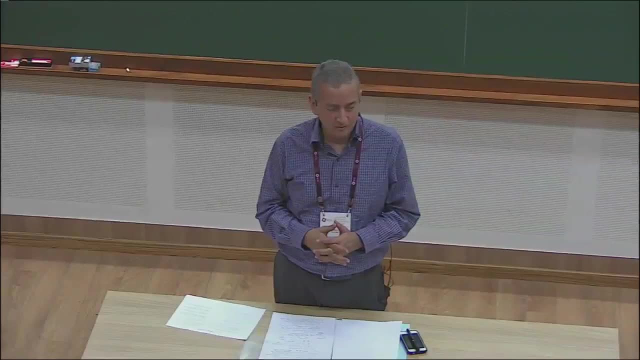 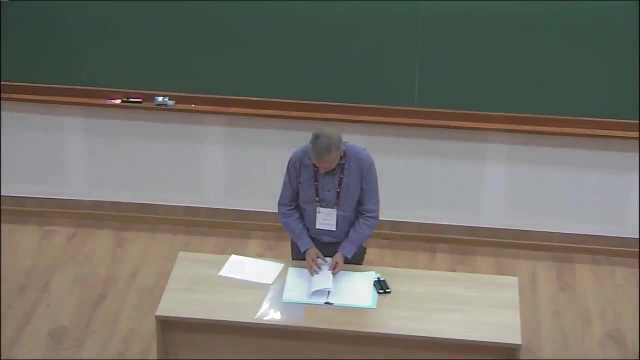 you should have received a problem set, and maybe some of you received it earlier by email. No, Okay, So anyway. so what I would like to do is to tell you how to understand the problem of the integer quantum Hall effect. So, just to remind you, we learned that from: 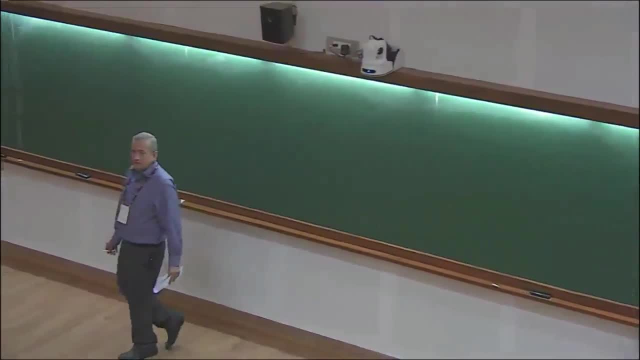 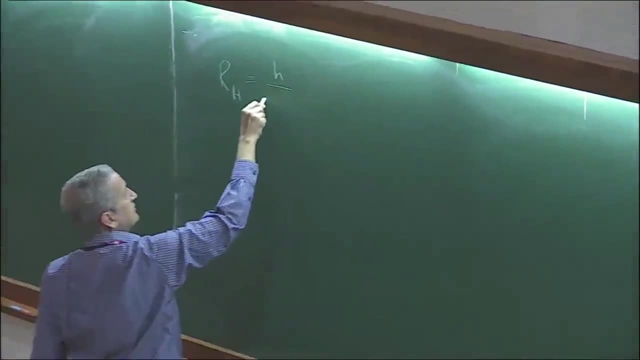 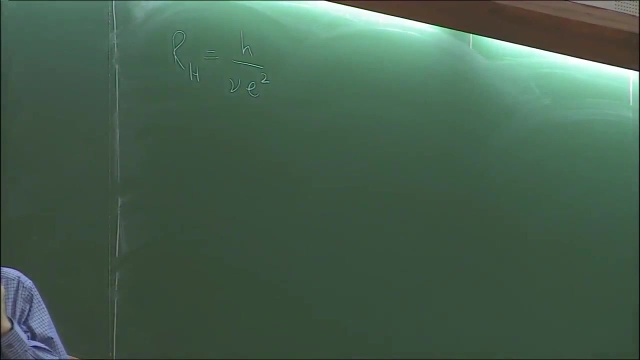 very general arguments, we can show that the Hall resistance is h over nu, e squared on a system which has translational invariance. Okay, so this follows very generally, And the question is: how do we understand the existence of plateaus? So you remember. 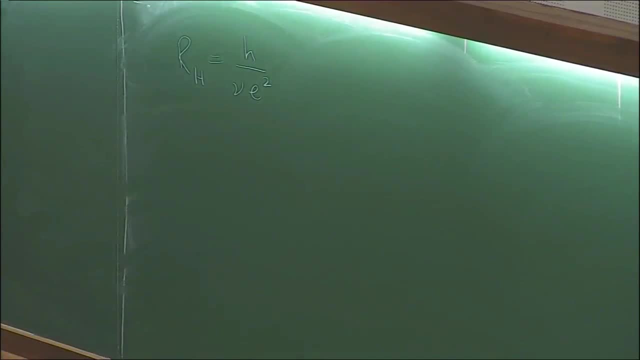 again to make sure we understand the puzzle. the experiment looks like this: As we are varying d, d goes like this: Okay, Okay, So this is the inverse of the filling factor. So we are varying the filling factor And. 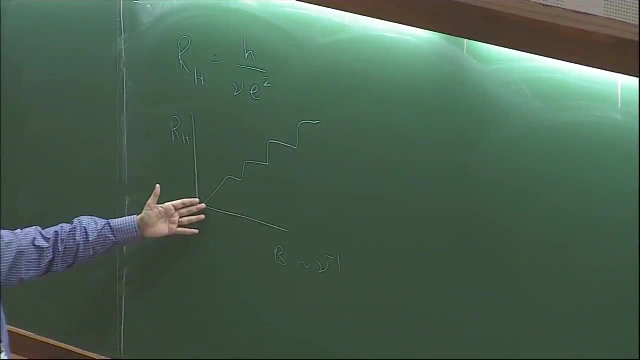 a plateaus means that there are regions of the…there are regions where the Hall resistance does not depend on the filling factor. it is just completely invariant to changes in the filling factor. So that's what we would like to understand. So there is a neat and 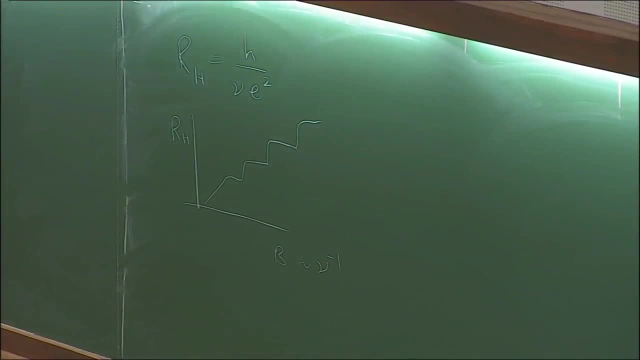 complex problem to see here explanation by this by Laughlin, It's called Laughlin's Gauge Argument And this has a topological flavor, as you'll see. In fact, the quantization of the Hall resistance can be understood as a topological quantity because, as was explained earlier, 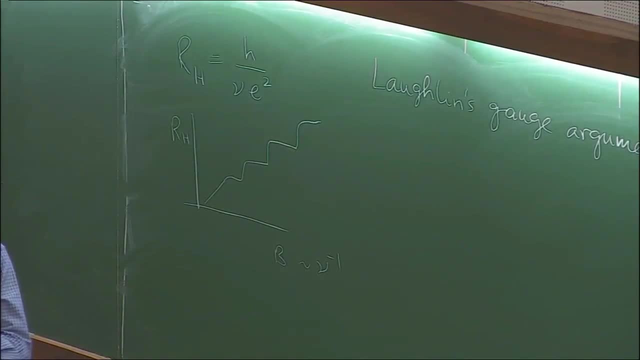 by Jadeep. topological quantities have the property that they are invariant under continuous changes in the Hamiltonian. So as we are changing the filling factor, we are changing the Hamiltonian, but the Hall resistance does not change. So you can see that it is a topological object. 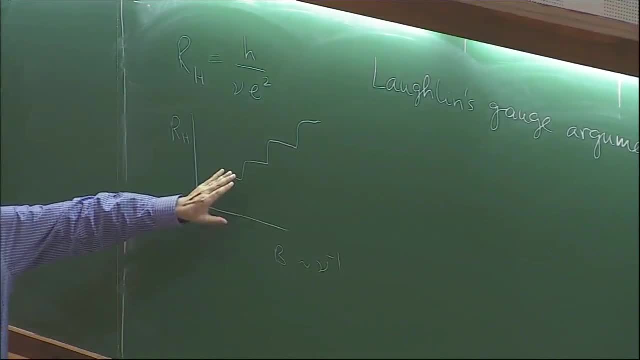 and indeed one can understand it in a topological fashion, And this is one way to do that. So we are going to do the following. First of all, let me consider a sample like this: This is the x direction, And what I will do is I will do a two-step calculation. The first step would 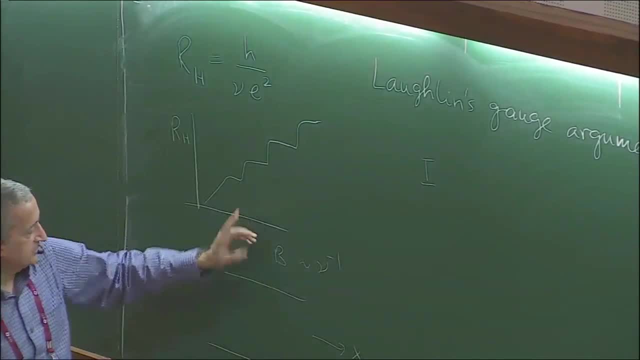 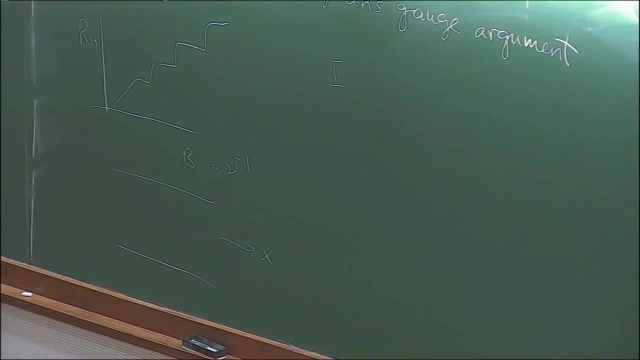 be to do the calculation for a system precisely at an integer filling and obtain the result that I had shown earlier. So that's a more complicated way to do the calculation, if you wish, But then we will see how the result remains unchanged even when we put some disorder or even when we 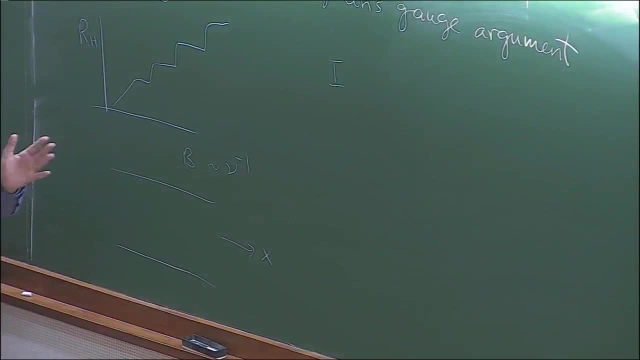 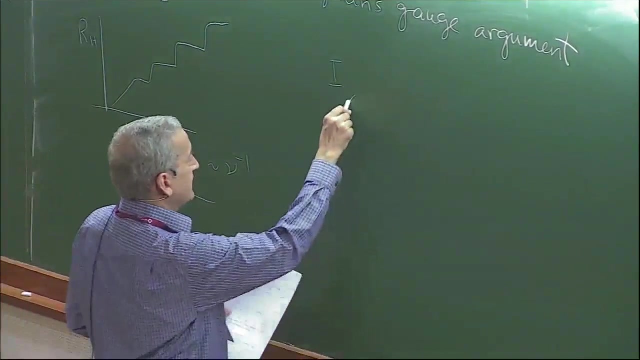 change the filling factor away from the special value. Okay, So let's first imagine that we are looking for a type of x and y. So this is our sample And what we do is we will do. we have no disorder and I want to write the current in the x direction. so current in: 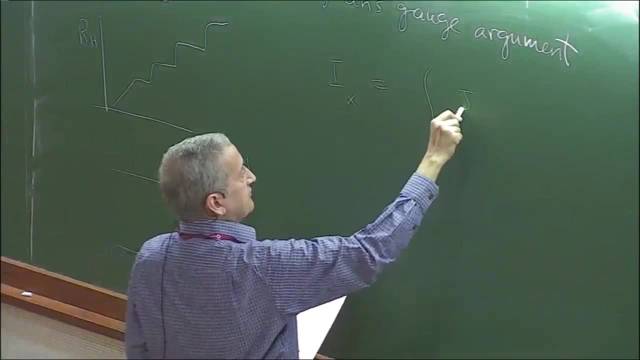 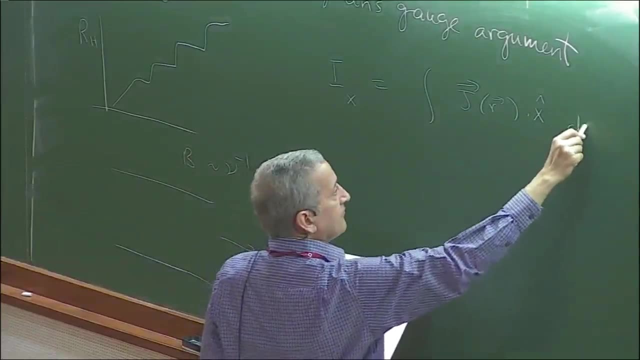 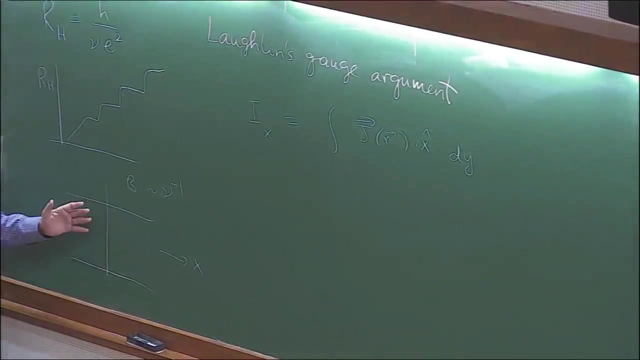 the x direction will have so if this is my current density. so I take a line like this and calculate all the so from the current density in the x, I take the x component of the current density and integrate over this line, that's the current going along the x. 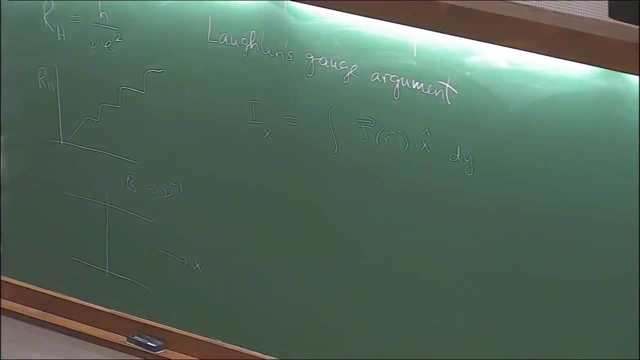 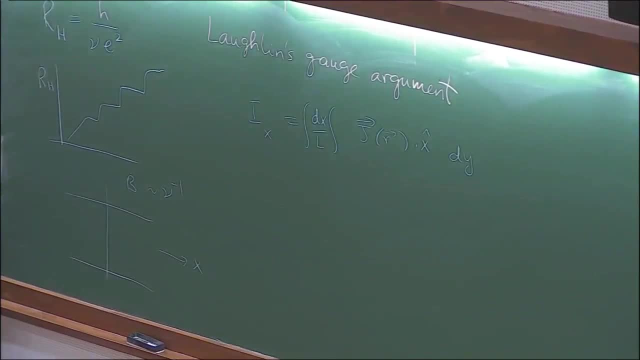 choose a line at any point along the x direction and I get the same answer. so the result does not depend on x. therefore I can integrate for simplicity also over x, but I need to remember that I divide by the length of the sample. 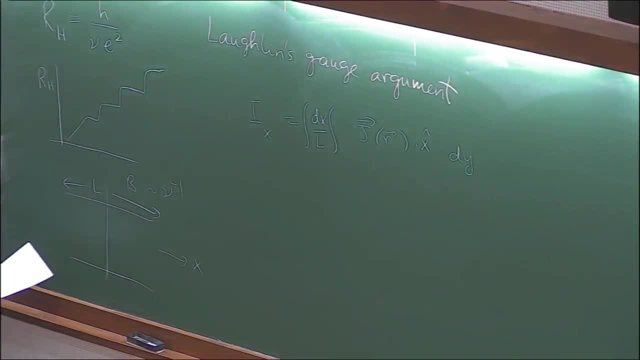 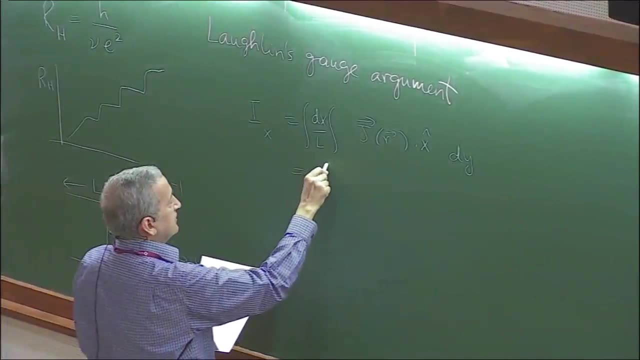 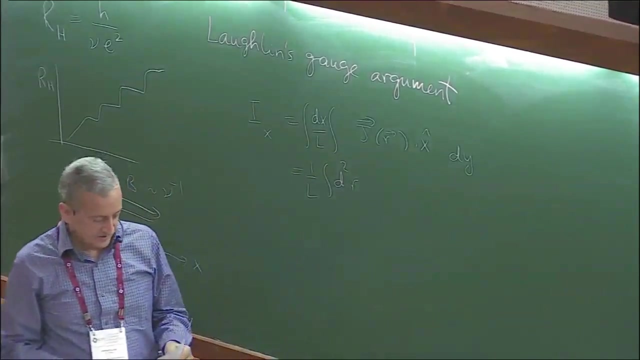 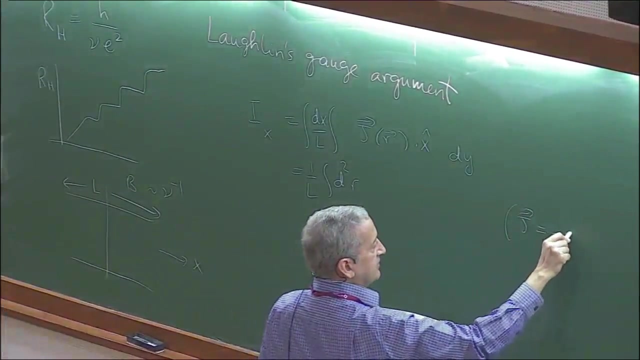 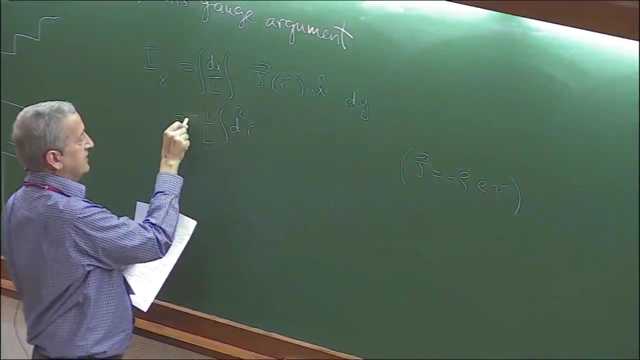 so let's say this is the length of the sample and that I need to know what the length of the sample is. so let's say that I need to get the length of the sample. So the length of the sample is x. so I have that. this is the length. this is my jx. j has the formula that, remember, j is minus rho, e, b, so it has the formula. there's a negative sign, but I'm not going to be very careful with the signs. there is an error. 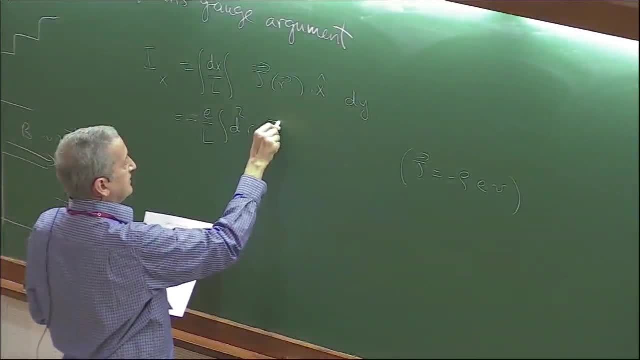 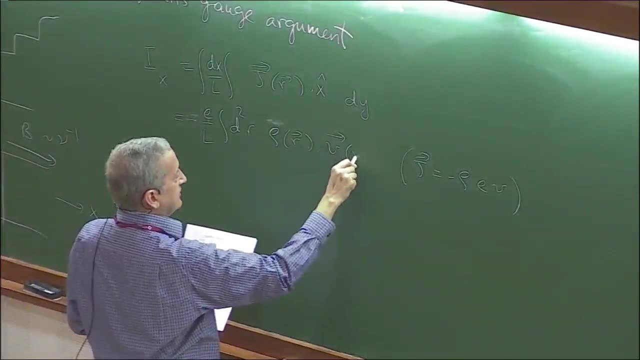 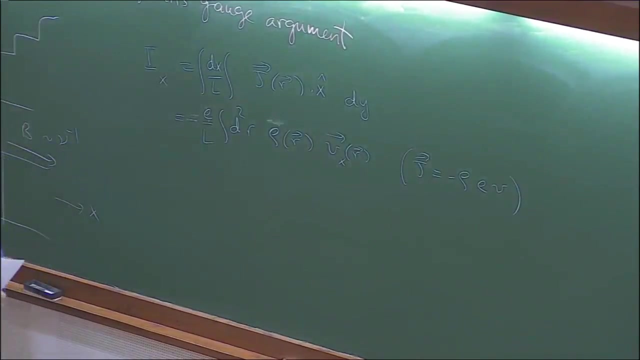 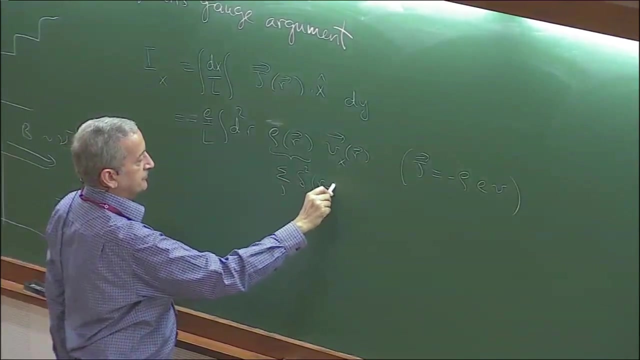 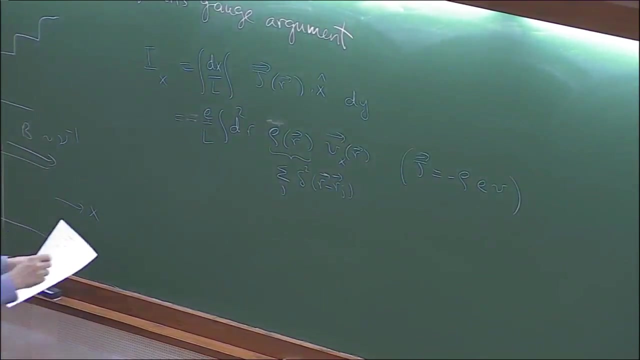 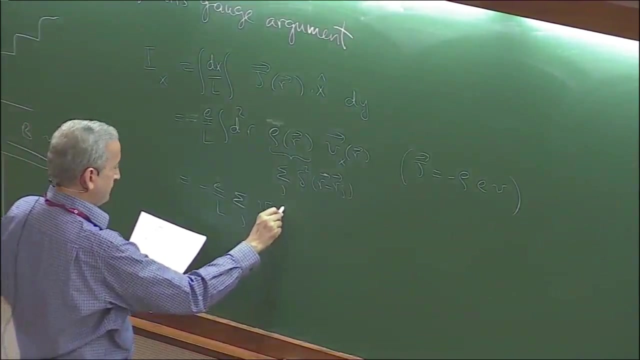 an E, there is density and there is the velocity along the x direction. Okay, so that's just the current along the x direction. Now I am going to write this density as sum over J and then I am going to do the integral, So I get this formula. Okay, so that's the current. 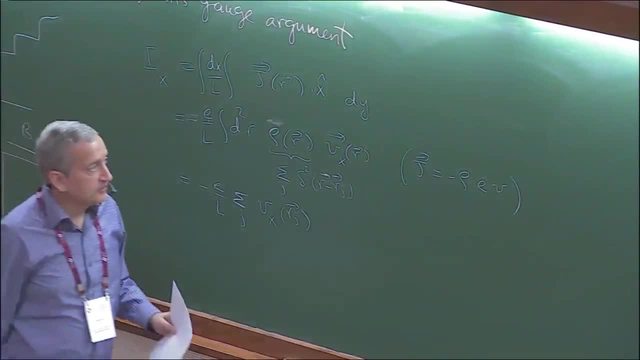 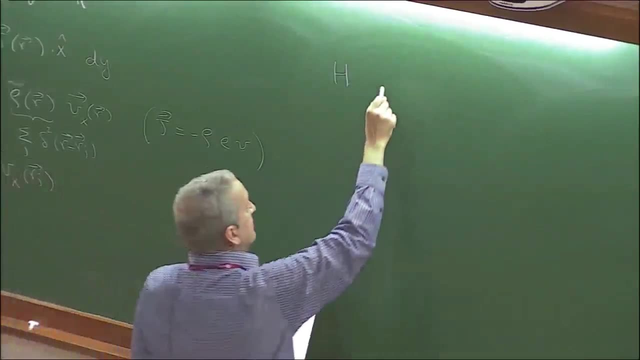 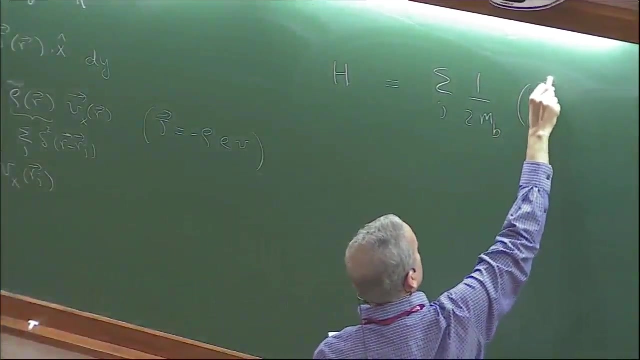 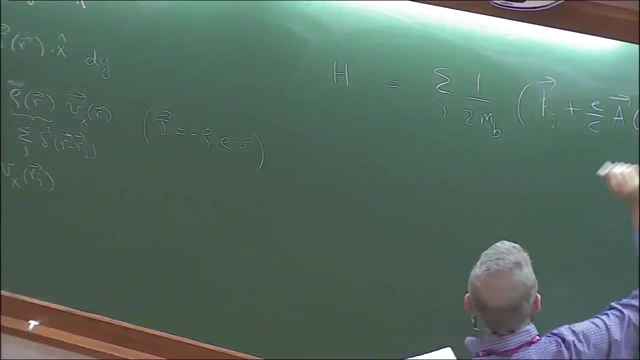 Now, how do we calculate this? So let's go to the Hamiltonian and we had earlier, we had already done this. Okay, so I am not worrying about the interactions yet. It's a Hamiltonian for non-interacting particles, But I am going to insert a test vector potential. 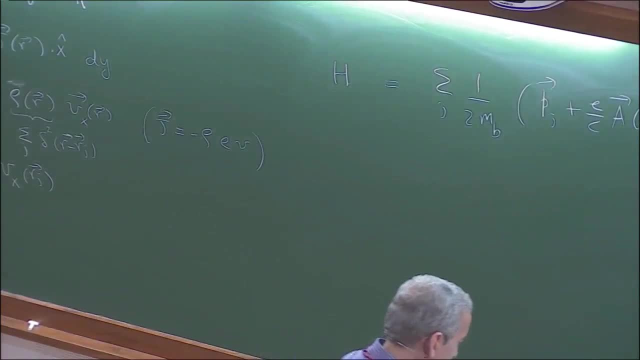 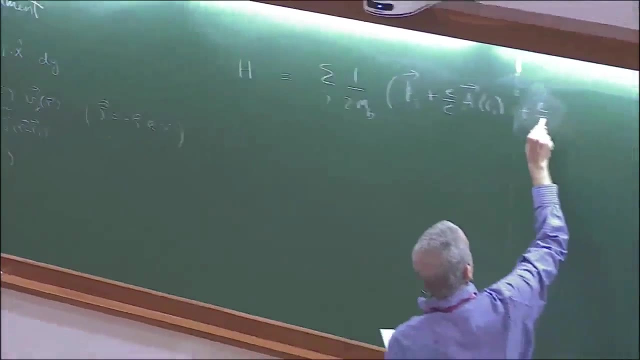 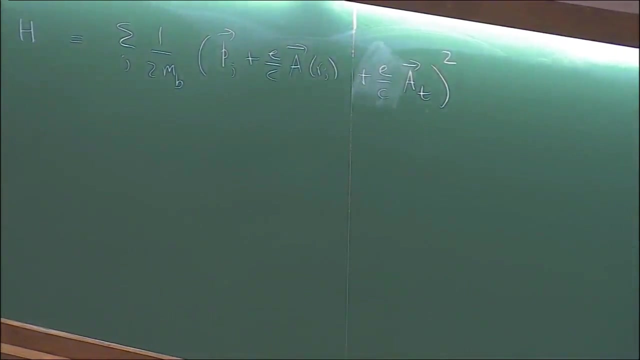 which will allow me to do the calculation, And I am going to insert a vector potential which will allow me to do the calculation. And I am going to insert a vector potential which will allow me to do the calculation. So let's insert this text: Test vector potential here. So the T here stands for test And furthermore, 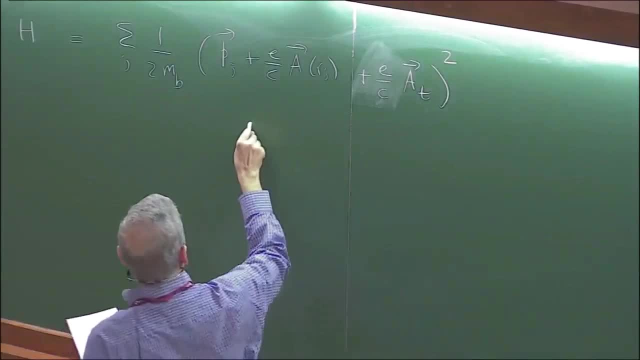 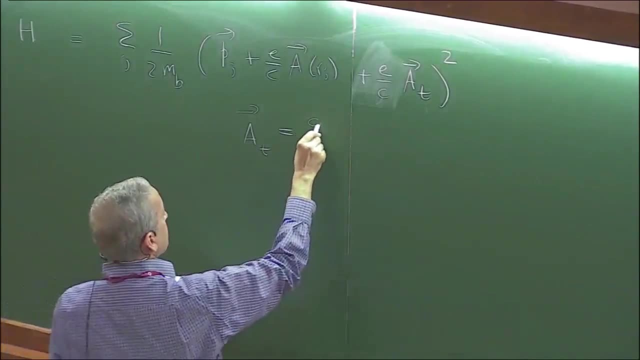 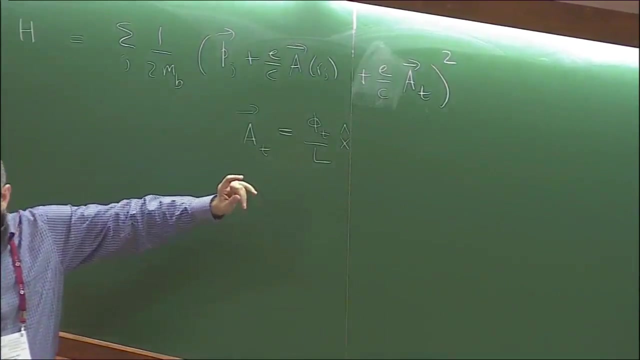 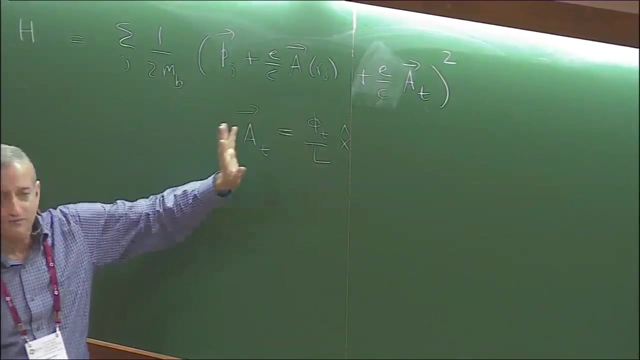 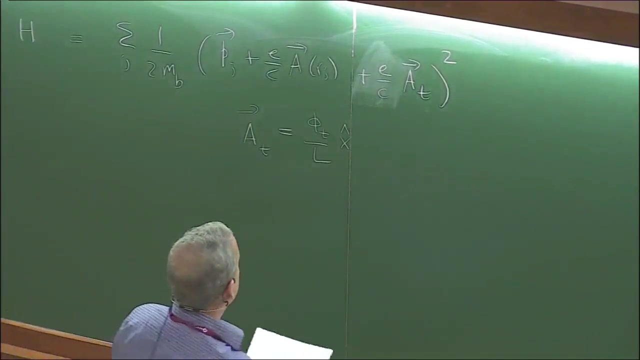 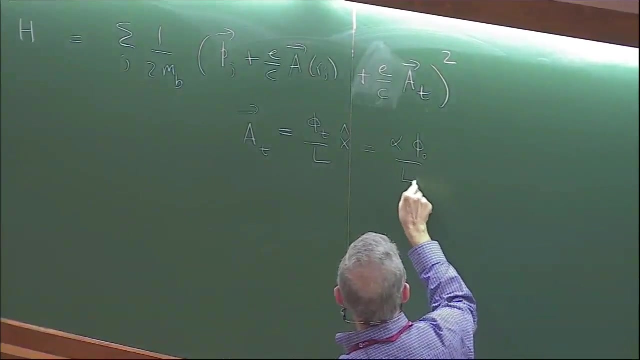 I am going to assume that this A test is. So it has this form: it's pointing along the x direction and it's phi t over L. phi t is some fixed quantity, In fact. I'm going to take the test flux to be. I'm going to measure the test flux in units of phi naught. 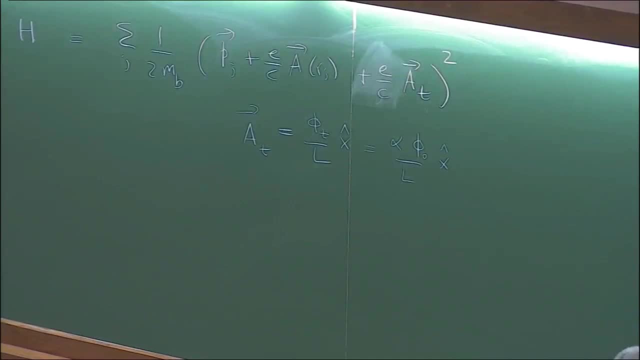 So I will say that the test flux is alpha phi naught. So there is a nice interpretation for this because of the following: Remember, we had assumed periodic boundary conditions for this sample, So what that means is that this sample effectively has the topology of: 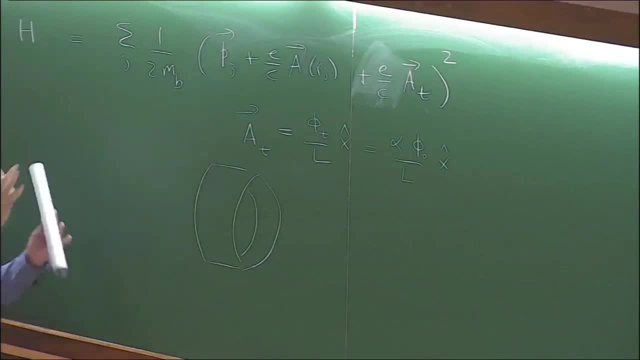 obviously the topology of the sample. So what that means is that this sample effectively has the topology of this type of a ribbon like this. And if you ask what is the flux through the ribbon- I mean through this cylinder- then integral, if I integrate over the flux like this: 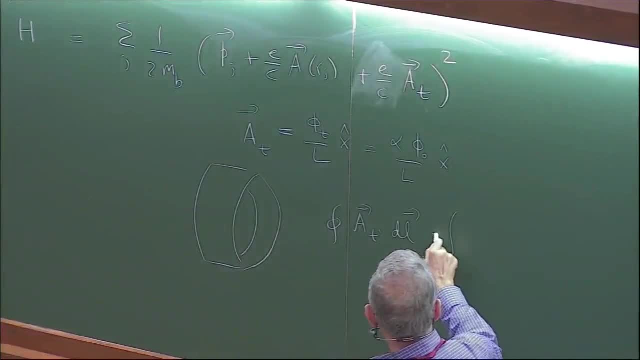 and I take DL to be along this, so it's the x direction. Then integrating all the way around is: it just gives me a factor of L and this is alpha phi naught. So this test flux that I have inserted here into the Hamiltonian 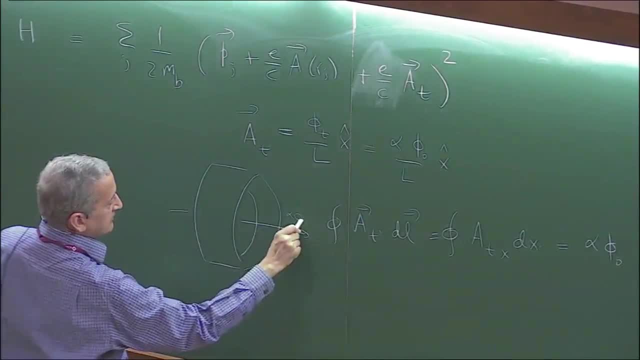 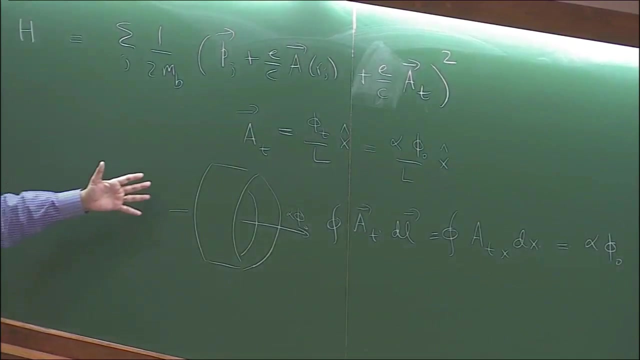 it corresponds to a flux, alpha phi naught passing, passing through the cylinder, passing through the axis of the cylinder. So why are we doing this? Well, for the following reason. So I'm going to come back here and I'm going to say that this thing- 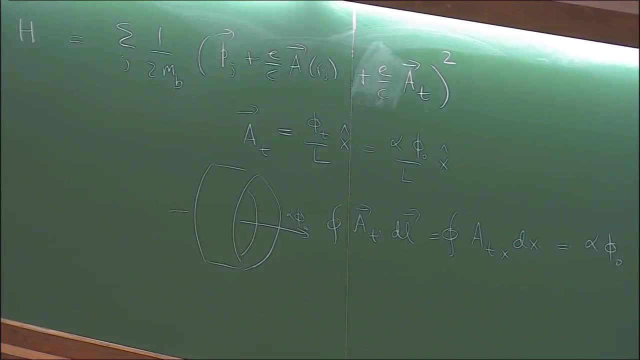 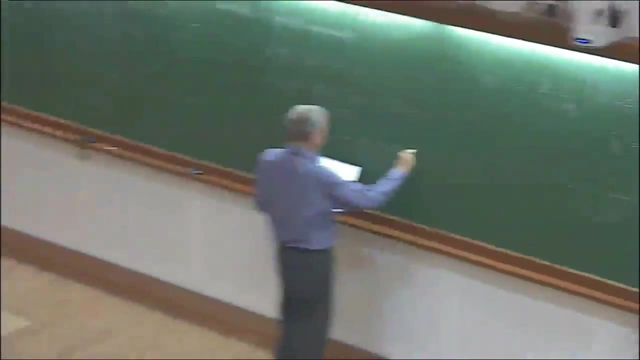 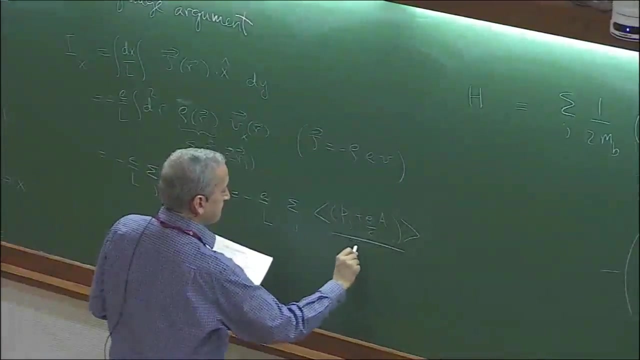 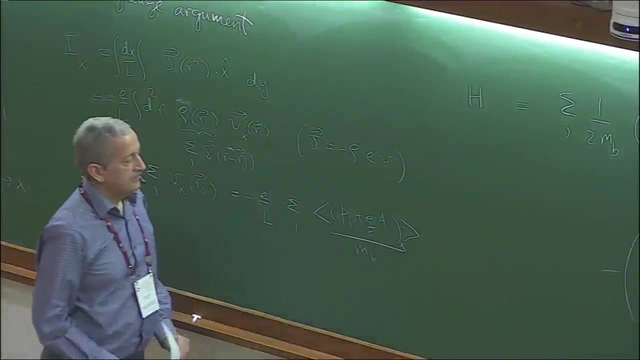 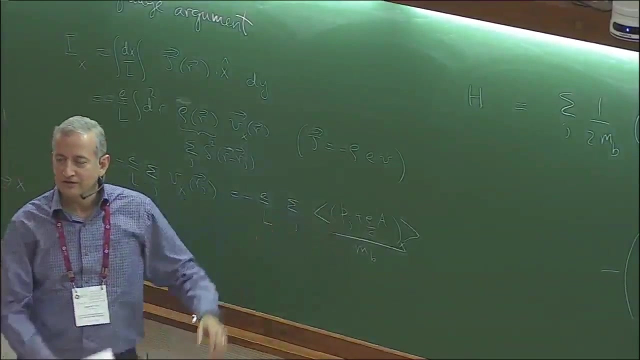 so what's the x component of the velocity? Okay, It's a. So the x- I mean the velocity in the presence of a magnetic field- is given by this, and we take the expectation value of this quantity. Now I can write it in a nice way, but I'm not going to write it in a nice way. 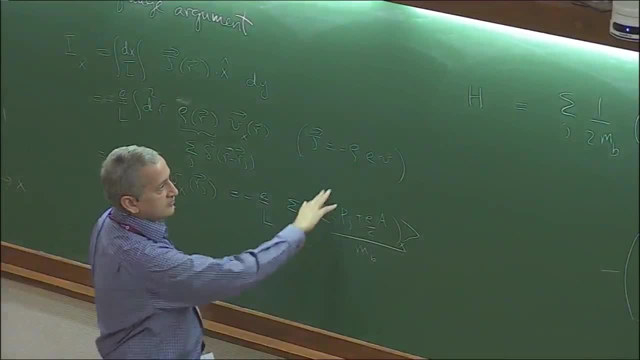 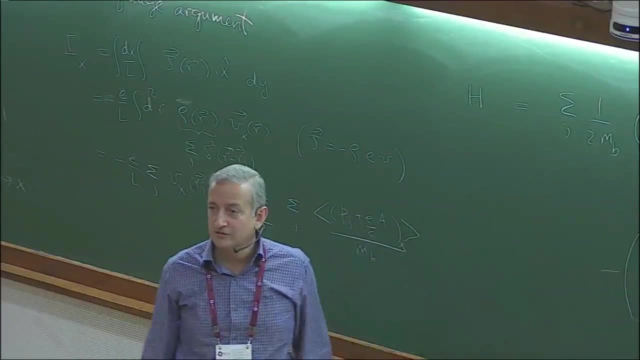 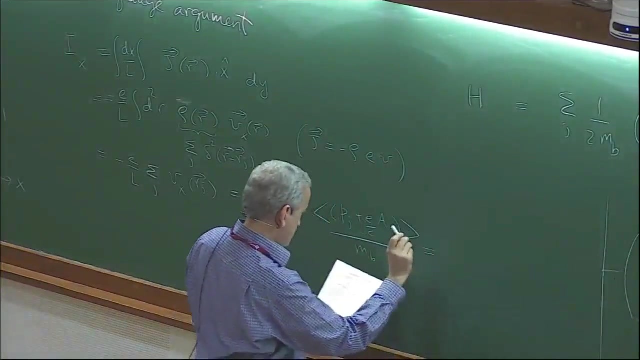 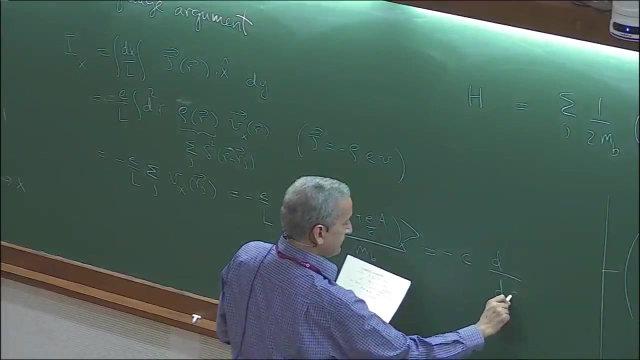 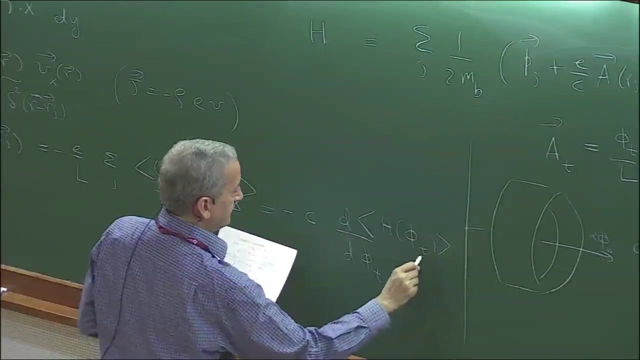 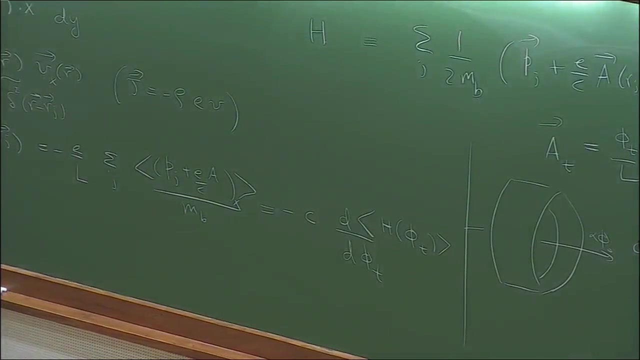 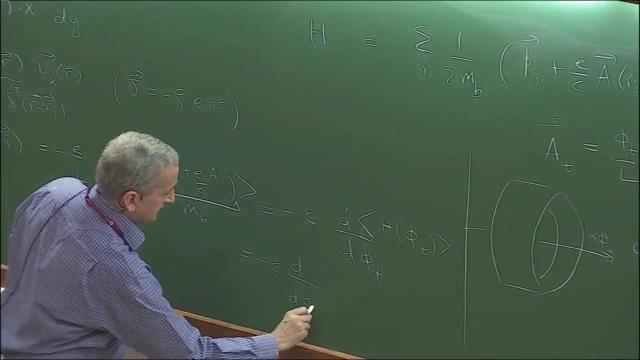 Because this thing, this quantity, is related to the Hamiltonian, if I take derivative with respect to the test flux. So I can write it in this fashion: minus C, Okay. So in fact I can go a step further and I can say this is minus C, d by d by t. 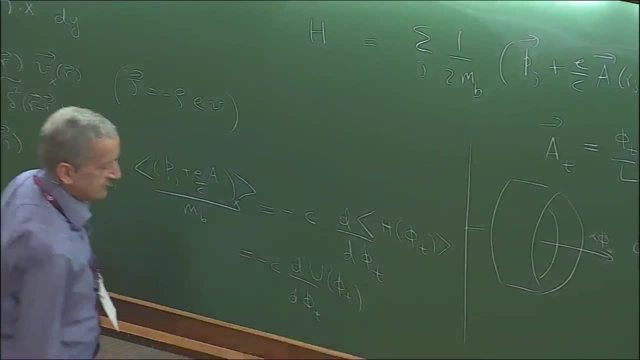 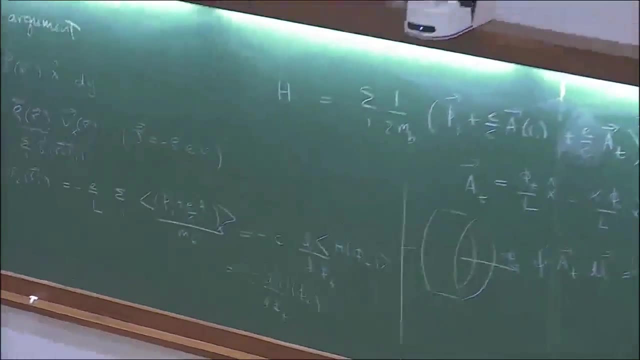 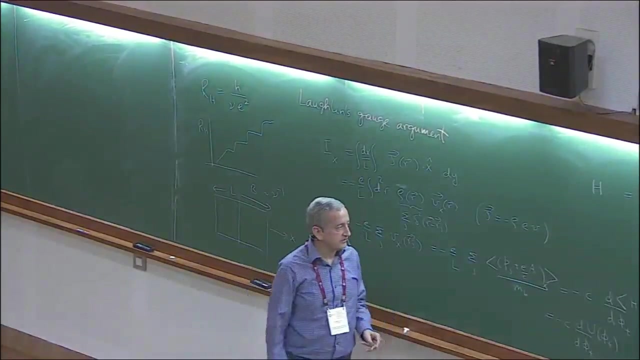 the energy as a function of test flux. So this is a way of calculating the current through the system by asking how the energy varies as a function of flux passing through the cylinder or how the energy depends on the variation on the change to boundary conditions. 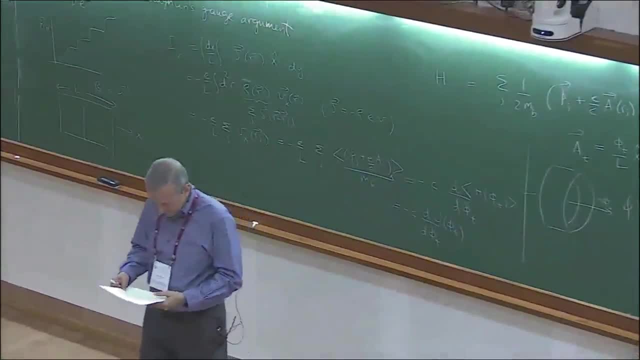 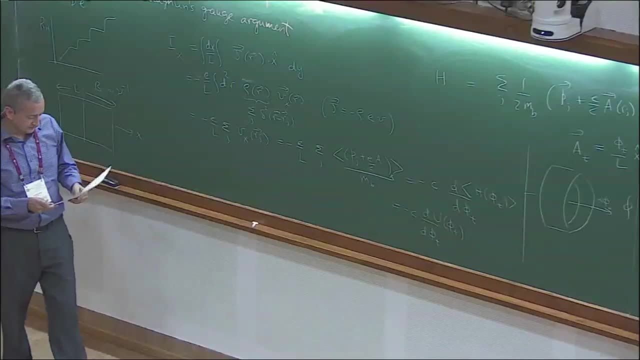 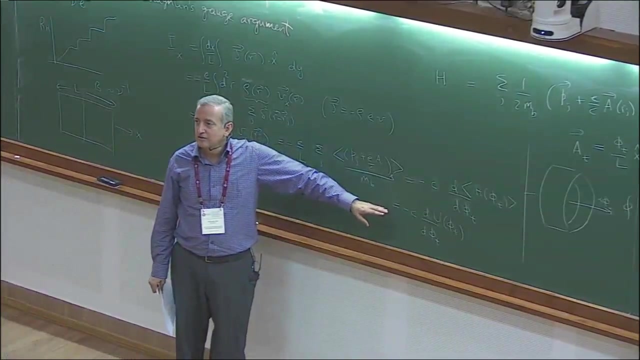 So now what this is doing is essentially changing the boundary conditions. Okay, So let's take this formula and ask what this means. So we will see that in general, this is very hard to calculate. So as we change the flux, this is going to oscillate a little bit. 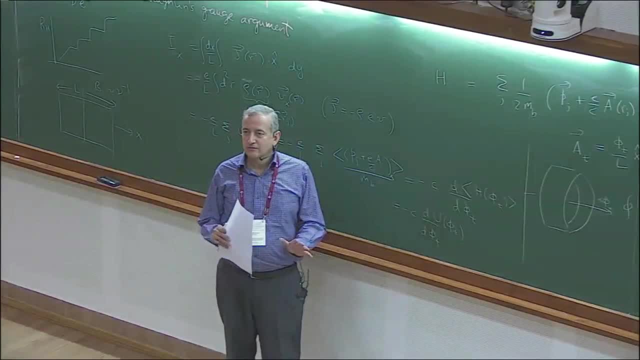 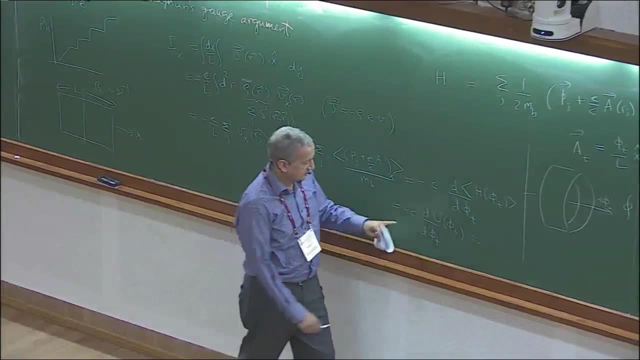 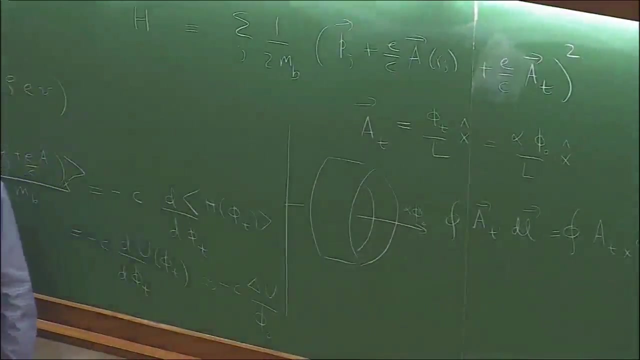 But one of the things, one of the things that Laughlin did. he said: well, let me approximate this by asking how much the energy changes When I change the test flux by one flux quantum, and we'll see that there is a neat way to calculate this quantity. 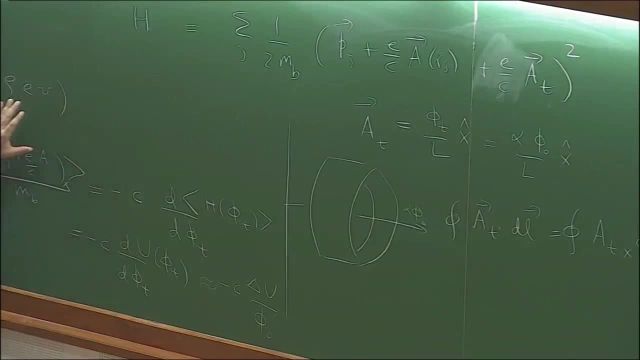 So we have approximated this derivative. So far. this is all exact up to this point, But here. so this means that you have changed the test flux by a small amount and asked: how much is the change in the energy? Now we are going to say that that small amount will take to be precisely one flux quantum. 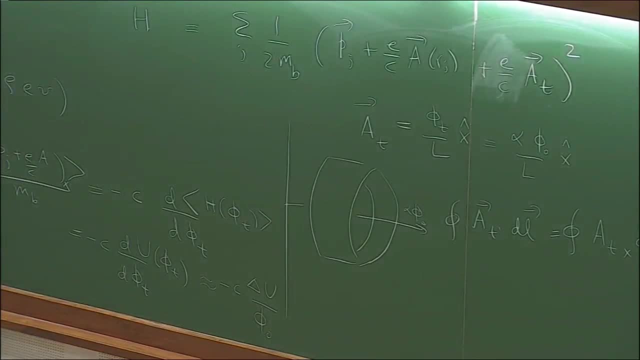 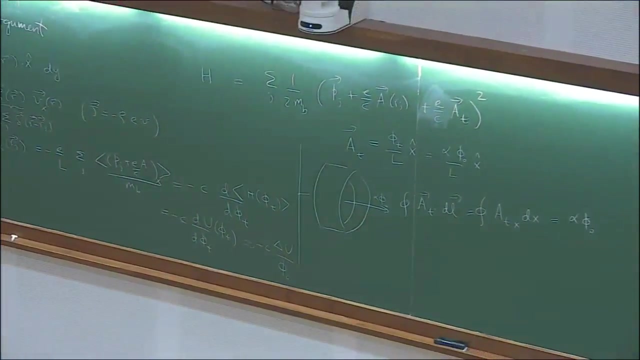 and ask: what's the change in the energy? Okay, So is this all clear so far? Okay, So let's ask how we can calculate this. So remember what the states look like. The states look like lines, And each line is labeled by a kx. 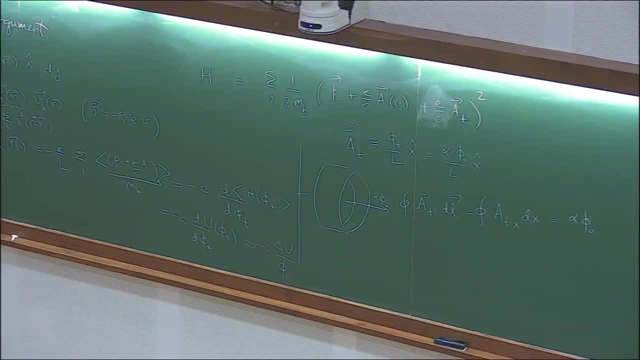 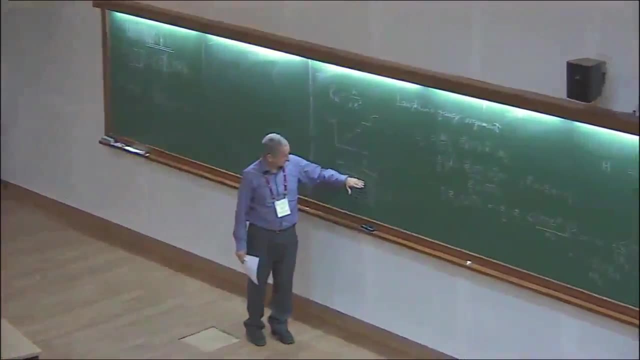 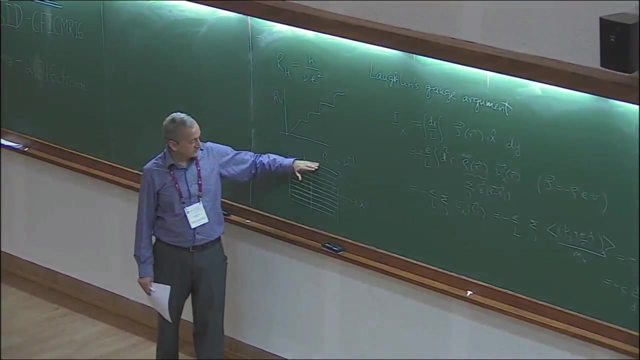 So for when we impose periodic boundary conditions, the kx wave vector takes some discrete values, as we saw last time, And these are the discrete values. So these are ordered single particle states with each one having a kx label. So the question is: as I change, so this would look like this here. 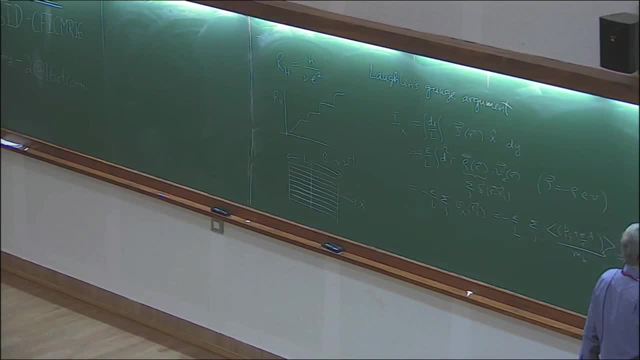 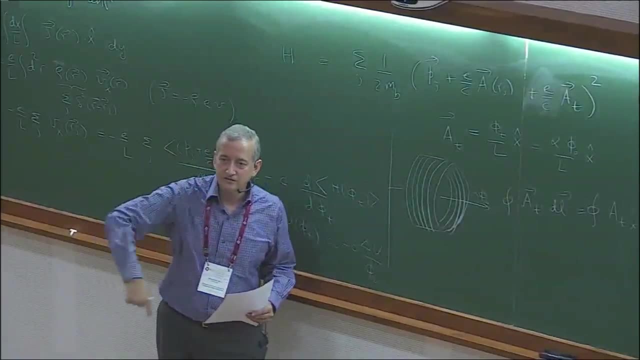 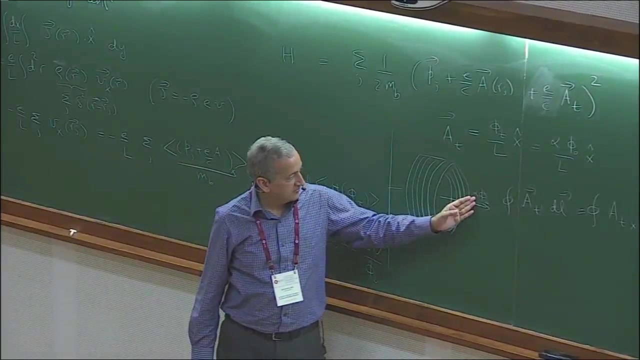 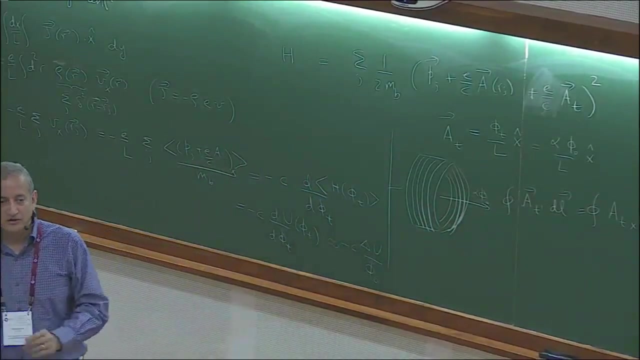 So all of these single particle eigenstates, they go around and the question we are asking is: suppose I change alpha or suppose I change the test flux from zero to one flux, quantum, idiomatically slowly. what happens to the system and what is the change in the energy? 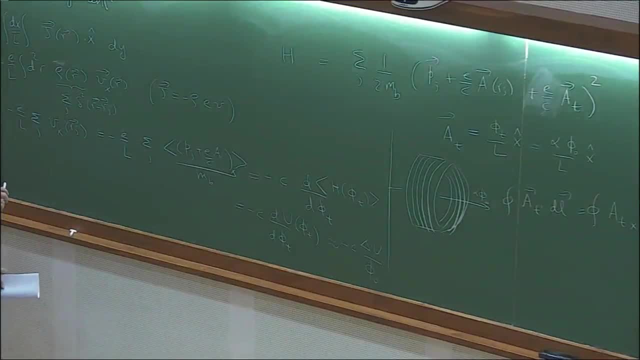 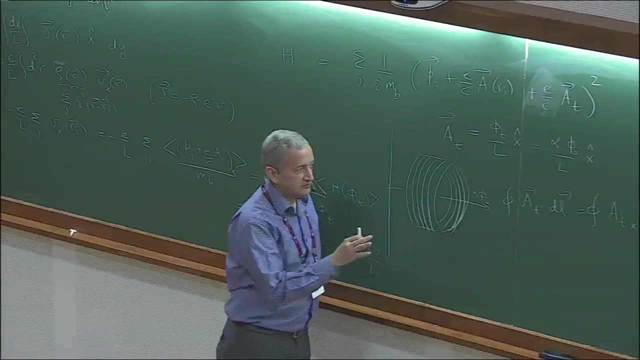 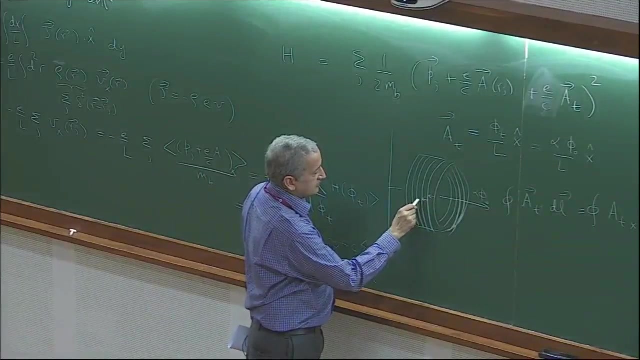 So the result? let me tell you what the result is and then tell you how to understand the result or how to derive the result. the result is that as we change the test flux by one unit, this eigenstate moves to this. this eigenstate moves to this, this eigenstate moves to this: 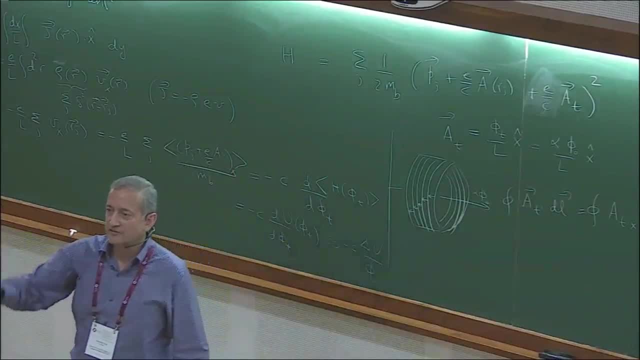 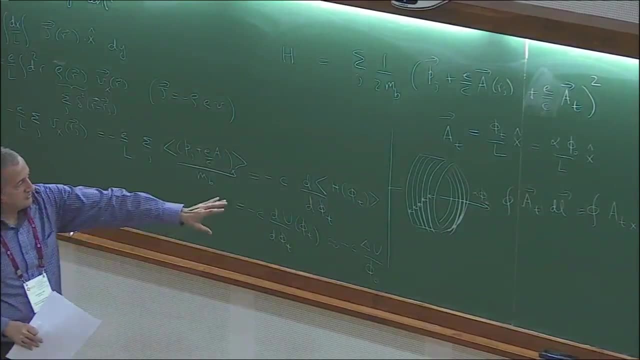 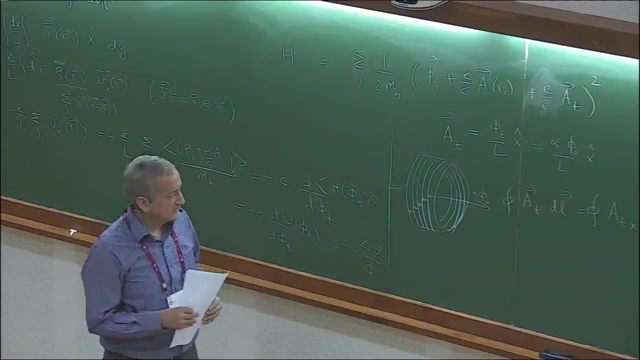 this to this, this to this, so each eigenstate moves to the next eigenstate. So let's see how, and therefore, so let me also derive the result: or in the presence of disorder, or in the absence of disorder, when the filling factor is precisely: 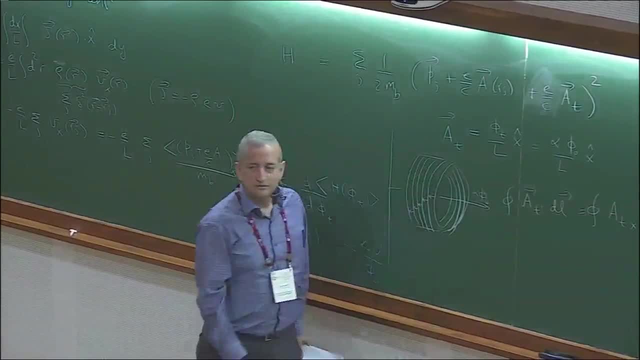 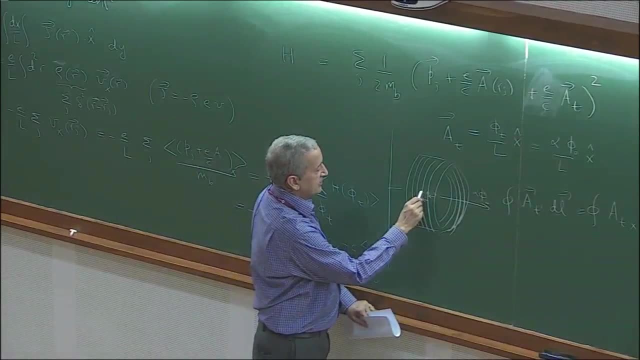 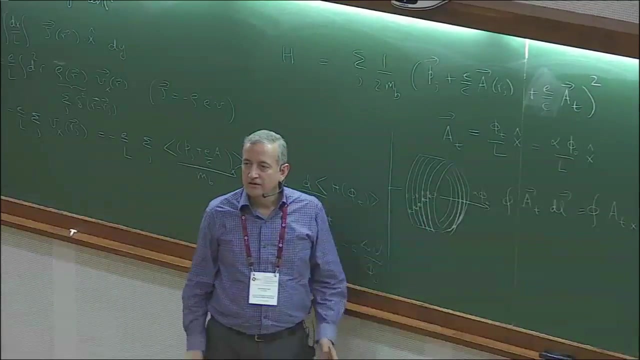 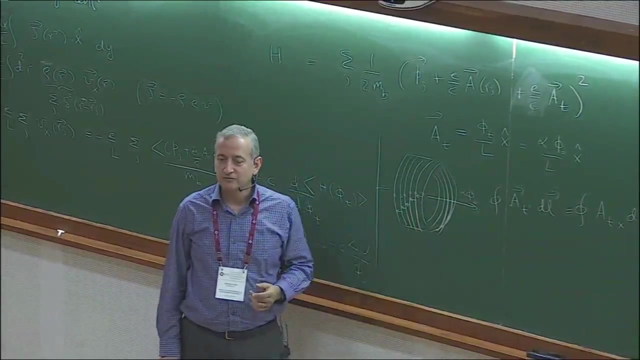 n. So let's say all of these states are occupied. so if all of them are occupied, so each one is carrying an electron, and when each state moves to the next state, then the electron moves with it to the next state and eventually the effect of piercing one flux quantum is. 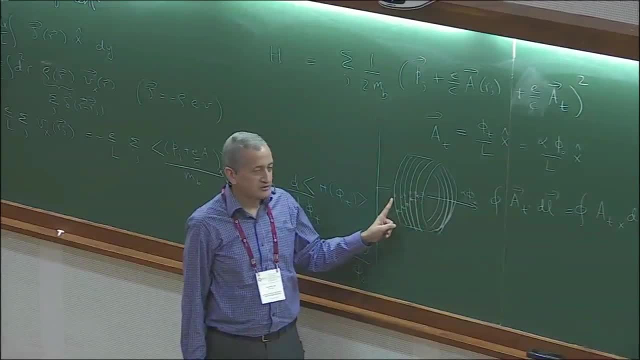 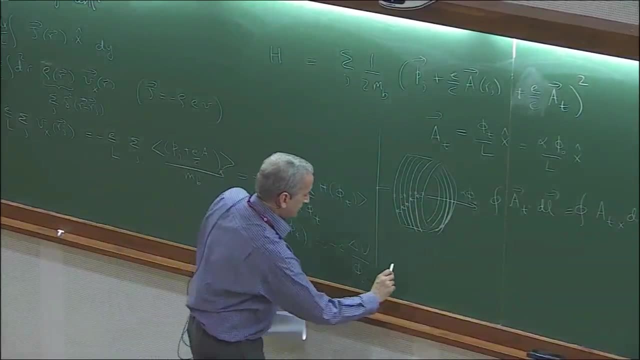 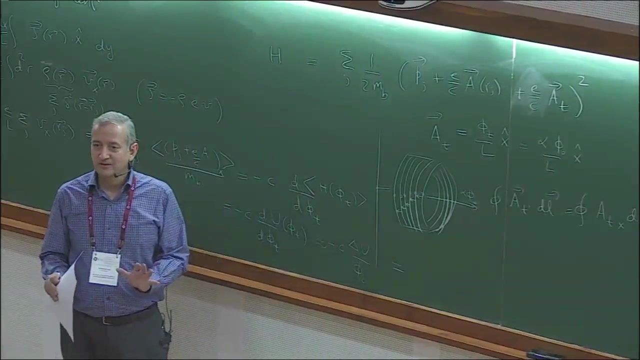 that we have taken one electron on one edge and moved it to the other edge. That's what we have done. So, therefore, what is delta u? So, again, this is. you know, this is the first step of this argument where we are deriving. 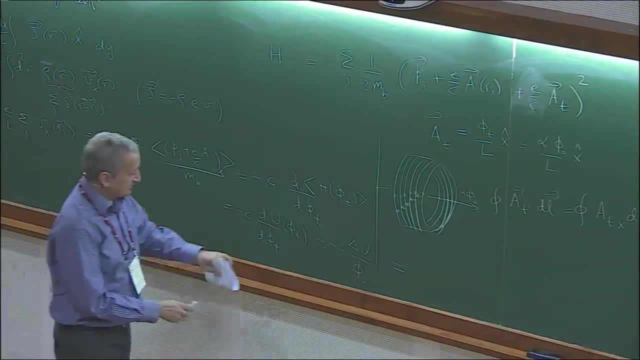 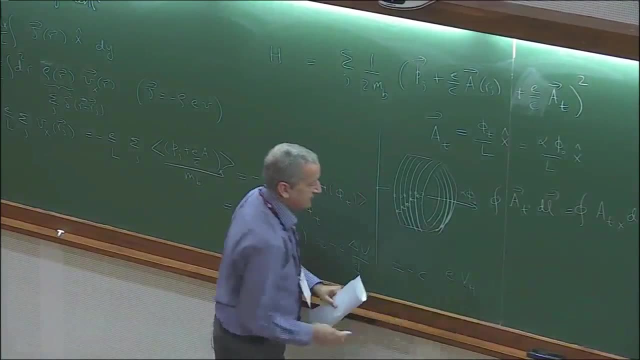 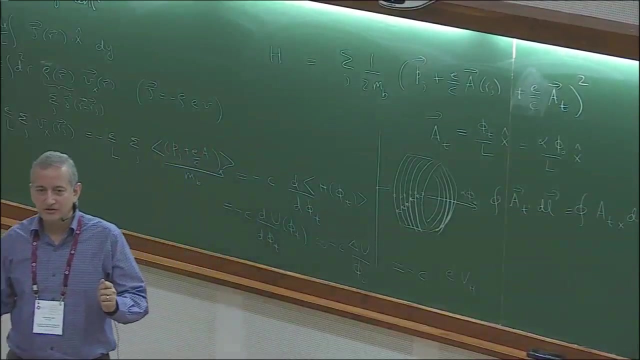 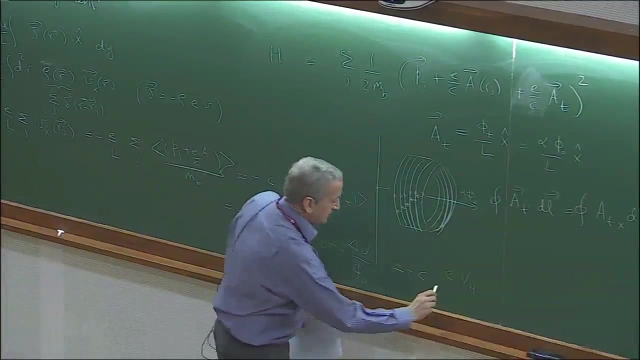 a result that we knew earlier By a different method. So delta u is simply e times Hall voltage. It's e times the chemical, the difference between the electrochemical potentials between the two edges, which is precisely what the voltmeter measures. And if there are n lambda levels, then the same thing happens in each lambda level. 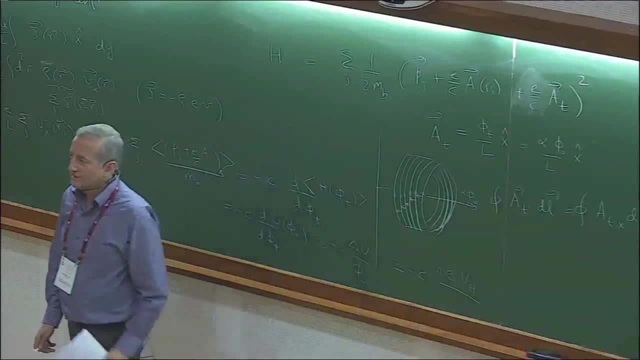 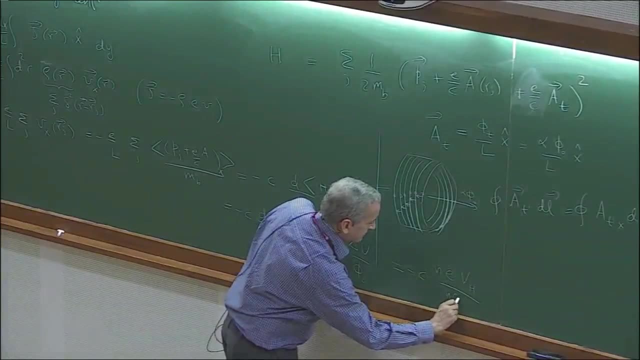 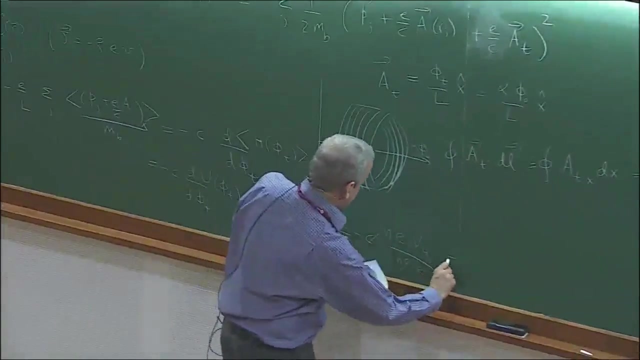 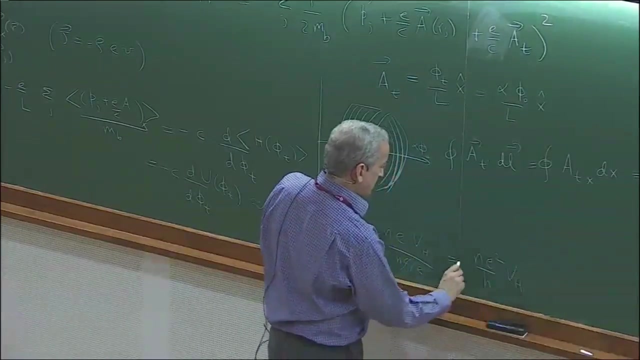 So that would give a total change in the energy which is n times e times Hall divided by phi naught, which is hc over e. So you see, c cancels out and we find a result which is n, e squared over h, vh, And this gives us Hall resistance. 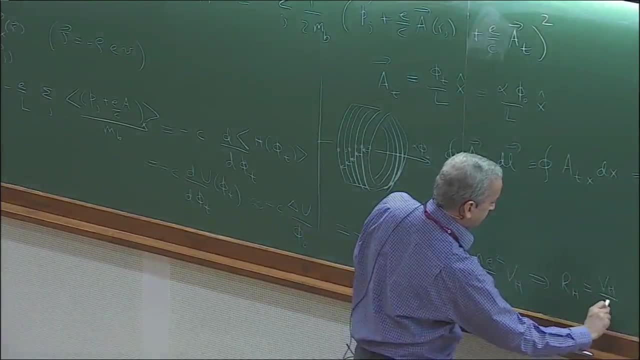 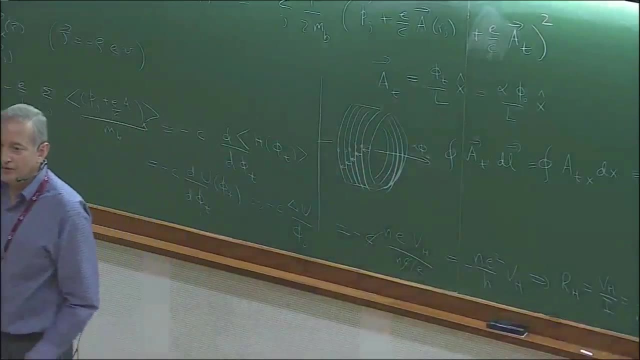 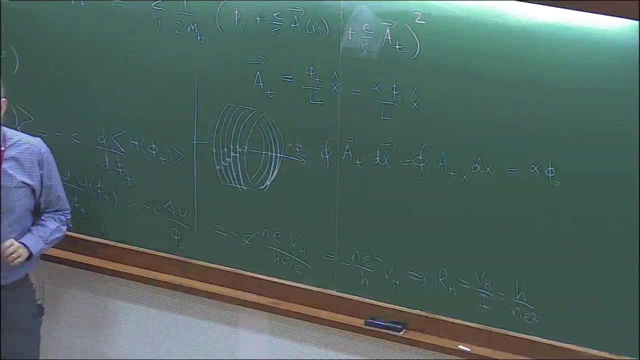 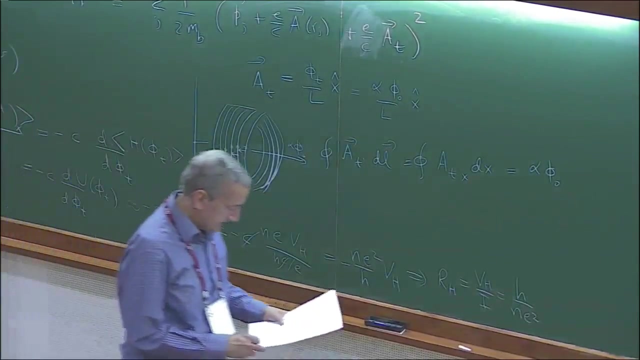 So this is e squared over h. This is e squared over h. Ok, So here I have assumed this result, that each state moves to the next one. Let's see how we can derive this result. So the derivation is fairly straightforward for the system, which has no disorder. 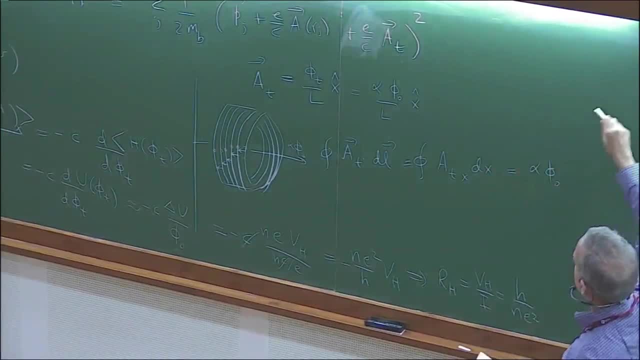 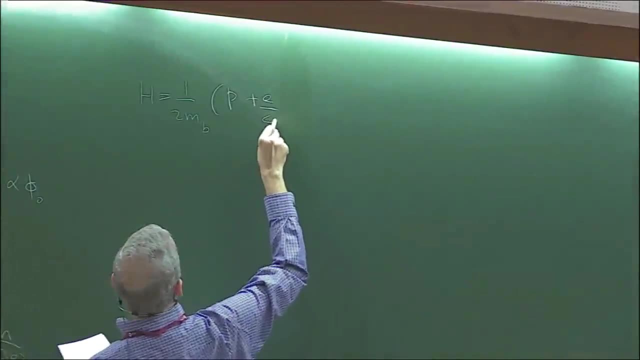 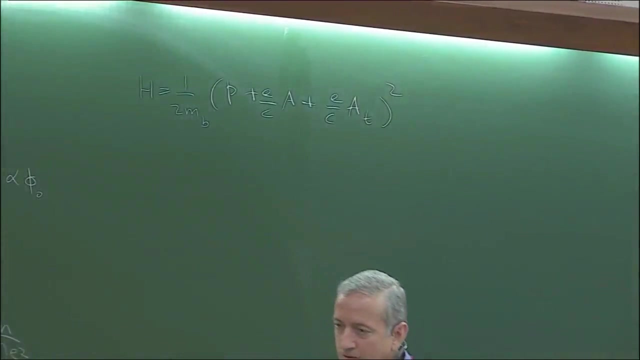 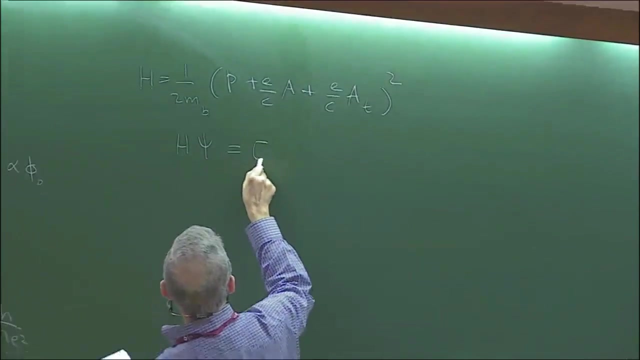 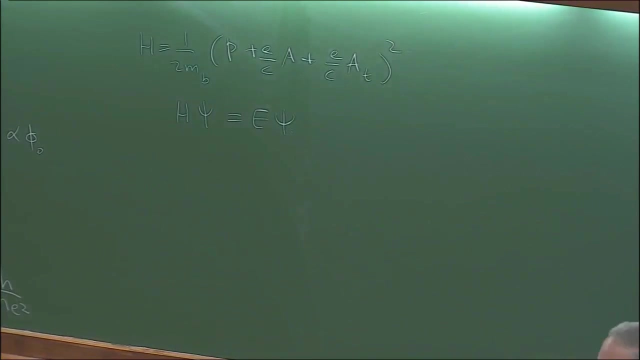 So again, I take a signal. So what happens when I remove the signal? single particle Hamiltonian. Okay, And I want to solve the problem: H psi equals E psi for this. So you know earlier we did that without this term. We know how to do it without this. 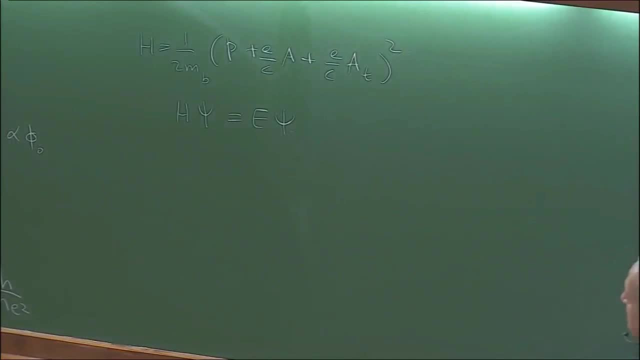 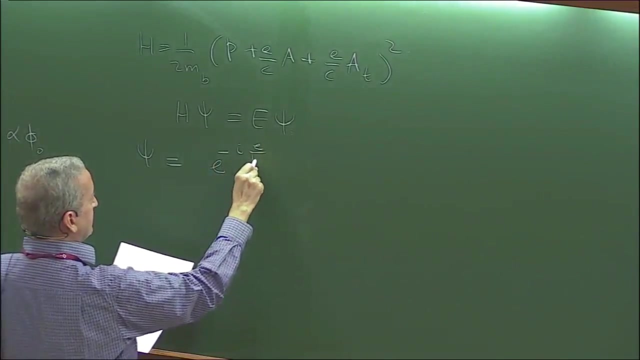 term. The question is, what happens to the Hamiltonian when we have this extra term? It turns out that the solution that we had earlier also applies to this problem, after a little gauge transformation. So let's make a gauge transformation where we replace psi, which is the physical wave function of the system, by e to the power minus i, e over h bar c. 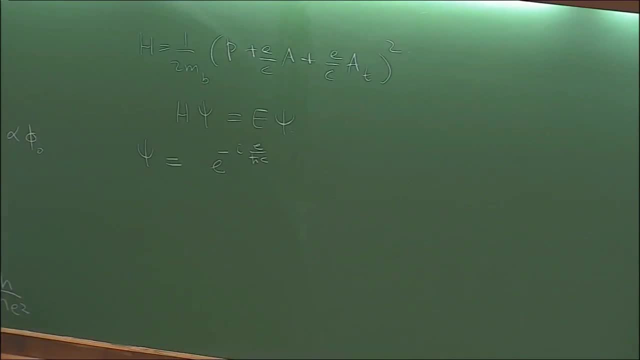 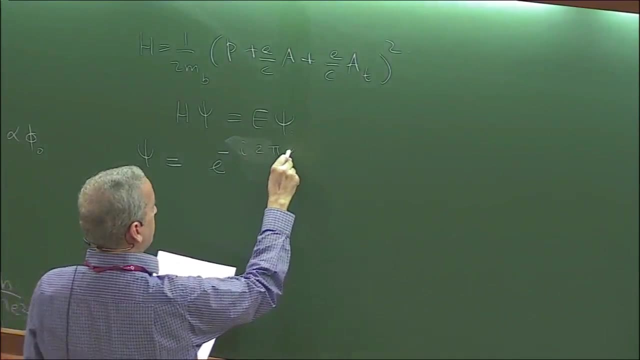 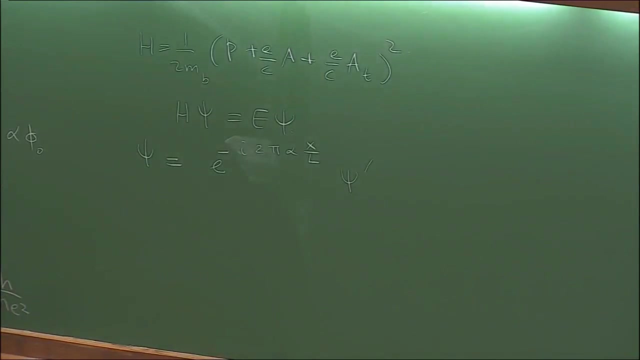 Or let's: Okay, So let's. Let's make the substitution in this equation So when the moment of operator acts on this, it produces an extra term which precisely cancels this part. So the new problem that we have is H prime, psi prime equals E psi prime, where 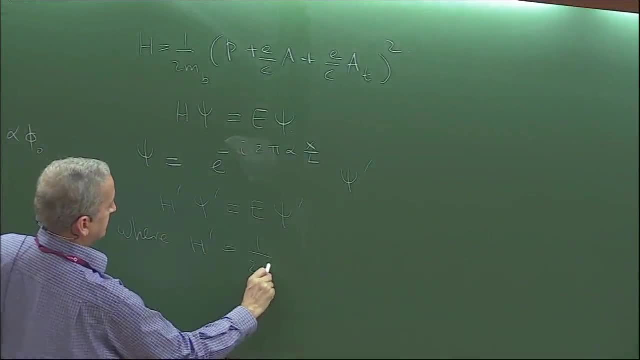 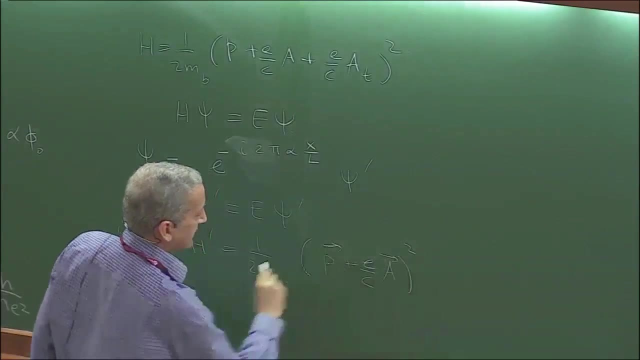 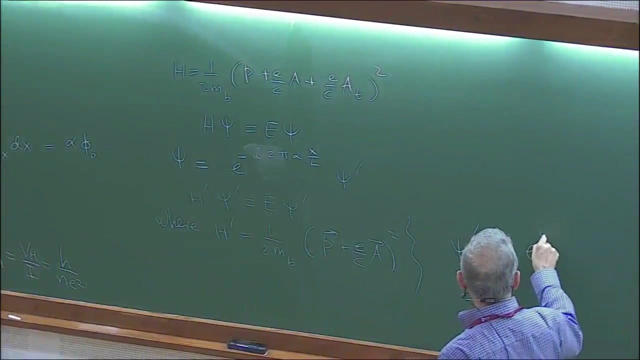 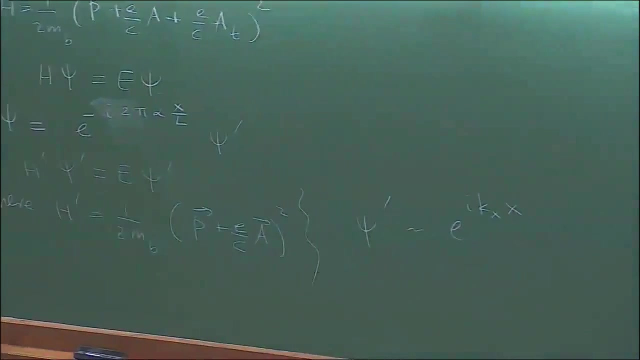 H prime is our familiar Hamiltonian that we know how to solve. Okay, So we know the solutions of this. In particular, we know that psi primed has a form like this. So remember what we did last time: We applied periodic boundary conditions. So we'll do. 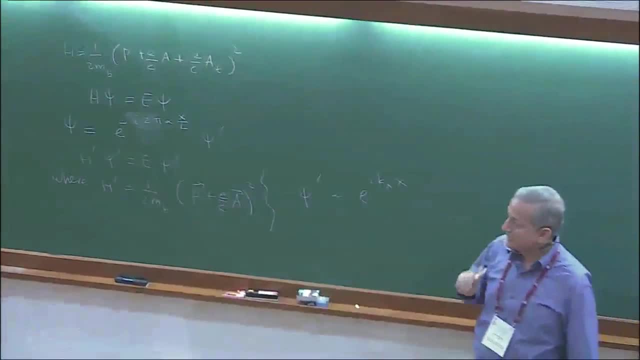 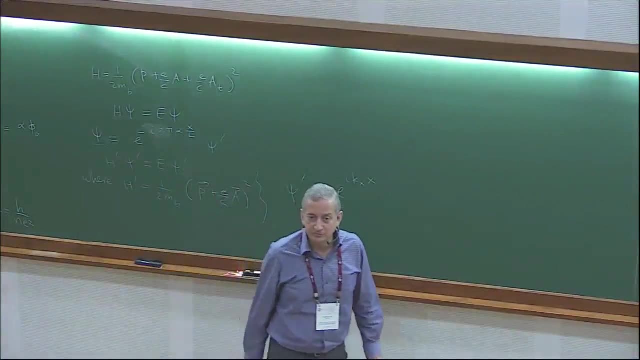 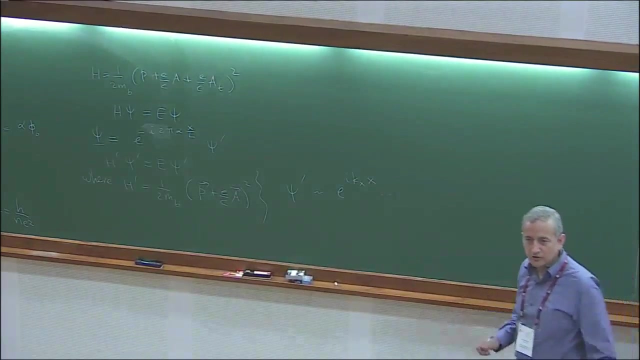 the same, But we have to remember that the periodic boundary condition acts on the physical, electron physical problem, which is psi. The physical wave function is psi, not psi primed. Psi primed is something that we encounter on the way to the solution. There is no I. 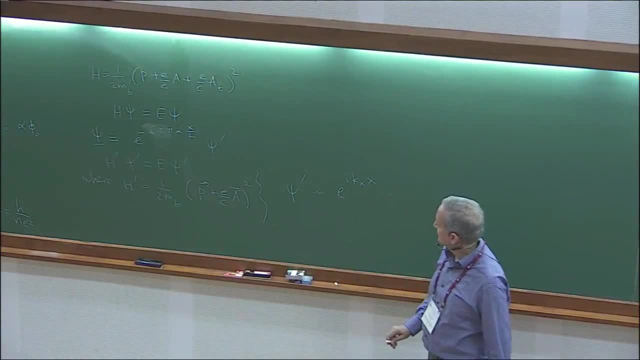 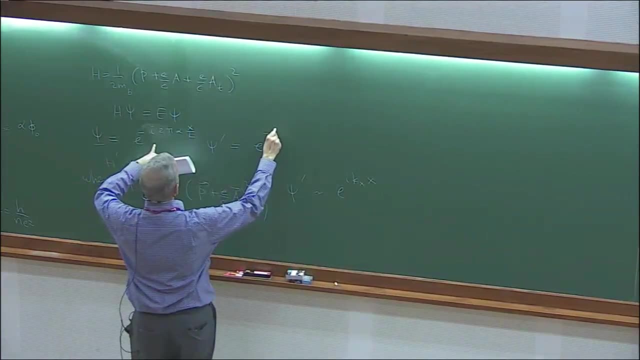 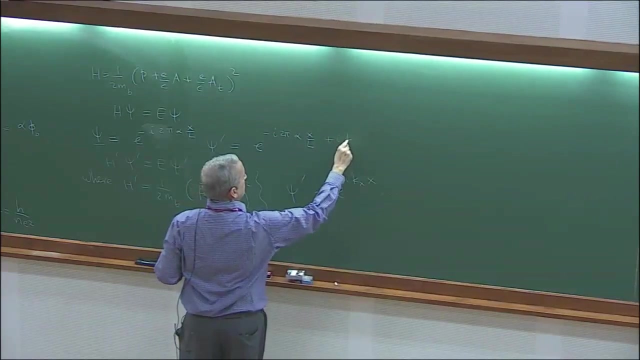 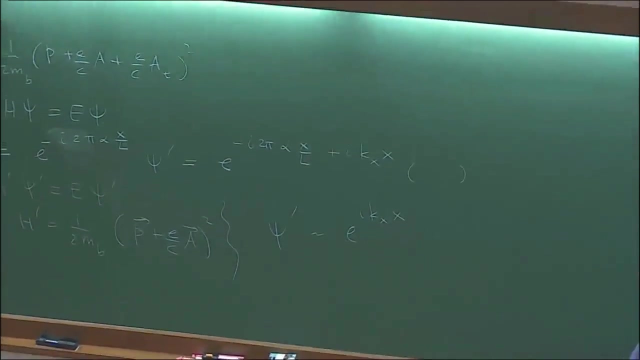 mean there is no physical meaning to be attached to psi primed. So if I go here I find that the solution goes like e to the power minus i, 2 pi, alpha x over l plus i, kx, x times something else. So there is also a component of the wave function. 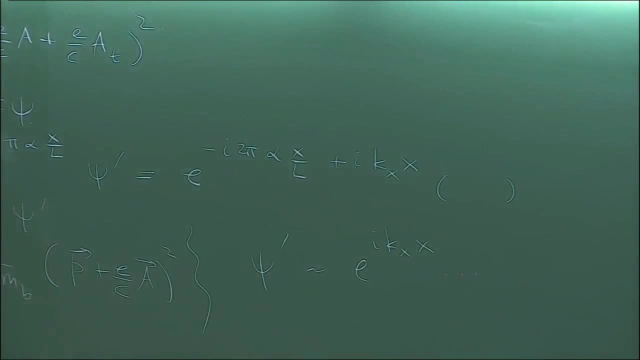 which depends on the y component. Okay, But that's not relevant to us for the present problem. So therefore I say I want to apply periodic boundary conditions. So that means that if I replace x by x plus l, the phase changes by an integral of multiple of 2 pi. So the 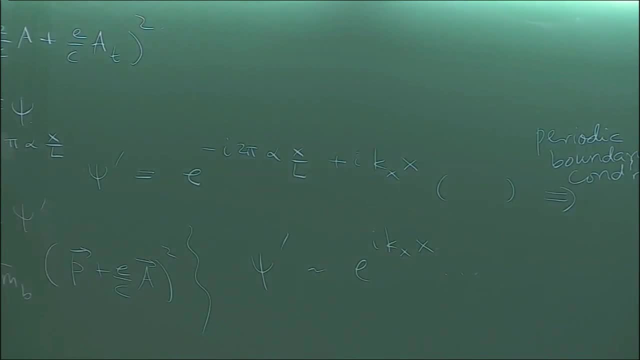 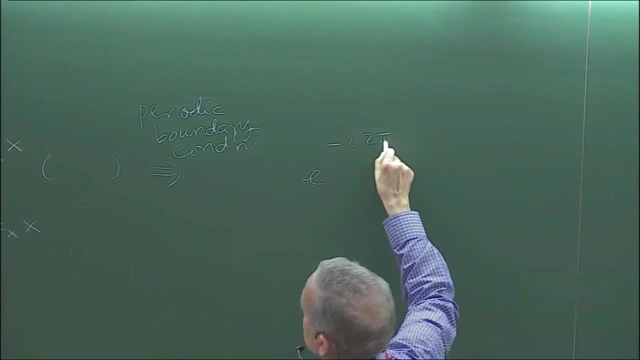 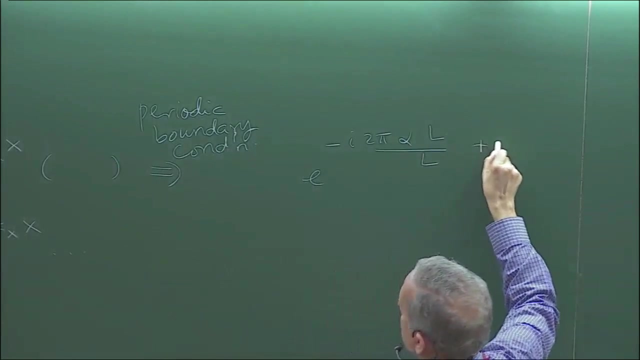 phase changes by an integral of multiple of 2 pi. So the phase changes by an integral of 2 pi. So the phase changes by an integral of multiple of 2 pi. So that means e to the power minus i, 2 pi. alpha l divided by l plus ikx l. 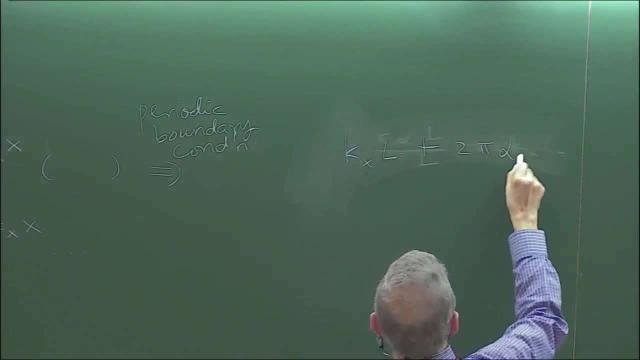 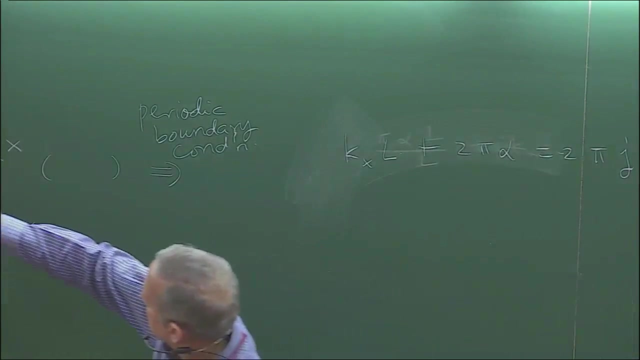 So periodic boundary condition means this thing where j is an integer. Okay, so this just means that if I replace, if I say that this quantity is equal to the same quantity, with x replaced by x plus l, then it would give me this equation. 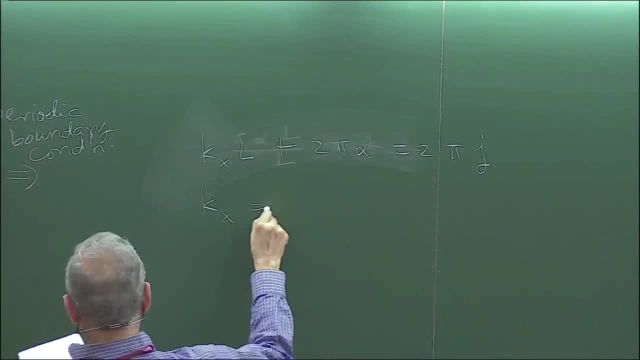 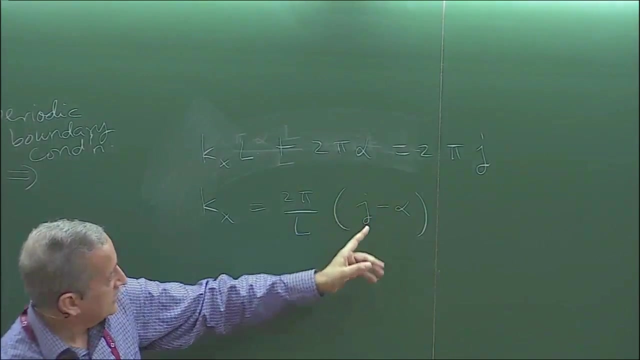 And this equation means that kx Is 2 pi over l j minus alpha. Okay, so now you can see the statement that I made. So as I change alpha from 0 to 1, this integer j changes by one area. 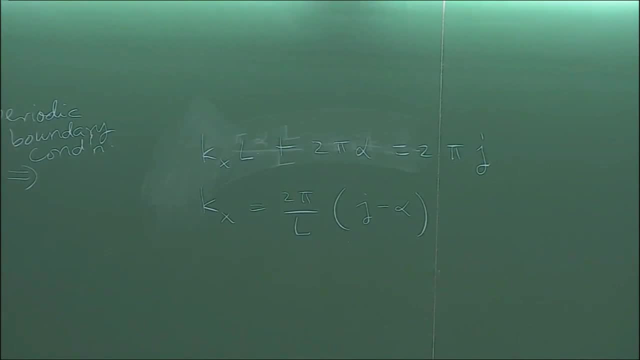 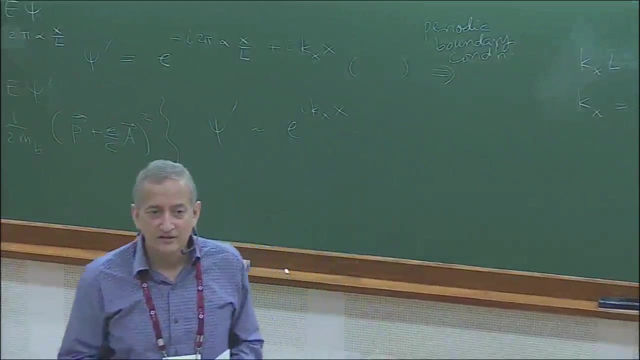 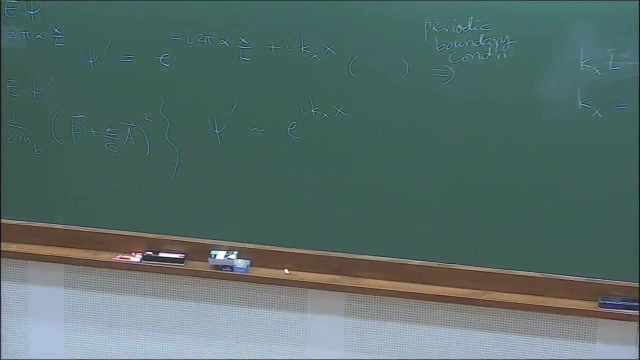 So my kx goes to the next kx. Okay, Okay, Okay. So this is the proof of this statement. Now, of course, we are not done yet. I mean, the actual argument is coming now. So right now we have only derived the result that if the filling factor is an integer, 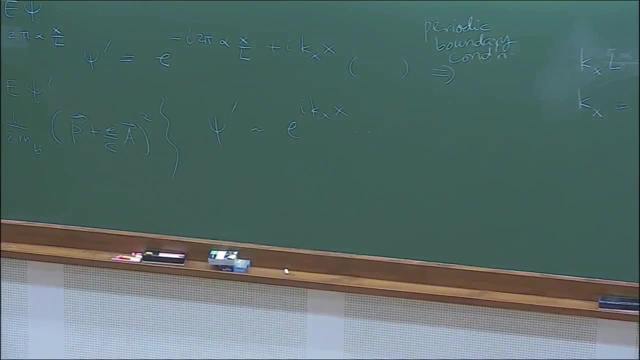 we get this result, But we have to show that this result is true even when the filling factor is an integer. So we can see that the filling factor is not an integer as we go slightly away from the integer filling. So there, the idea of Laughlin's was the following: 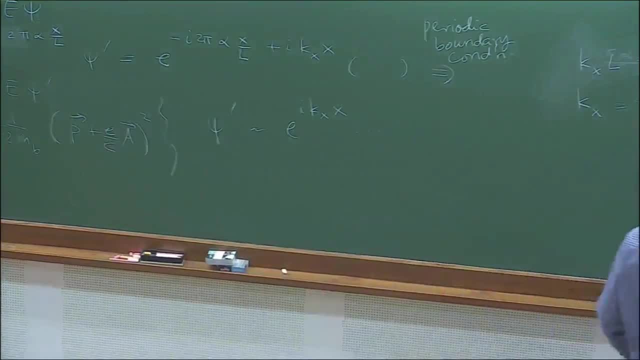 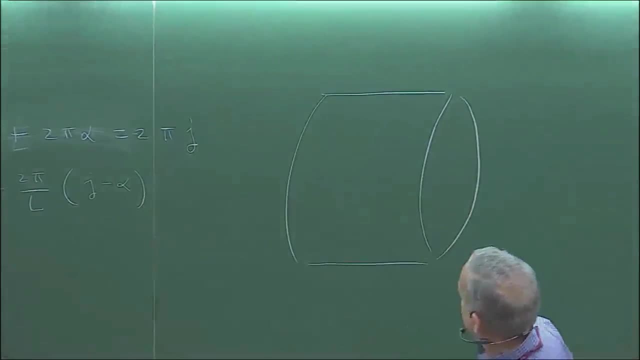 Let me now put some disorder in the system. So let's again. okay, so that's my cylinder And I'm going to assume that I don't put any disorder in the system. So that's my cylinder And I'm going to assume that I don't put any disorder in the system. 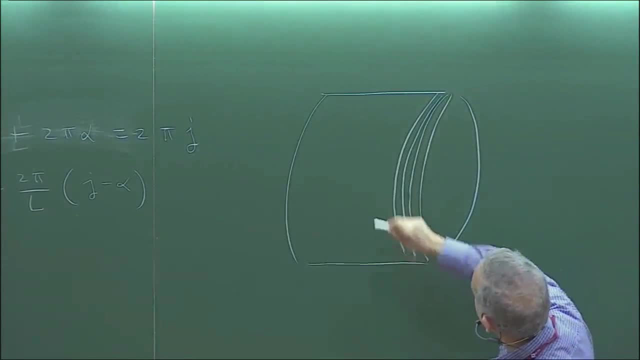 So let's say that I don't have any disorder close to the boundaries. Okay, So this is like trying to prove a concept. So we don't put any disorder close to the boundaries, We put disorder here. We saw earlier today that the disorder localizes substates. 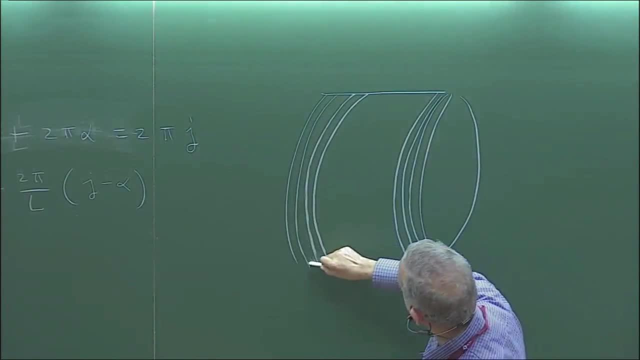 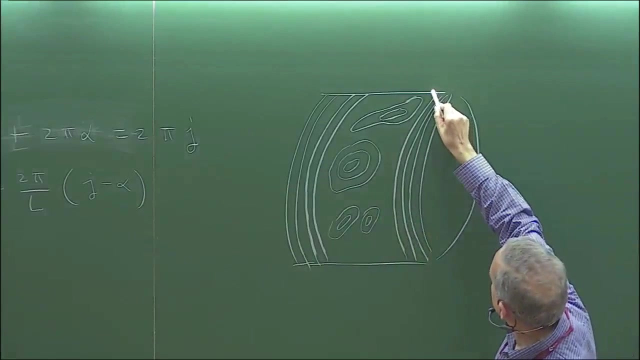 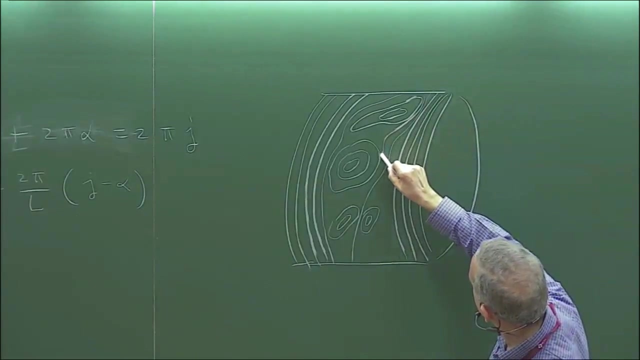 So let's assume that they put up a disorder here, And of course I will also have some, some of these other. so I will have two types of states, The states that go around the cylinder, like this one, this one or this one, and 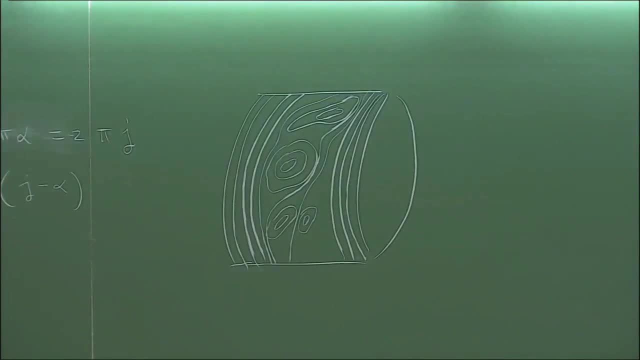 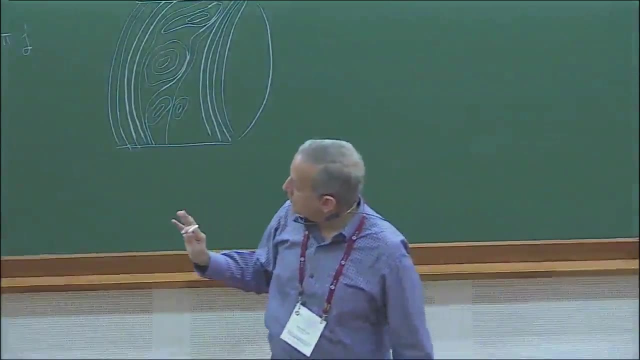 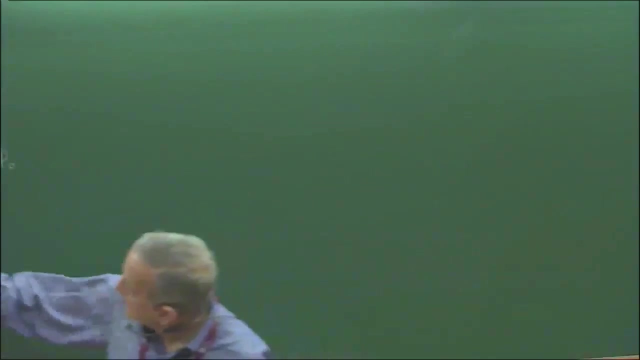 the states that do not go around the cylinder, that just are localized in one region. So when we insert this flux, so let's say I change this flux slowly, nothing happens to these states because I am not changing the boundary conditions for these states at all. These 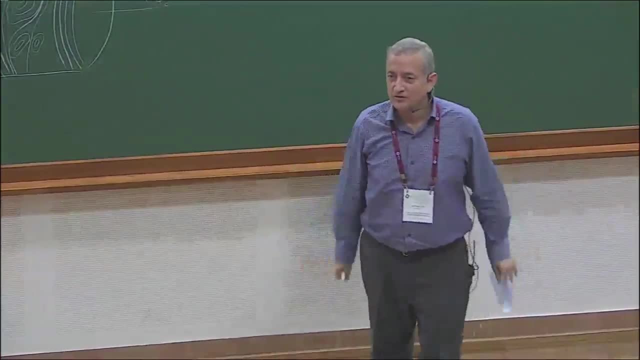 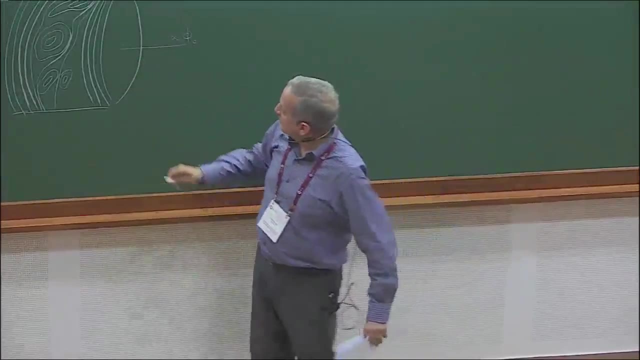 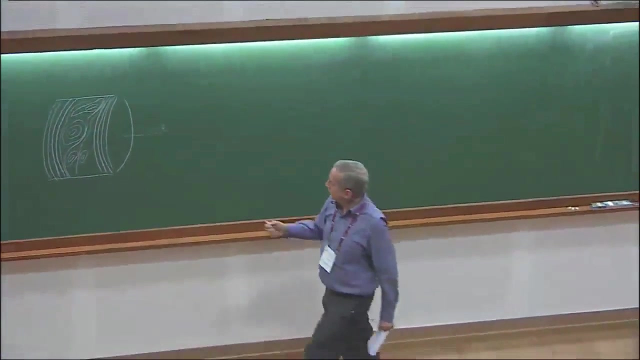 states remain exactly the way. they are completely unaware of the fact that there is this other flux. I mean, they are not sensitive to the boundary conditions. On the other hand, these states which go around the flux, they are sensitive to the boundary conditions. So this one will. 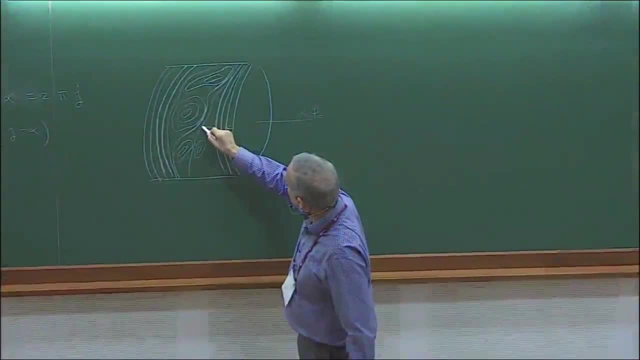 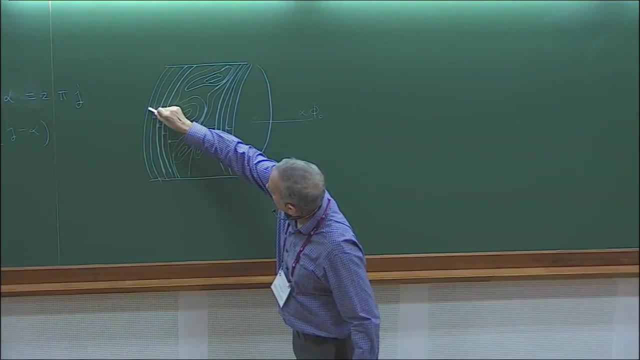 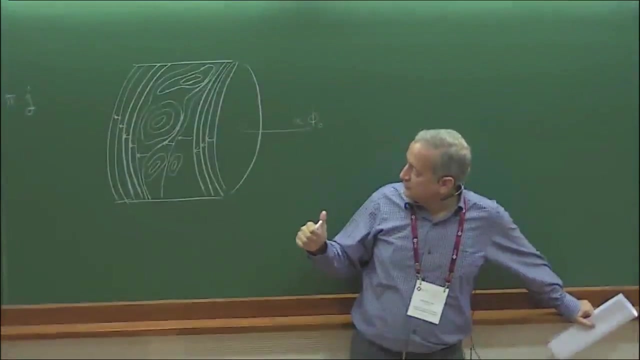 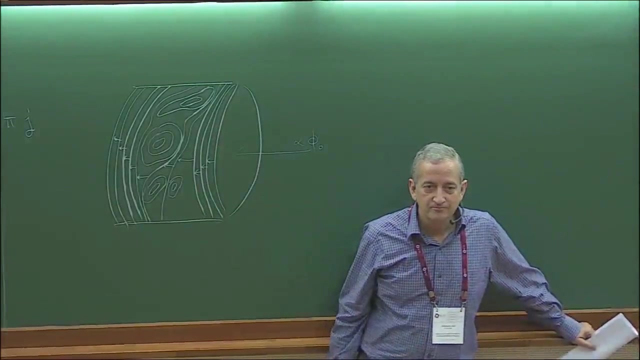 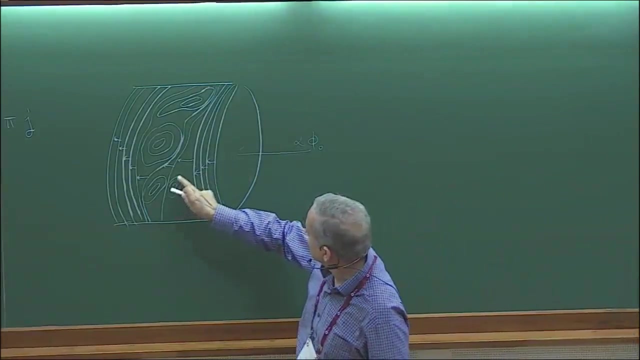 go here, this one will go here, this one will go here, this here, this here. Now let's assume that all of these states that go around the cylinder, they are all occupied. If they are all occupied- so I am assuming that these guys are all occupied- I don't say anything. 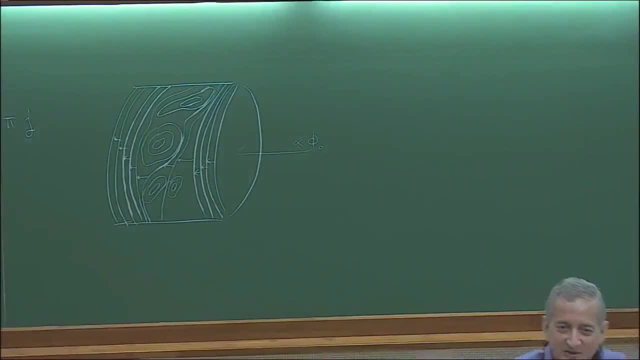 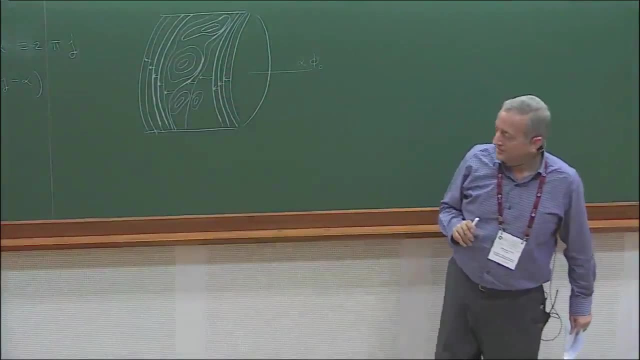 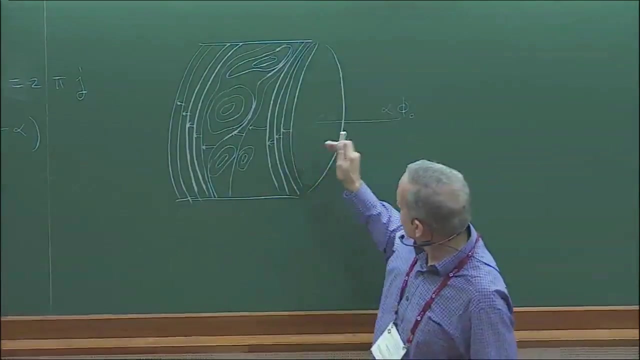 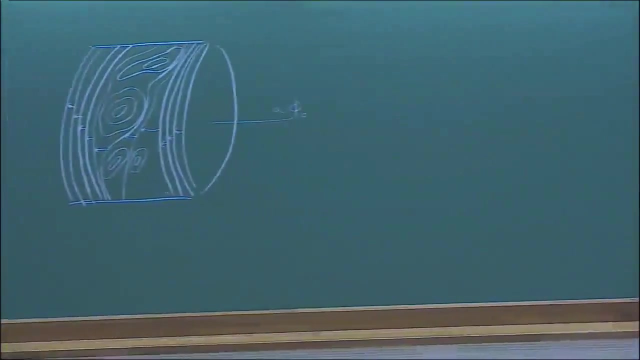 about these localized states. I don't care whether they are occupied or not. I assume that all of these states which go around are occupied. Then again, I get the result that when I change the flux by one unit, the energy is changed precisely by an amount that can. 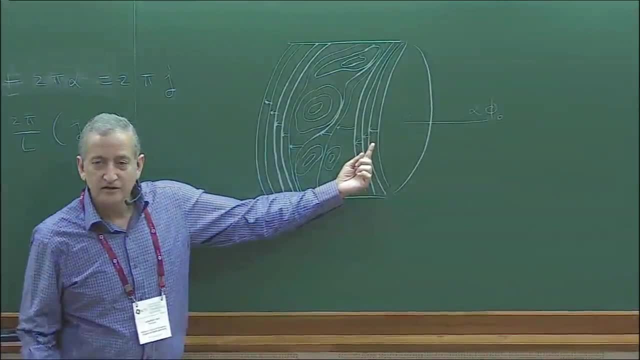 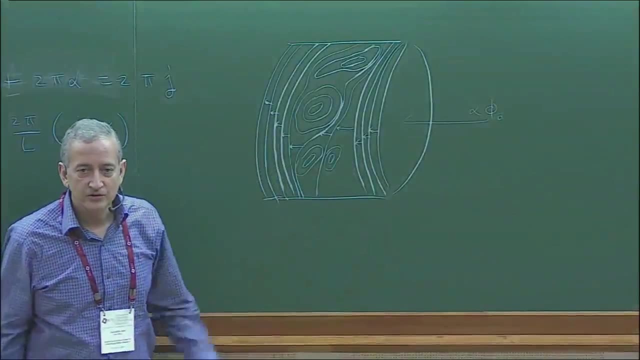 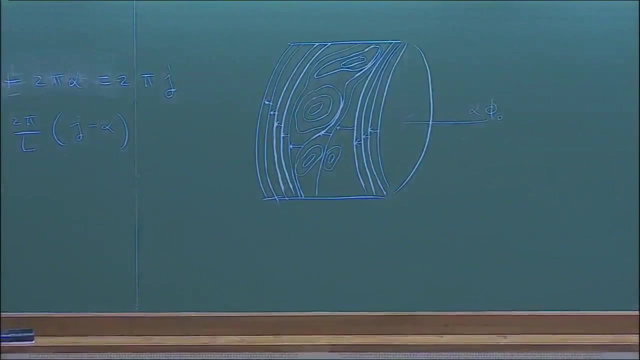 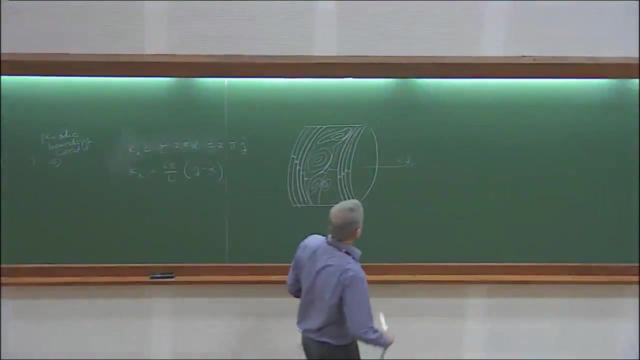 be calculated by noticing that n electrons go from here to here, where n is the number of Landau levels. So this happens for each Landau level And therefore we get the same result. We get exactly the same result. We get exactly the same result so long as all of these extended states are occupied. 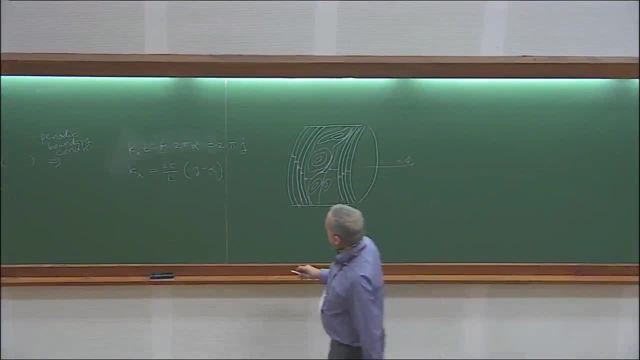 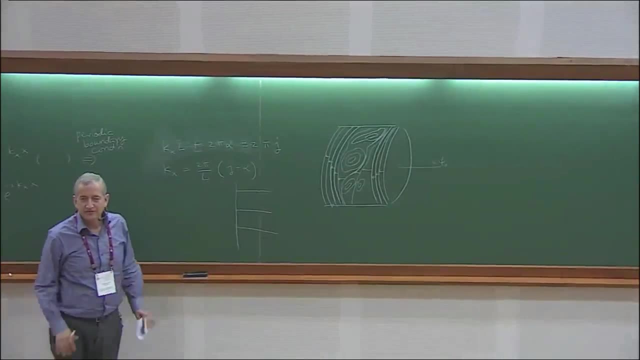 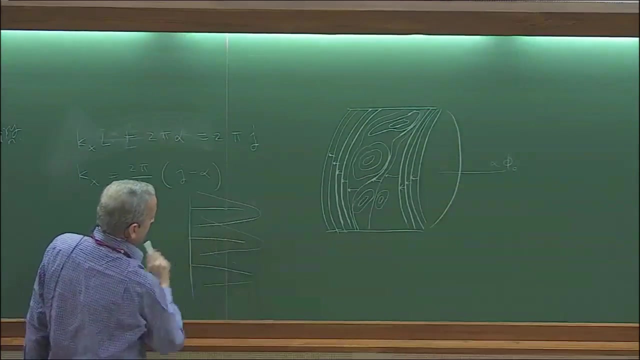 So the picture that appears is as follows. So this is something I had drawn in the morning. These are our piston Landau levels in the absence of disorder. When we have disorder, the Landau levels broaden, But there is, there are extended. 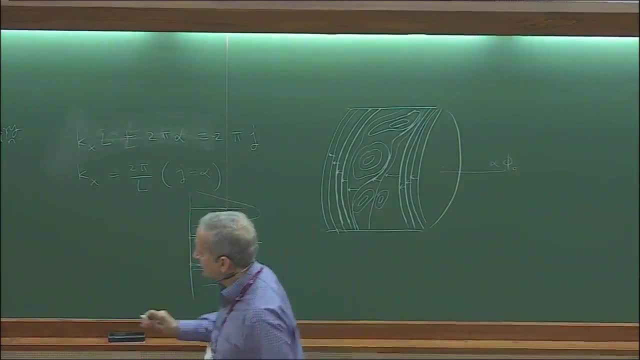 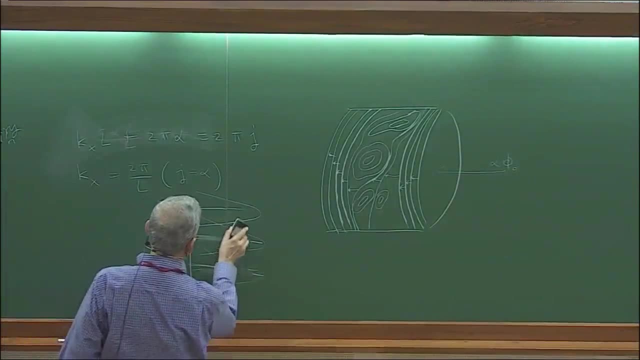 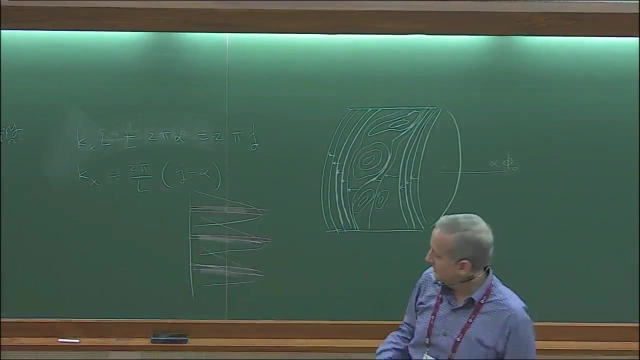 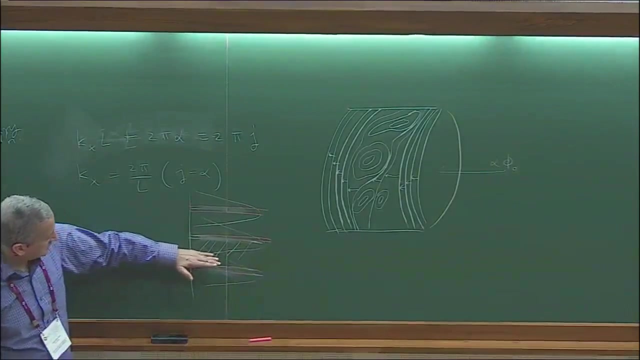 states here, So I can even use colored chalks. So I am for simplicity. I am showing a band of extended states And then I have localized states here. So so long as the Fermi level lies in the region that is localized, I get quantized all resistances. 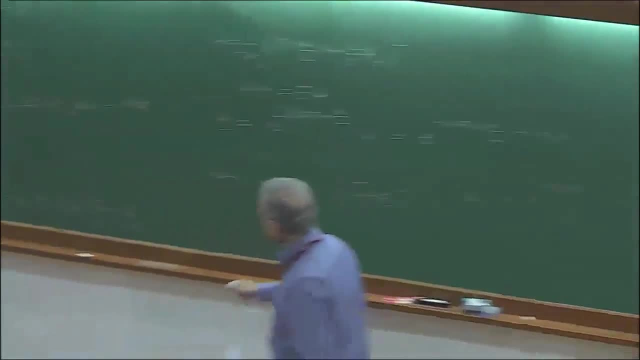 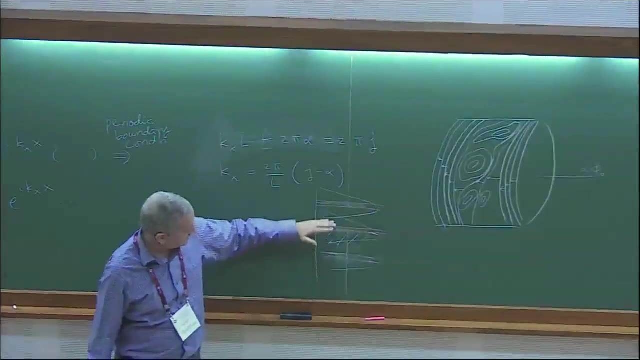 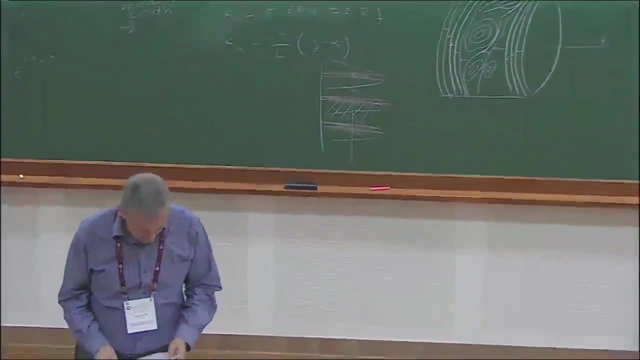 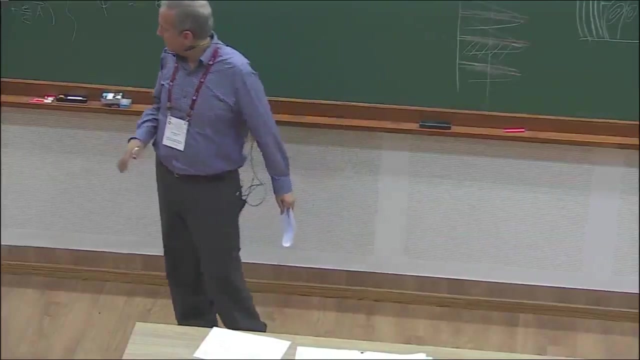 I get a plateau. The value of that is precisely given by this, where n now counts the number of extended bands below the Fermi energy. So that's Laughlin's gauge argument. The the crucial things. there are two crucial things in this argument. First of all, we 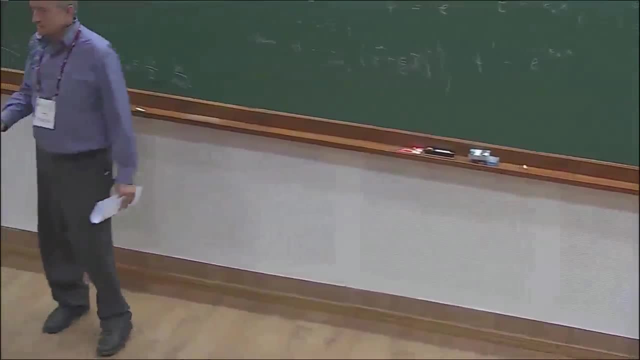 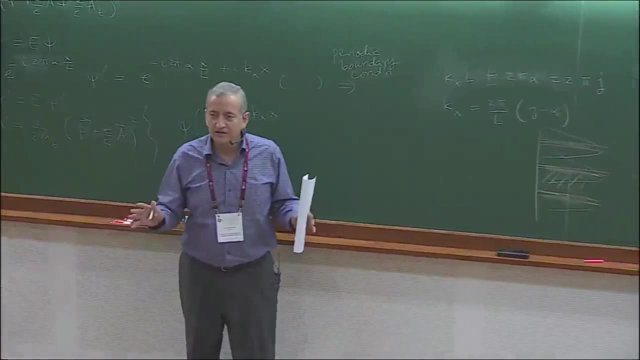 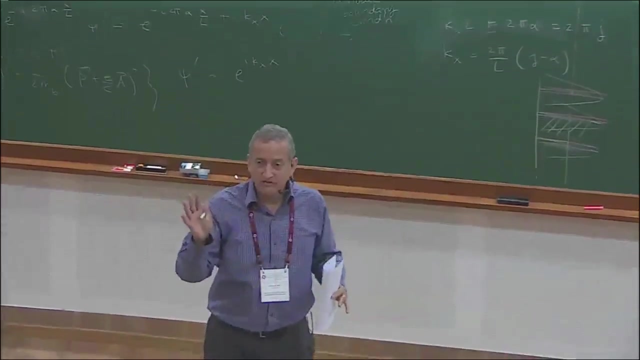 have to start with a system which in in technical terms it's incompressible at integer filling factors, which means that when the filling factor is an integer, I have gap to excitations. I fill n Landau levels completely And it costs some energy to excite a particle to. 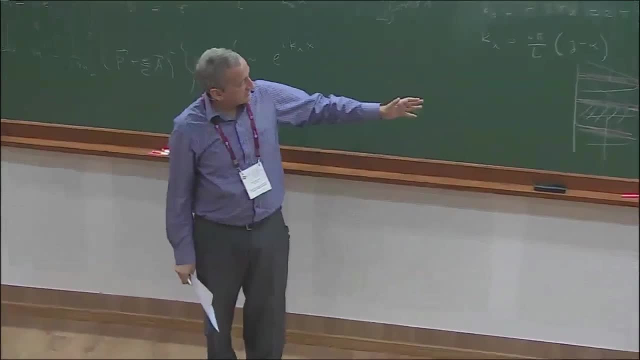 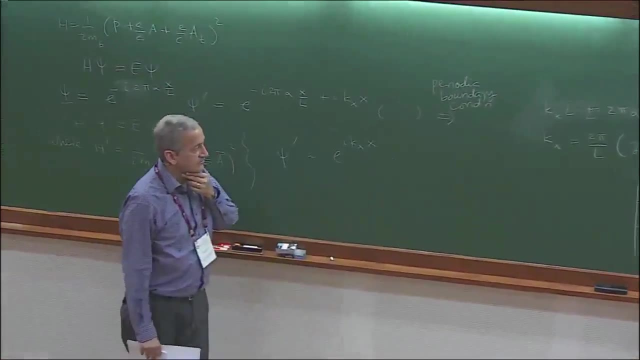 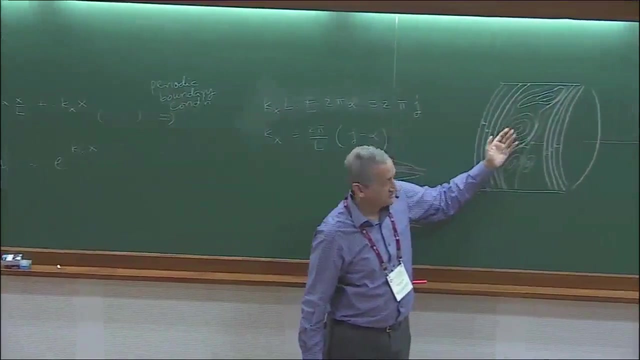 the Landau level. So that's number one, And the second thing that we need is disorder, which localizes some states And it acts as a reservoir, uh, which does not affect transport at all. As I empty these uh localized states. 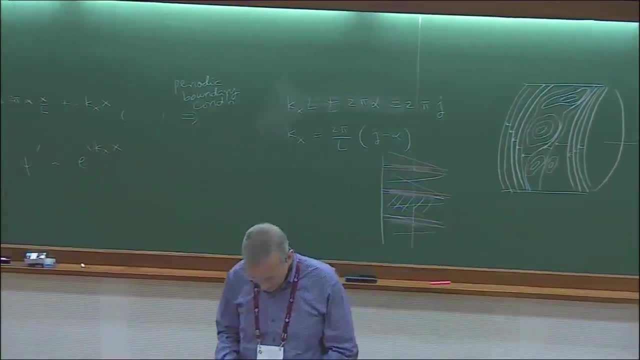 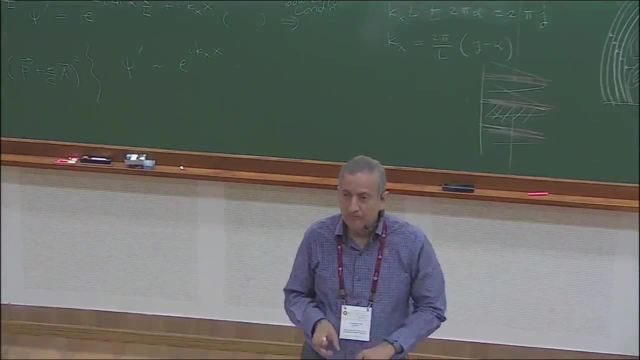 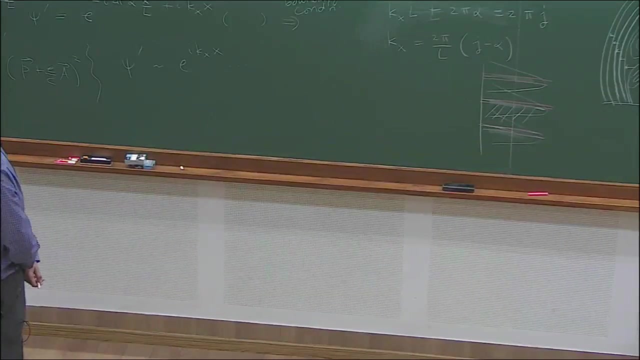 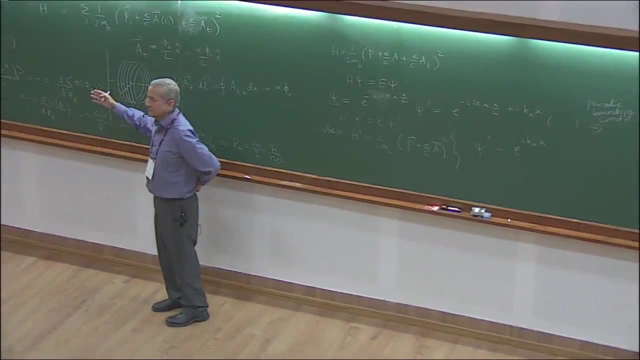 it does not change any of the transport conditions. So any questions on this? this part, Okay. No, n is the number of Landau levels. So this is a picture for one Landau level. Okay, But there is a similar picture for the second Landau level and a similar picture for third. 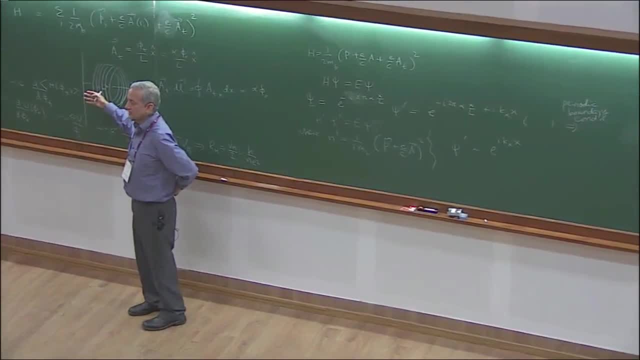 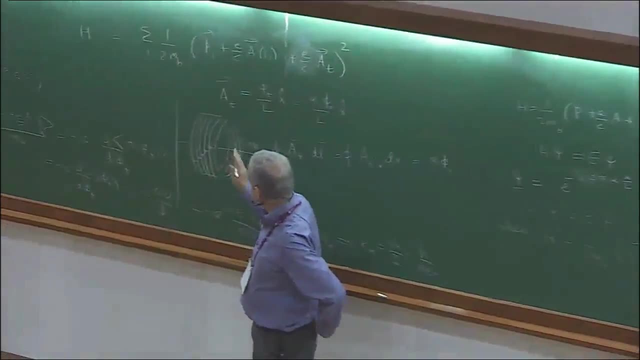 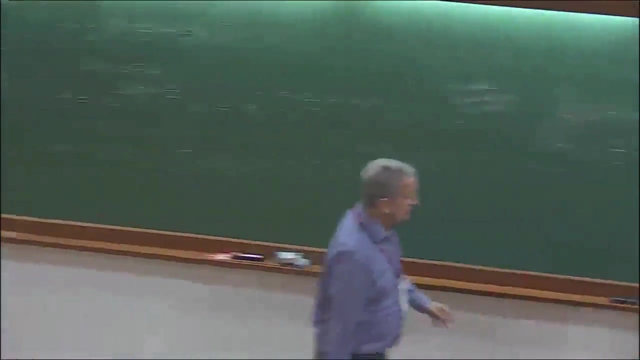 Landau level and so on. So these are all the Landau levels that are below the Fermi energy. Okay, So if if I consider only the lowest Landau level, then n is one. So it's uh. another way is: n is the number of these extended bands below the Fermi energy. So if I'm here, I 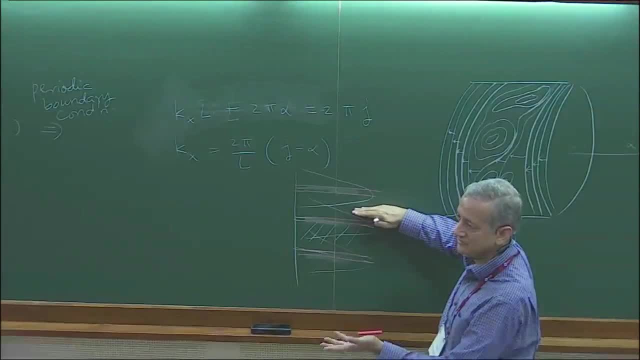 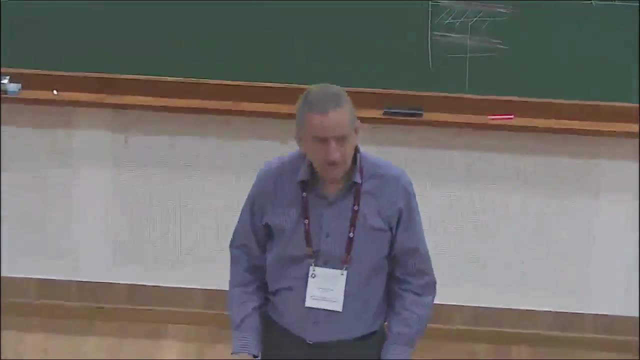 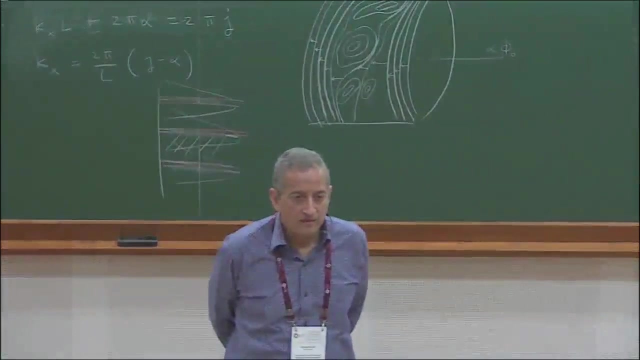 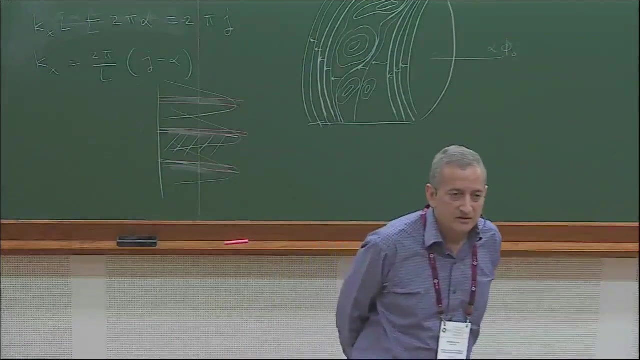 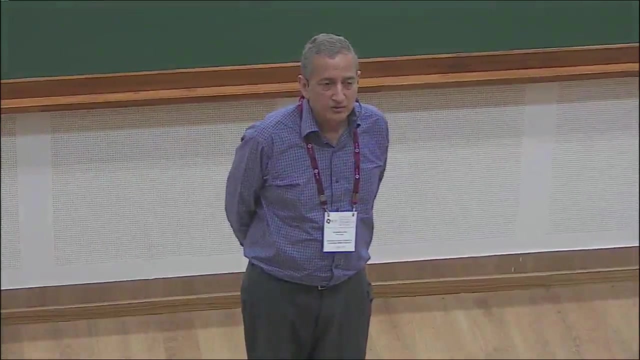 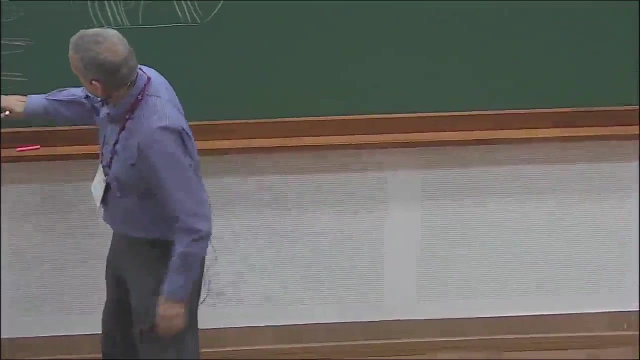 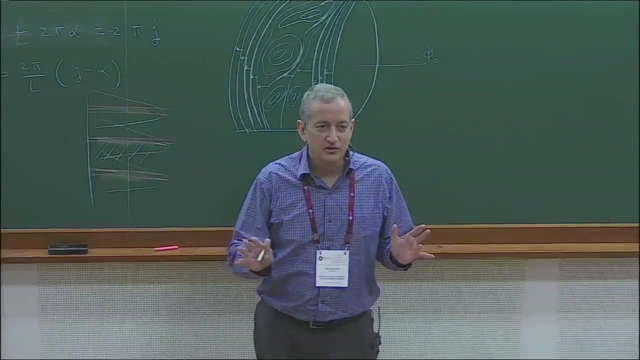 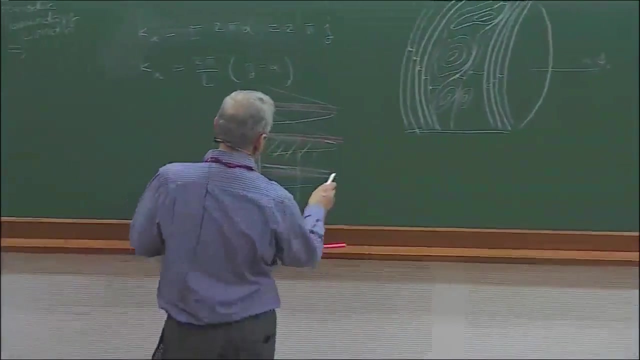 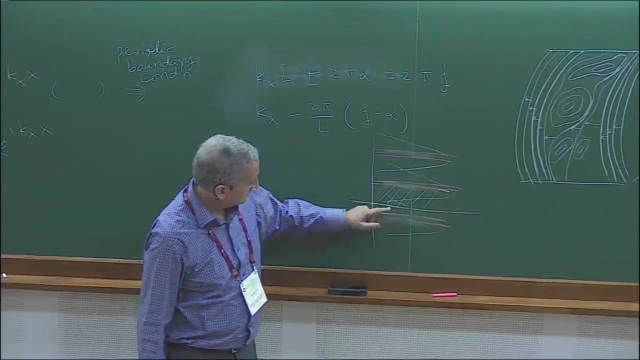 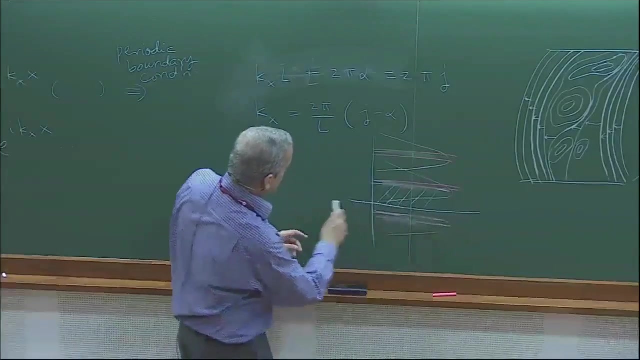 have two, two of these bands, which actually is the number of Landau levels below the Fermi energy. Yes, please, Let's warmer, Let me, let's cool that down, guys. 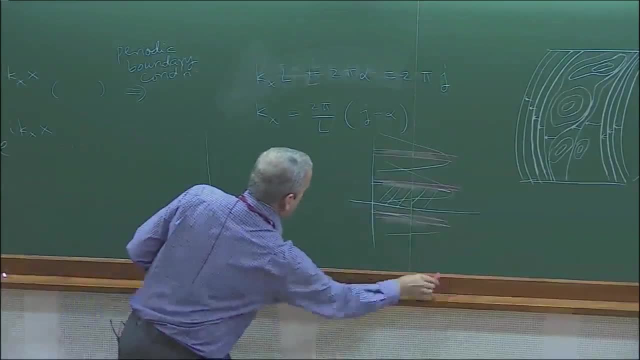 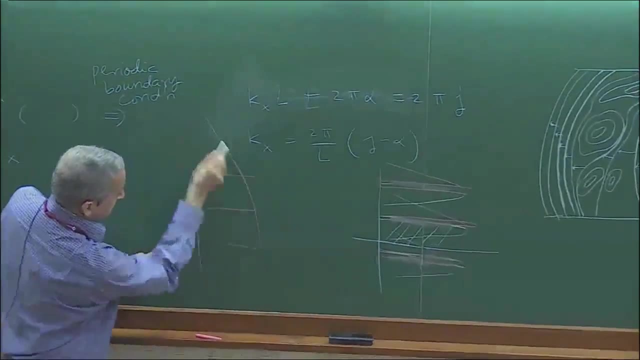 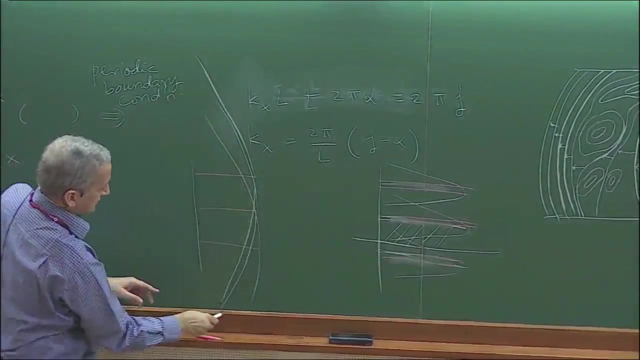 So this can become very broad and this lander level can also become very broad, and this becomes very broad and the Fermi energy will go somewhere here, because I have localized. 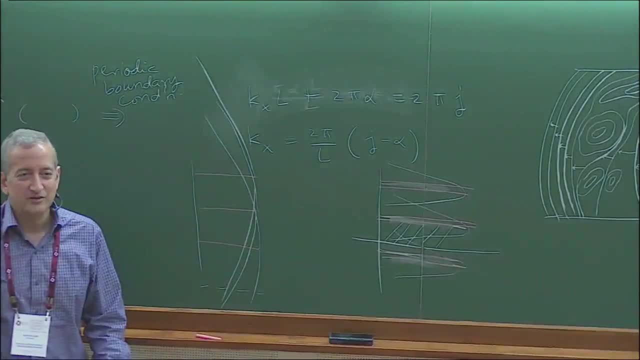 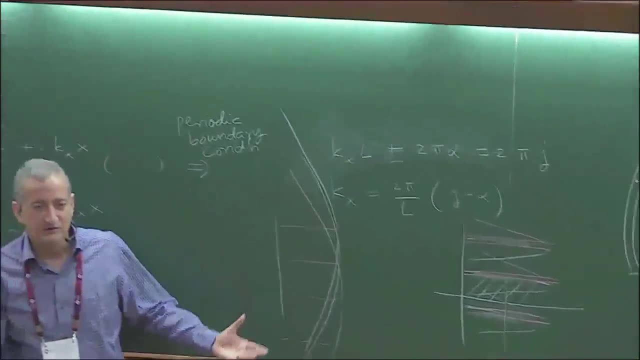 states from higher lander levels that electrons can fill at lower energies. So eventually I mean this, you can say it's. there is a name for this. it's called floating up of extended states, because relative to the Fermi energy, the extended states are. 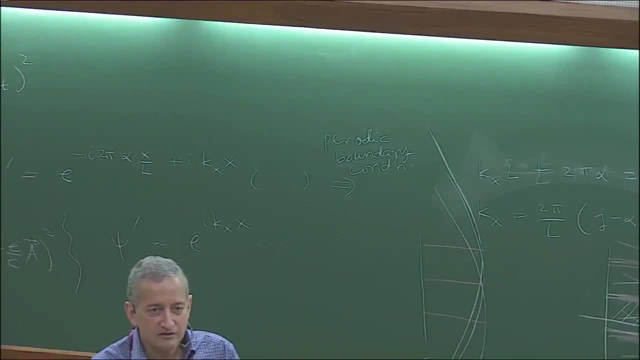 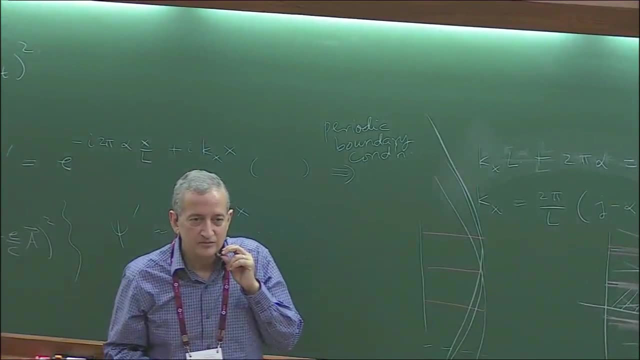 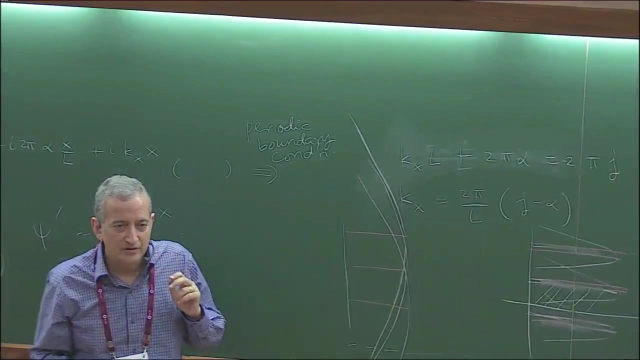 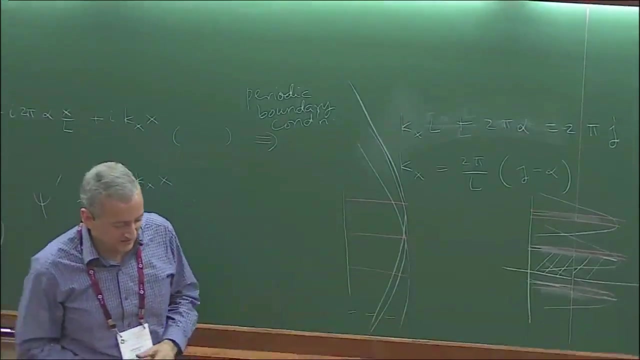 kind of rising up, but eventually you can get to an insulator which is just a regular insulator. Yeah, exactly, So there will be an energy where you have an extended state. So this is a statement in the… like it is true in the asymptotea. you have an infinitely large sample and you have random 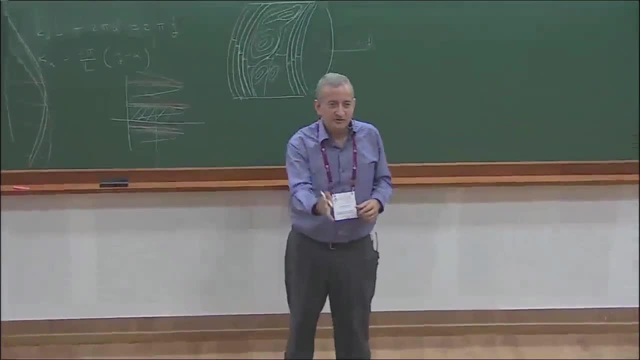 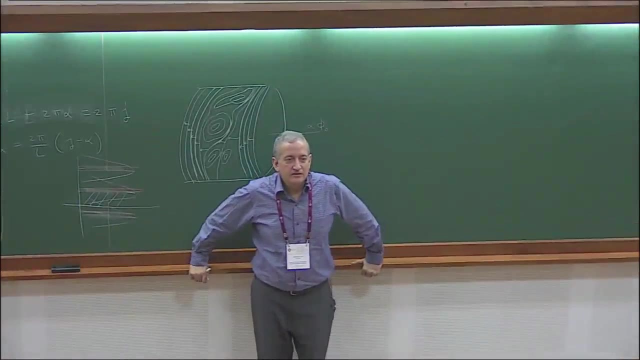 disorder. of course, if you have a finite sample and you break it into two, then you- I mean this, but it's believed to be true conceptually that for a sufficiently large system you cannot get rid of these extended states. get one energy Okay. 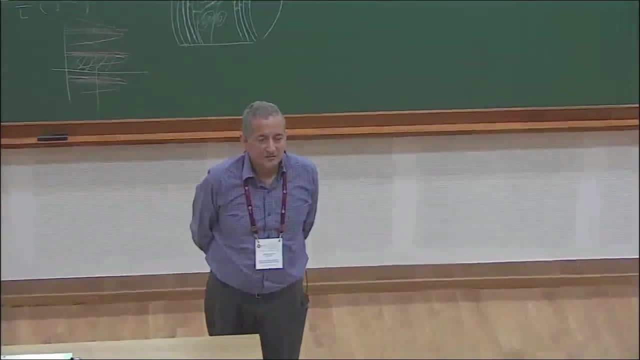 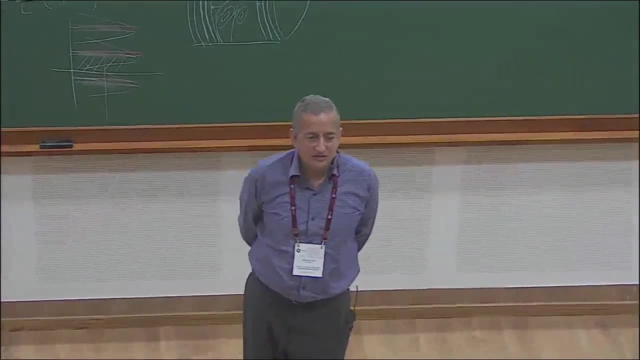 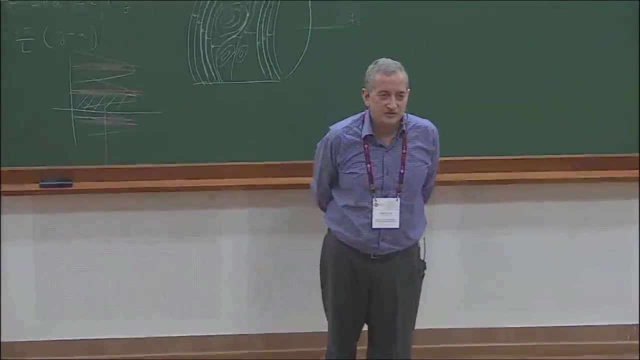 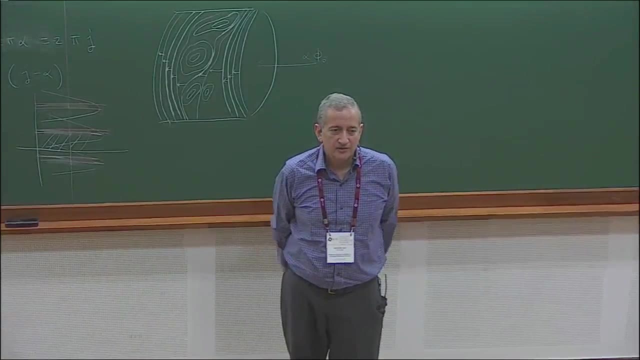 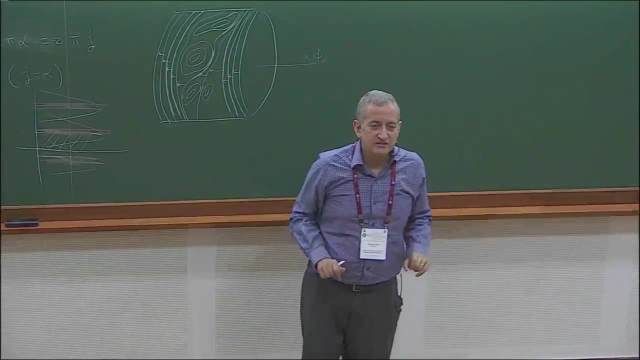 So there can be many extended states. It's not very easy to see, So in the kind of picture that I drew it, let's say I have both potential for that. it's easy to see because it's a percolation transition. So imagine you have two free states. it's going to be, it's going to go straight to one energy. but what ever it is, it's going to go directly to another energy. So it's going to go, so that it's going to go, so that it's going to go and so that it's. 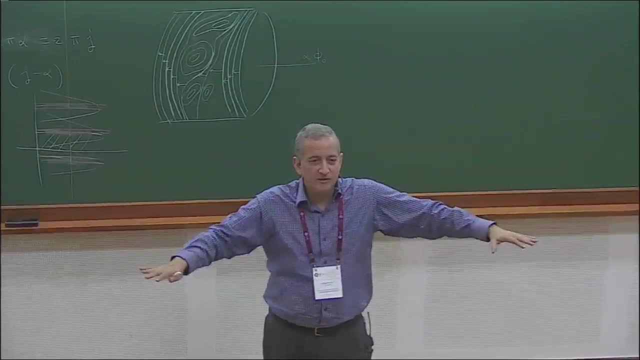 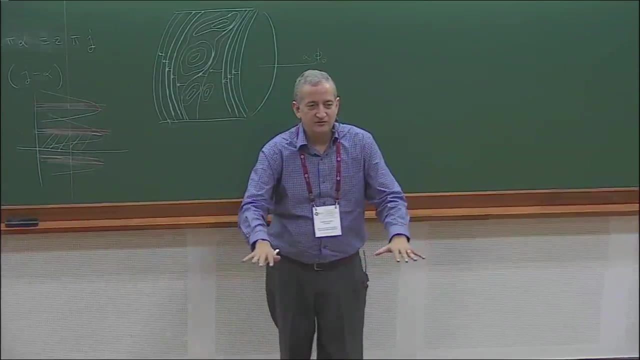 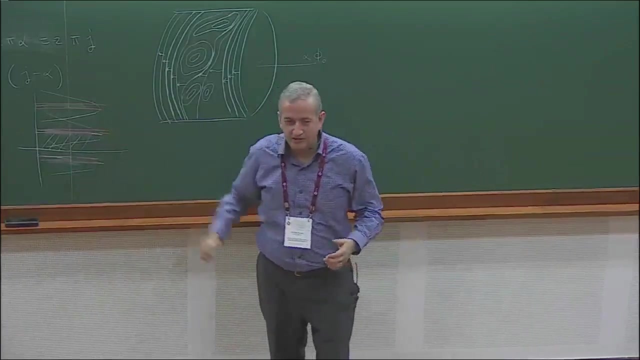 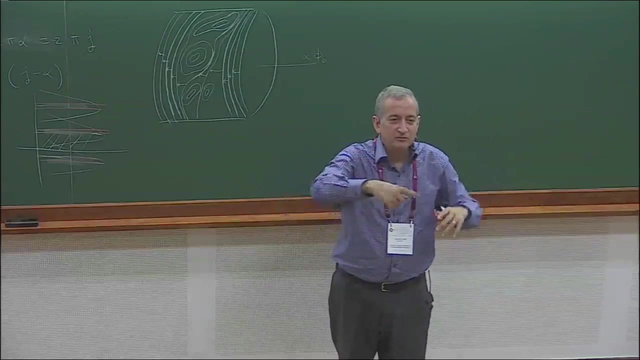 going to go together, like you know, hills and valleys and so on, and you start filling water. okay, so water tells you where the sample is filled and the region outside region not covered by water, is like these potential hills. now, up to some point the land percolates, but at some point the water percolates. 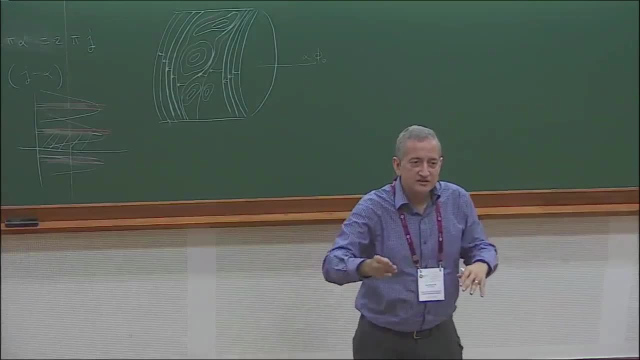 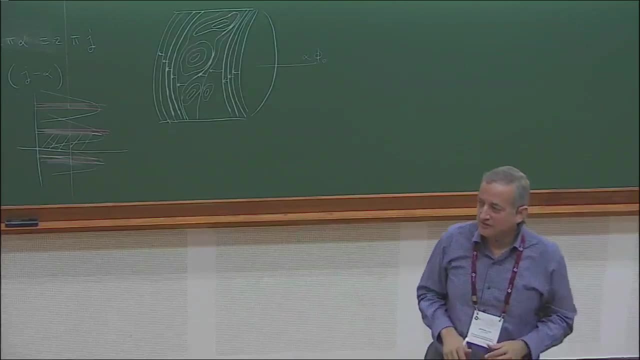 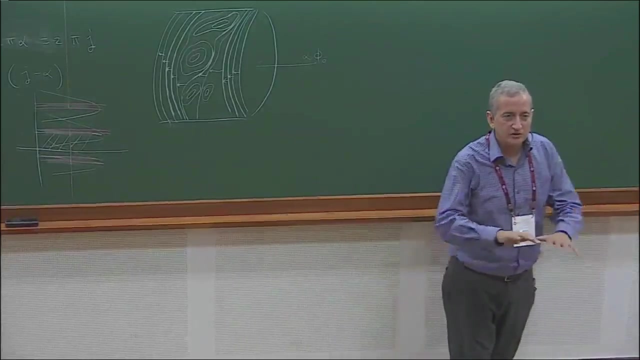 and at the transition there is an extended state, so the percolation length goes to infinity. so that's like classical percolation picture. that remains true even in quantum holopact, although the quantum mechanical nature changes the exponents and so on. but the overall picture remains true. 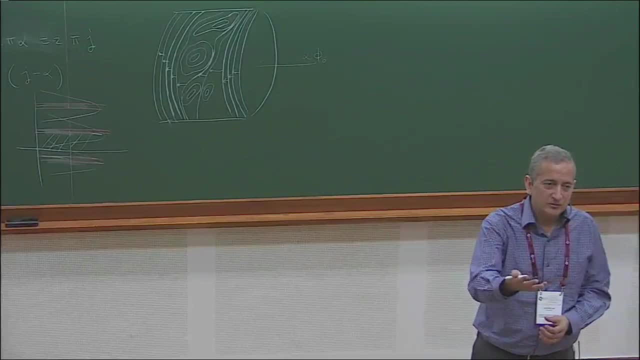 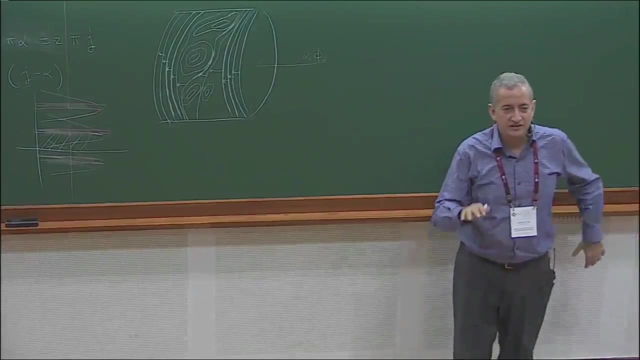 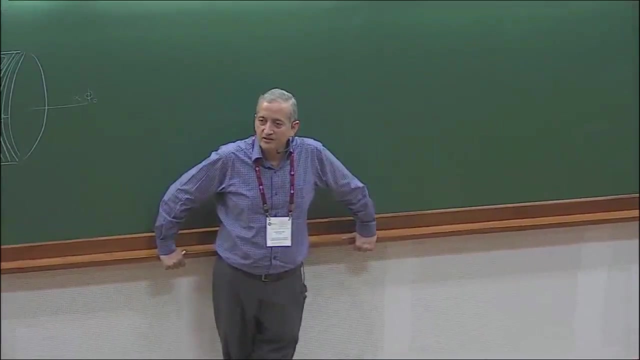 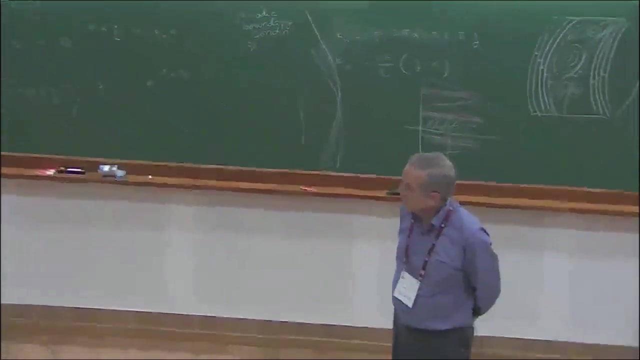 but you know that's a simple picture. but you could ask what happens if i take delta function disorder and at least numerical calculations say that again there's a, there is, there are extended states at a, at a single energy. Any other questions? Yes, please. 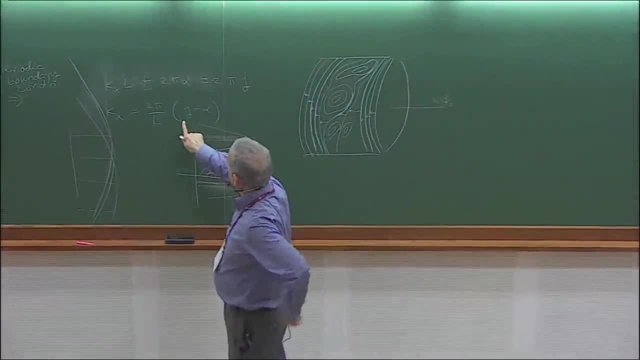 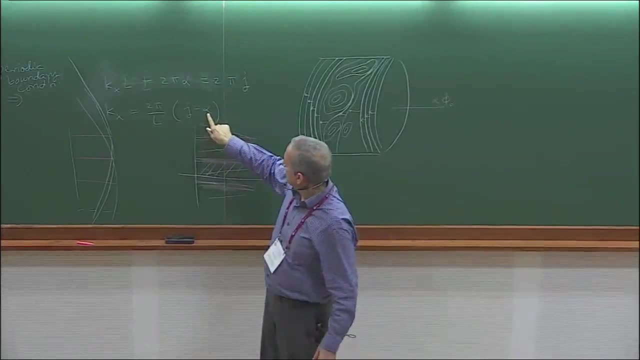 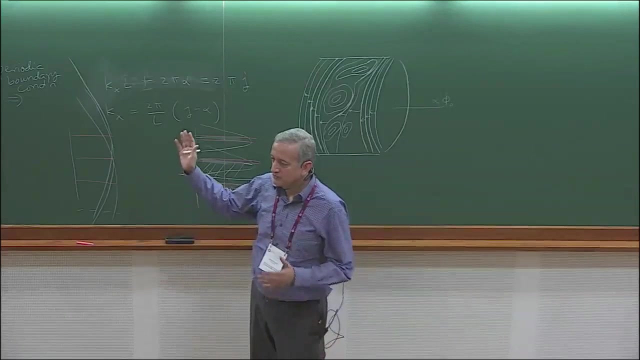 Well, that that follows from this. So as I change. so let's say I start with a state which has j equal to ten, then and alpha equals zero. as I change alpha from zero to one, this integer becomes nine. So the wave vector, and remember there is a connection. 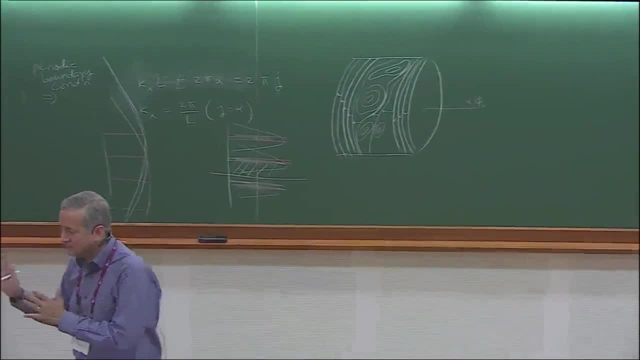 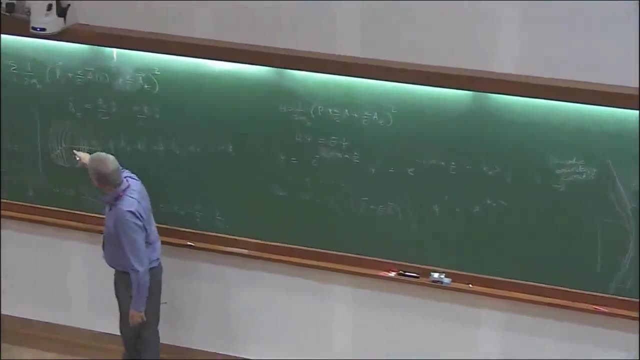 between the wave vector and the position of the state. Okay, so as the wave vector change, changes I mean. so by changing the boundary condition, you are actually changing the wave vector, and since wave vector is connected to the position, this thing is slowly moving. 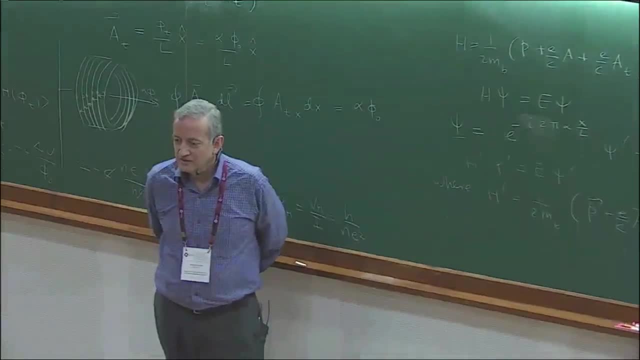 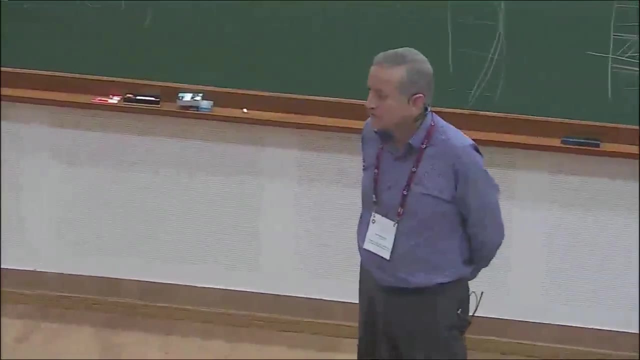 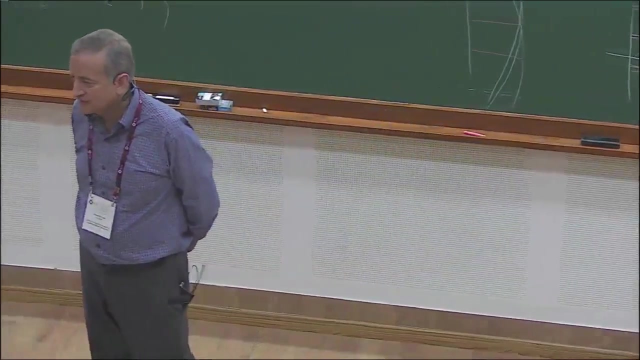 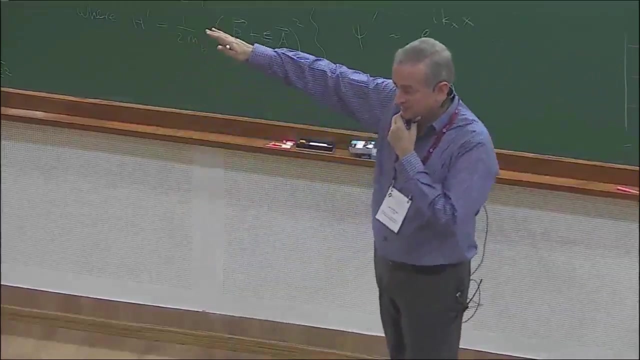 to one side. Yeah, so periodic boundary condition is a nice way to derive the result. I mean there are other ways to see this. So this is also connected to what is known as churn number. So there are other ways to see this. but I mean that's a generalization of Lafayette's. 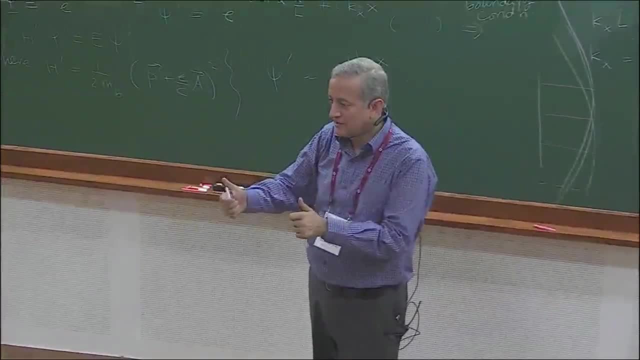 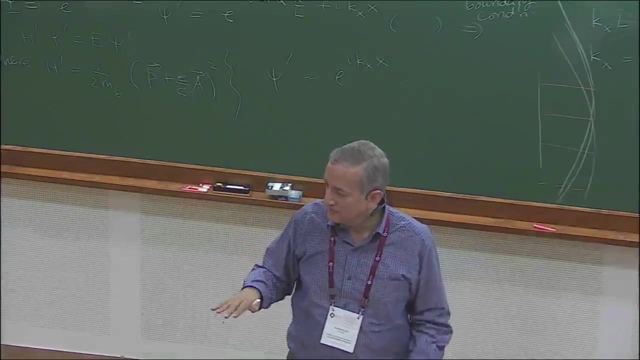 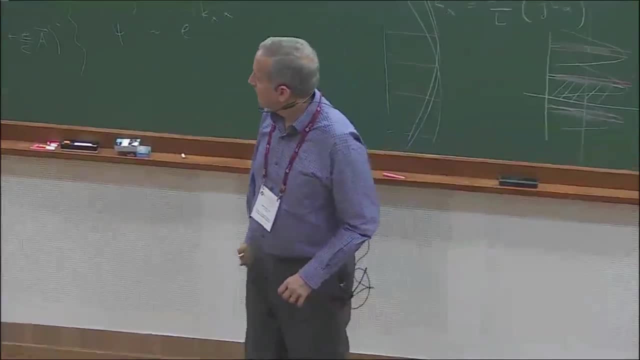 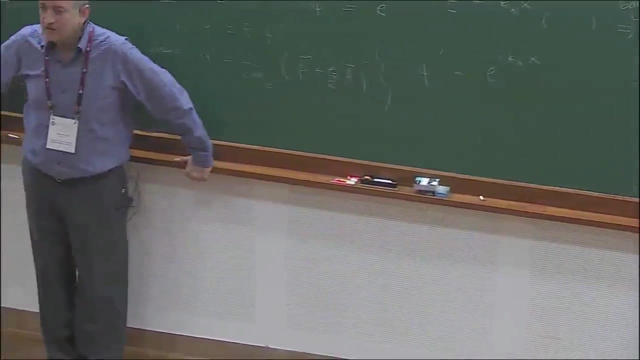 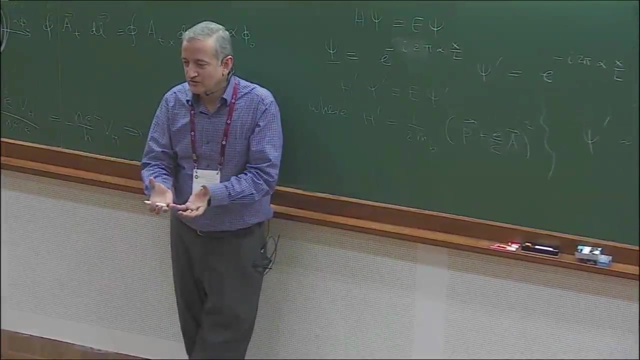 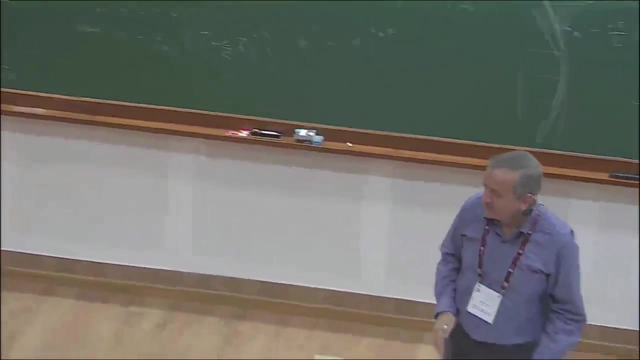 change it discontinuously. So so there are more rigorous arguments, which I mean even there you do make use of periodic boundary conditions because you have to have this log torus. So anyway, assuming that the results, that the real physics, real coefficients, 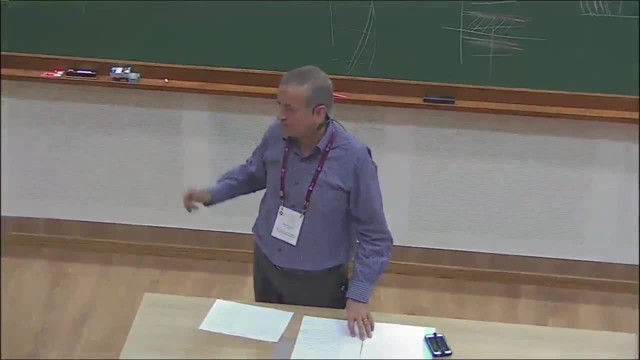 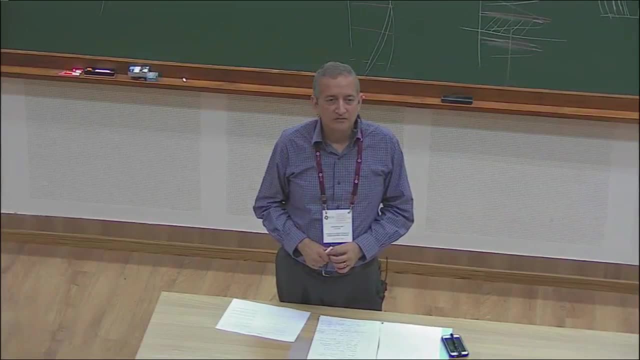 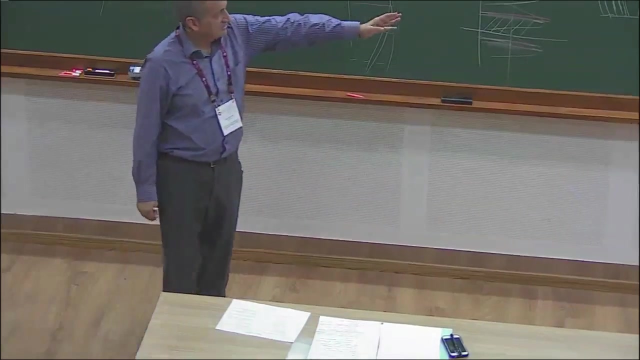 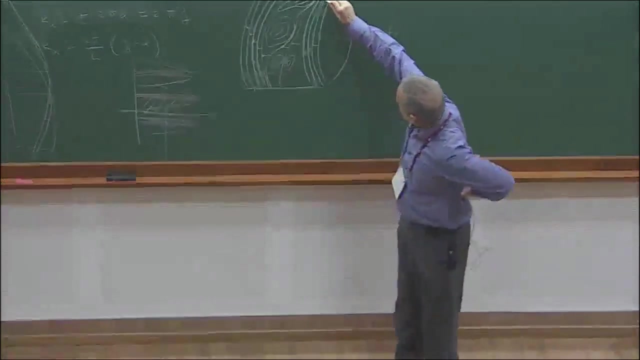 do not depend on the choice of boundary conditions. you know, this is one way to derive this. Yeah, Yeah, yeah. So, in going from here to here, I'm going to, I'm going to, I'm going to. I'm now talking about some more general situation. So what I have done here is that. 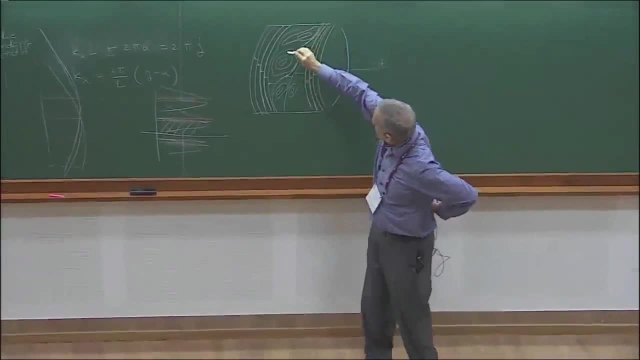 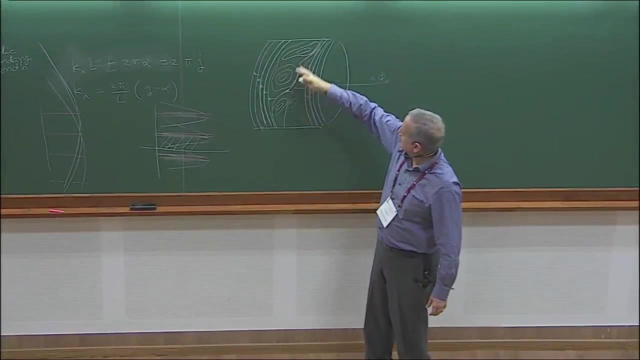 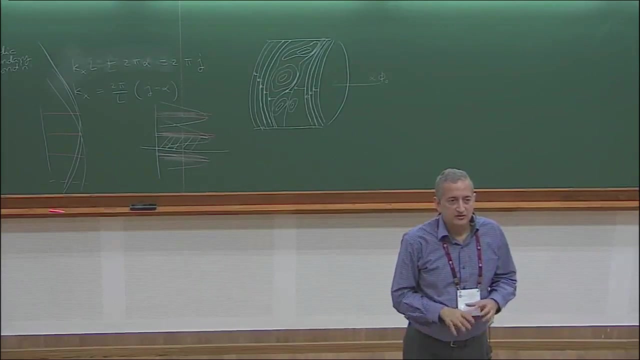 I have assumed that I have well-defined wave vector in this region and this region. okay, and then there is no wave wave vector defined for these states. These are going to be some very complicated states, which would depend on the actual disorder there. Well, there. 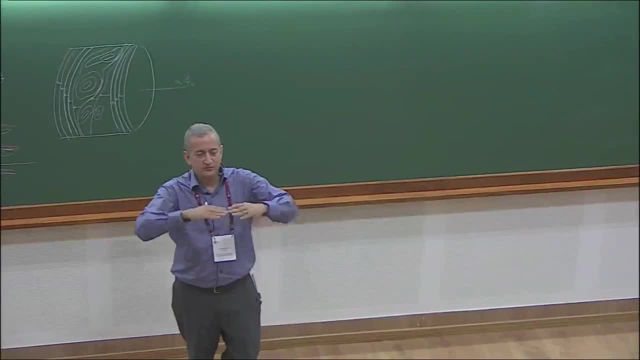 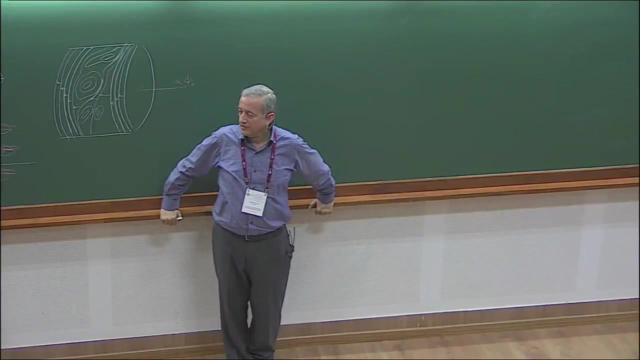 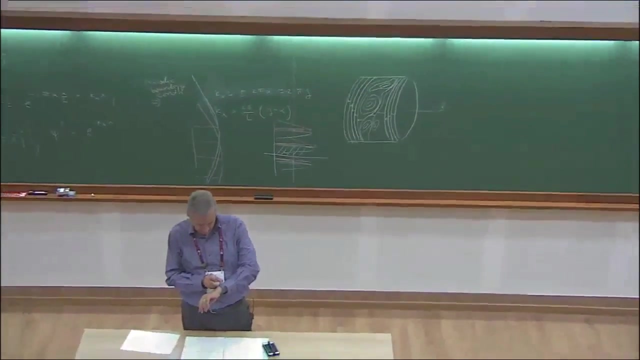 is a mobility edge, but it's just one. so typically a mobility edge means all states below are extended and all above are localized. but here it's a different problem because you have extended states only at some discrete energies. Okay, So let me, since we are here, 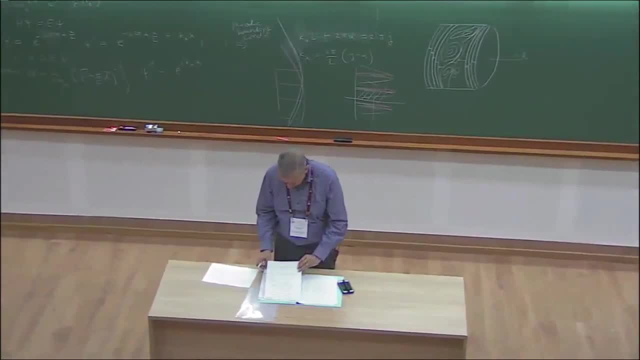 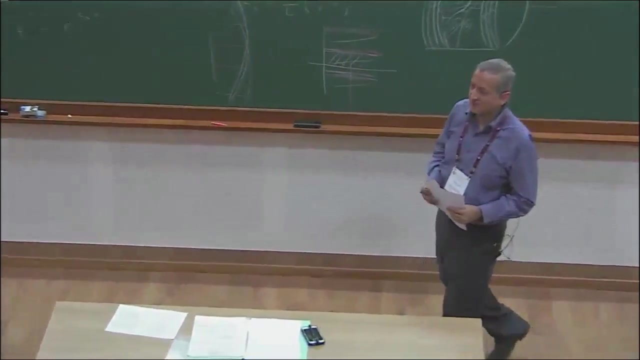 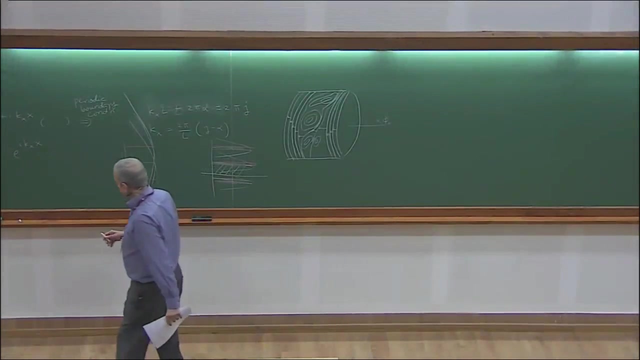 okay, Okay, Okay, Okay, Okay. So, since I have some time, let me go to fractional Hall effect and introduce Laughlin's wave function, because since we are talking about Laughlin's theory for integer Hall effect here, let's go to his work for fractional Hall effect. 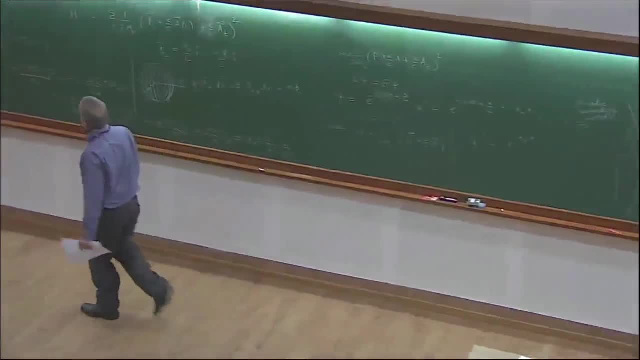 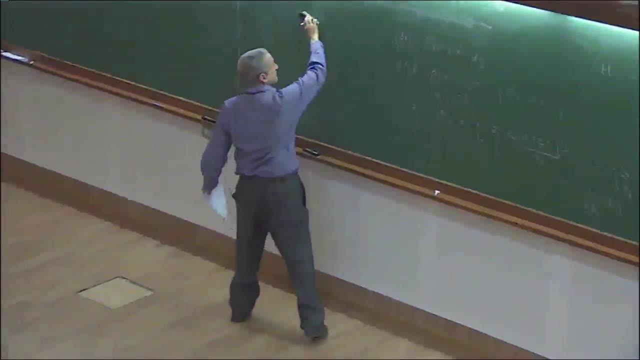 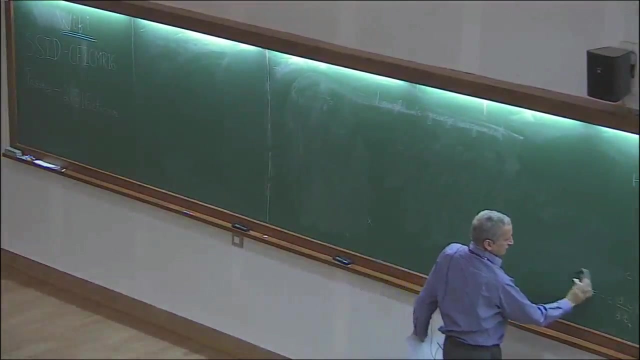 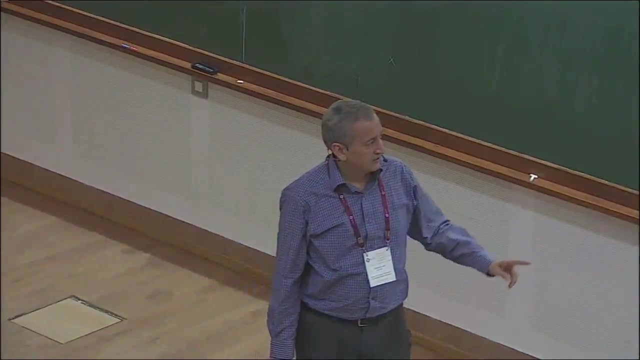 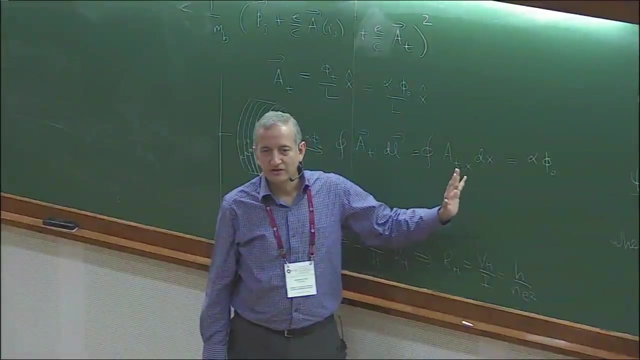 So Okay. So one thing you can see already is that if I assume electrons to be non-interacting, if I ignore the interaction between electrons, then I can only get h over an integer times e squared by this argument. You cannot get anything else. So the question is: how do? 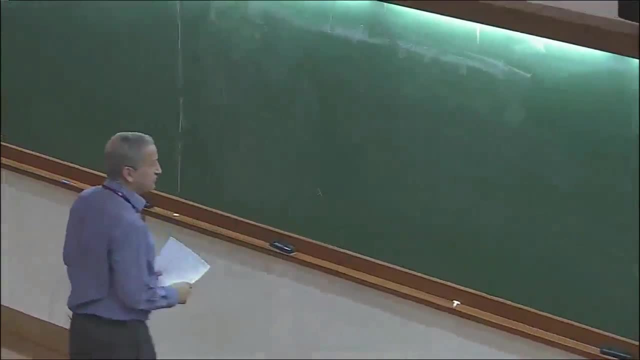 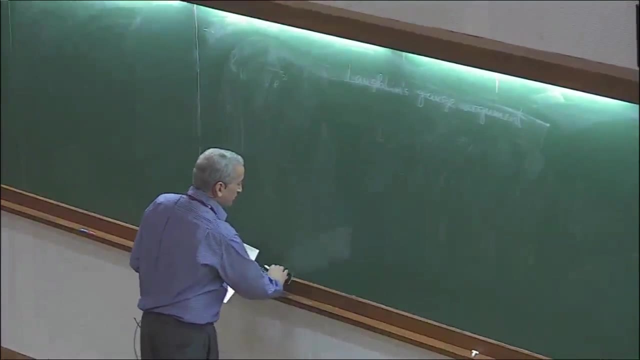 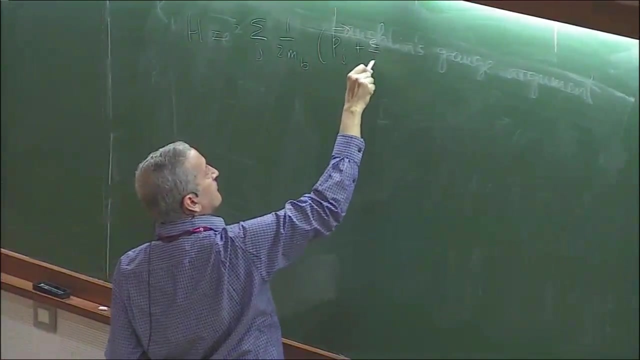 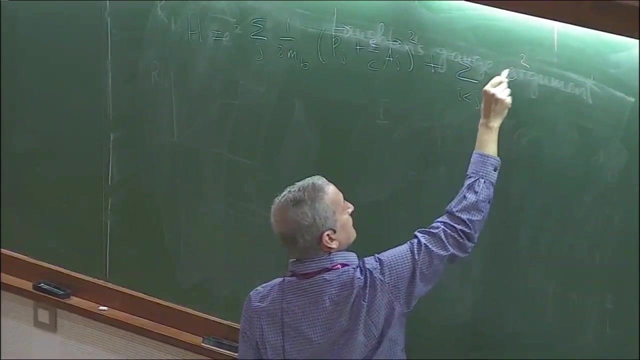 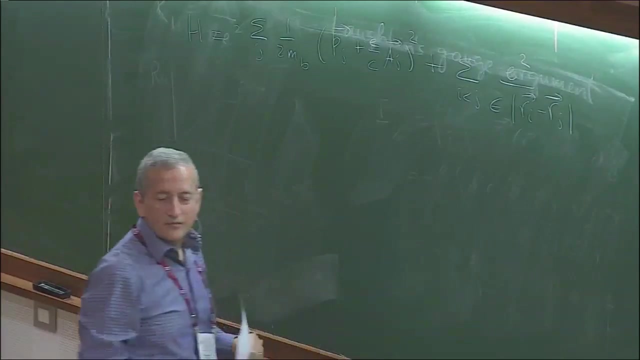 we get a fraction. So one has to introduce interaction to do that and therefore we are going to now write the following: Hamiltonian: Okay, that's our Hamiltonian And I will continue to assume that this is a Hamiltonian. Let us assume that the system is fully spin polarized, so we won't talk about spin explicitly. 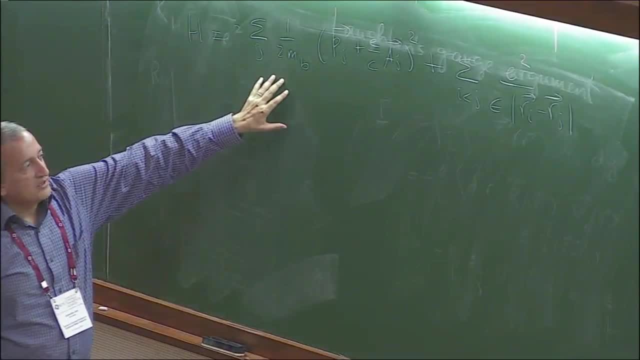 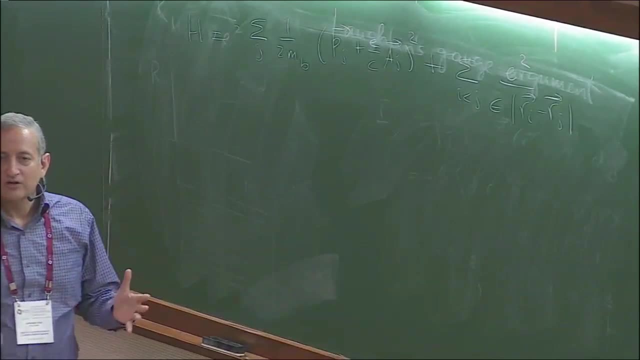 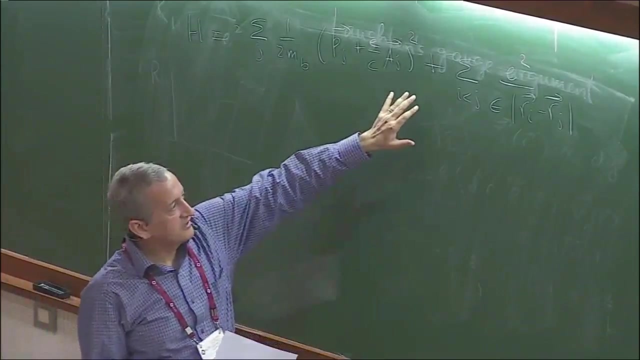 Now I am further going to make an approximation- that the magnetic field is so large, you know. So I want to consider a filling factor which is like one-third, you know, a fractional filling. So I am going to assume that the magnetic field is so large that that my interaction 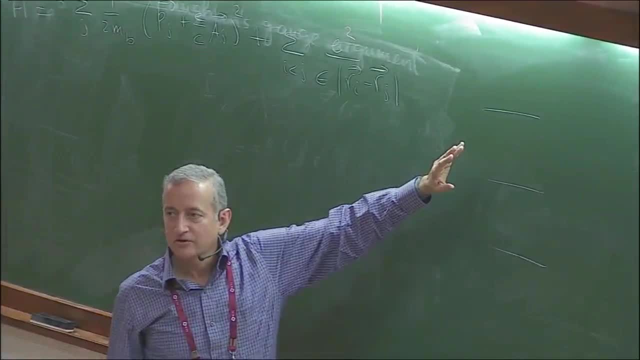 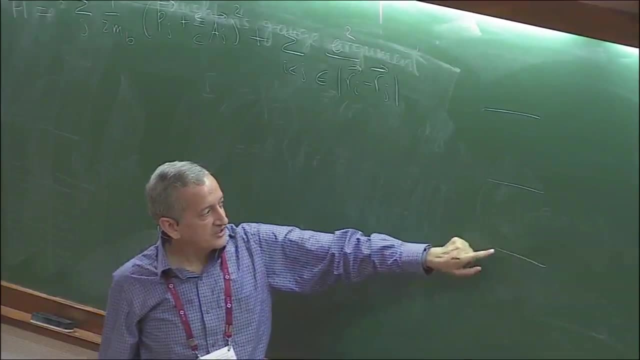 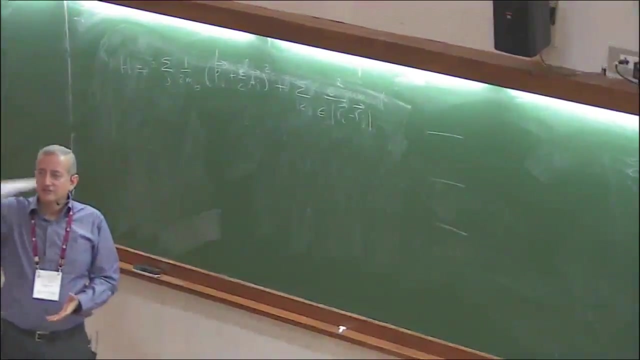 couple the system to higher lander levels. So of course, if there is no interaction, all electrons will go live in the lowest lander level. happily, Interaction can push them into higher lander levels. but we will assume that the cyclotron energy is, let's say, infinitely. 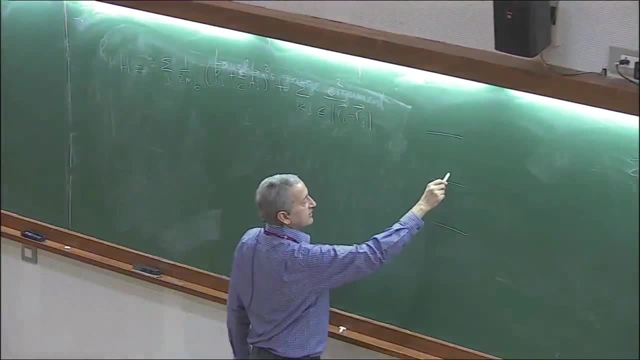 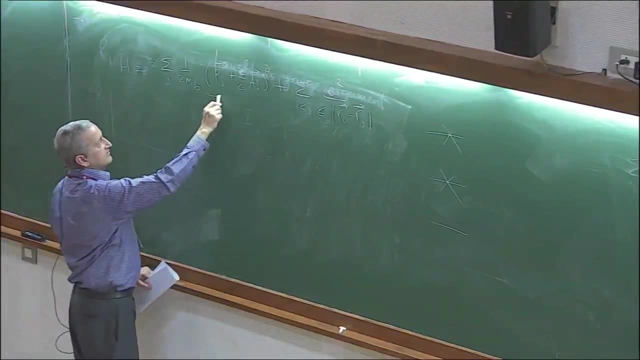 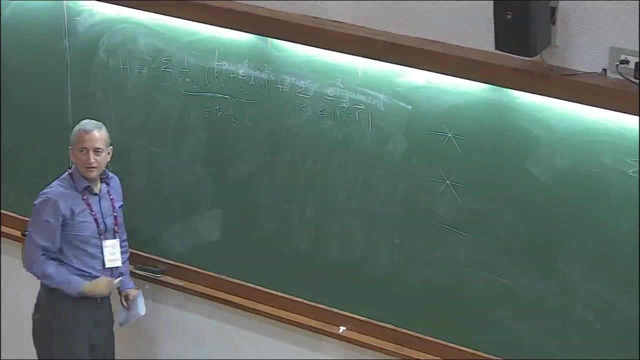 large. so therefore, we are going to throw away these higher lander levels, keep only the lowest lander level. and what does that mean? That means that this guy is precisely remember: the kinetic energy for the lowest lander level is just one half h bar omega c. so that's just a constant. and by taking some 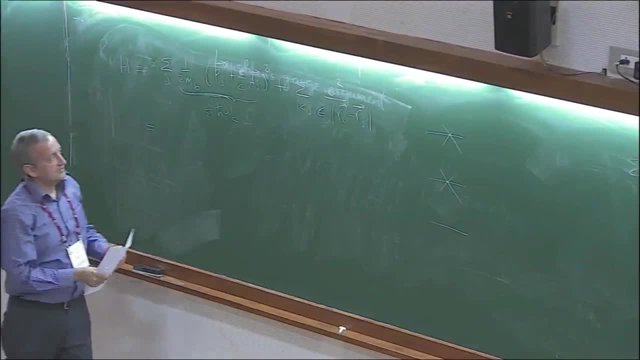 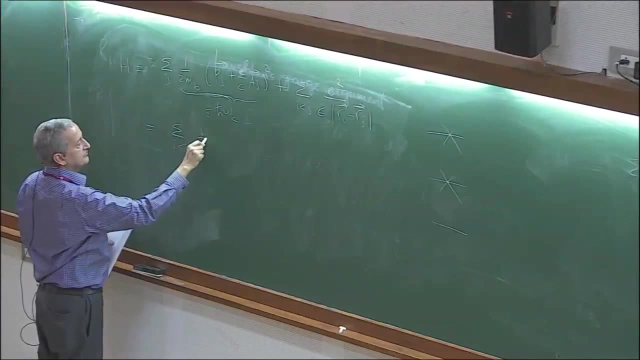 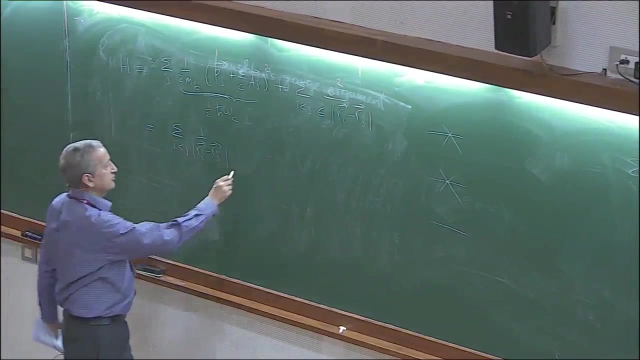 by choosing my constants, I mean my dimension of the energy, or unit of the energy. appropriately, i can write this very simple looking hamiltonian. okay, so that is the hamiltonian of the fractal hall effect. remember, we have to work within the lowest lambda level subspace. 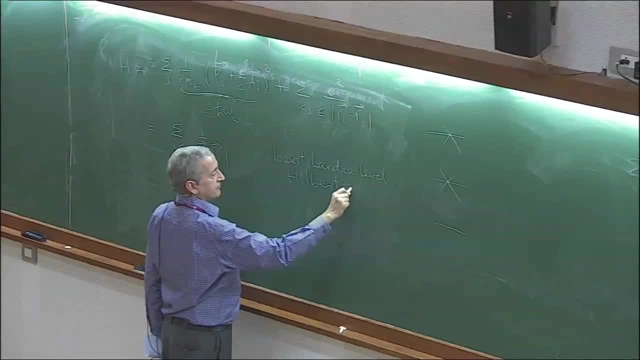 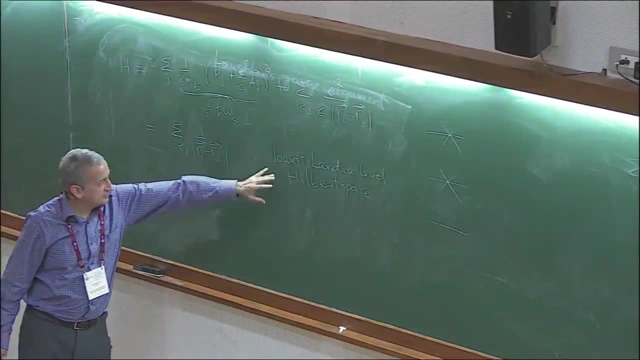 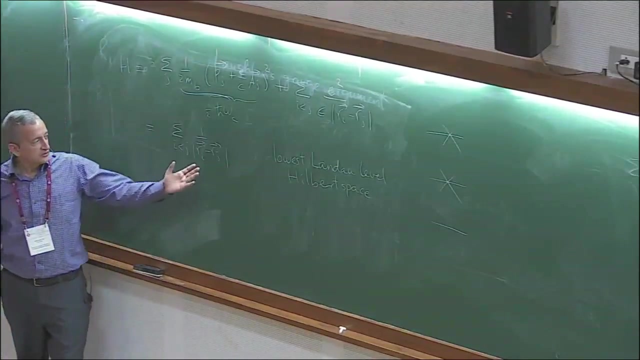 so in fact, this is crucial because if we don't think about it, you may say: well, there is nothing quantum mechanical about this, so all r's, they commute with one another and therefore it's just like a classical hamiltonian. but it turns out that if you restrict to the lowest under level, then x. 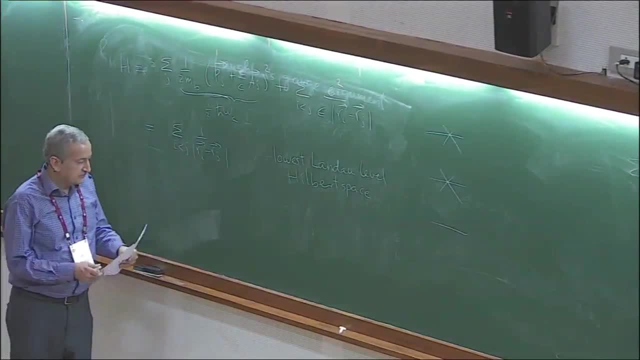 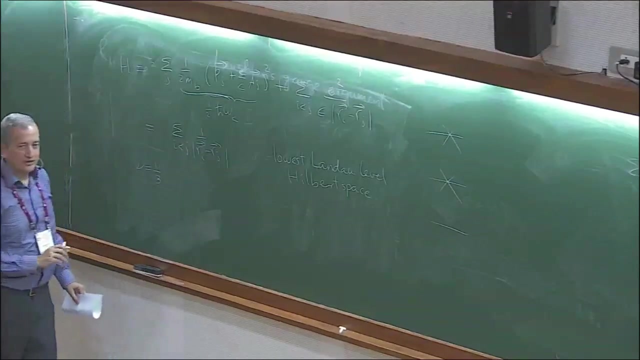 and y do not commute. uh, so, anyway, that's the problem. uh, now what does the situation look like? so let's consider filling factor one-third, okay. so first of all, by taking analogy from integer quantum hall effect, we know what we are trying to show. we are trying to show that somehow, because of interactions, we 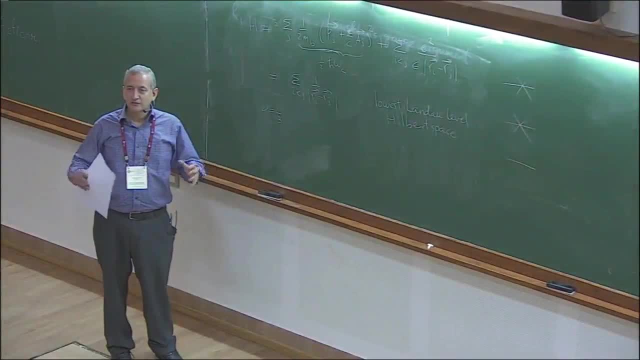 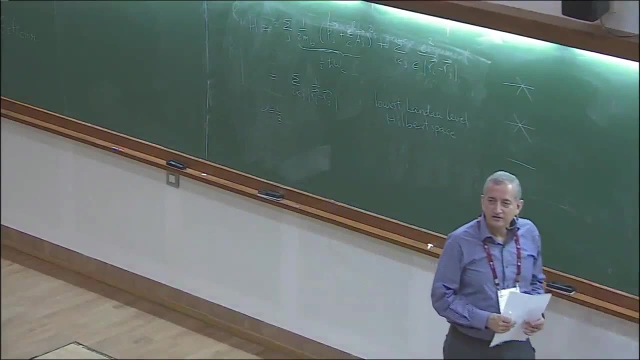 have a state of the art of the interaction and we are trying to show that somehow, because of interactions, we have a state here. it's a many-body state, but there is a gap to excitations. so remember an integer hall effect without disorder. the system had the property that whenever the filling factor is an integer, 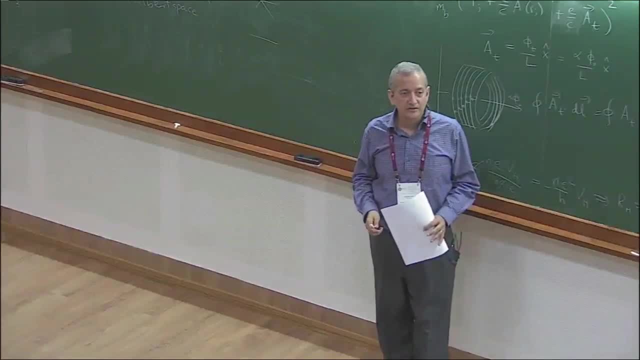 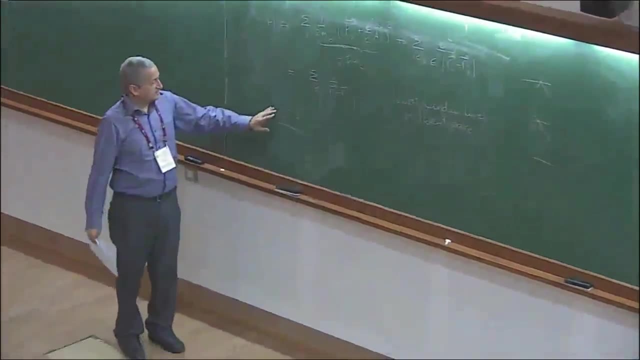 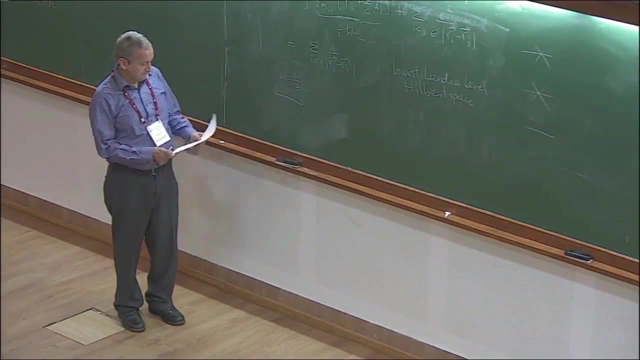 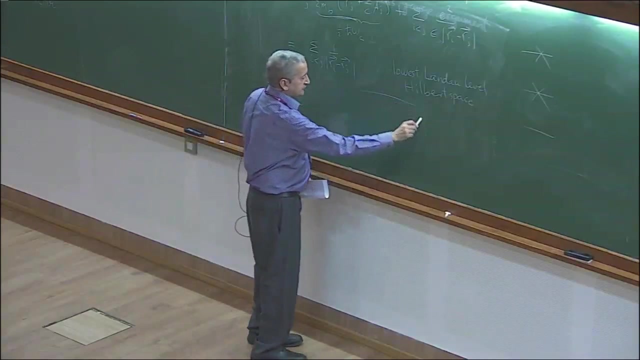 there is a gap to excitation. so you say the system is incompressible. so we would like, we are looking for a state that is incompressible at filling factor one third. that was the first fraction and that was seen. But if you are at filling factor one-third, that means if you take the 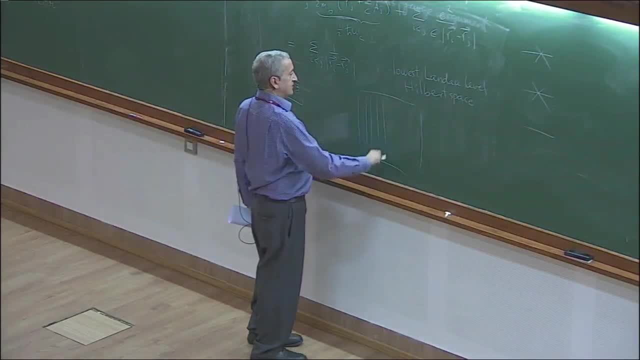 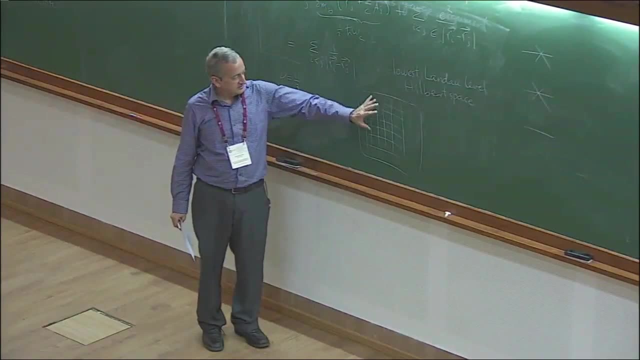 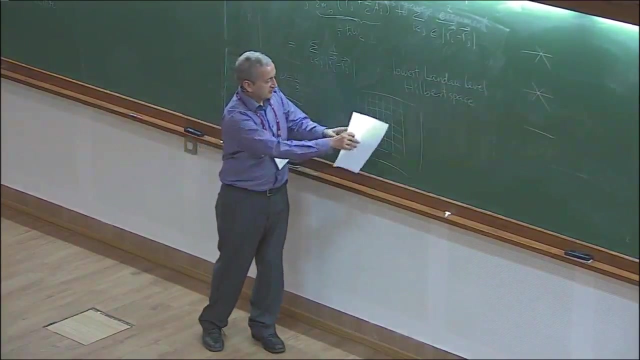 lowest lambda level and you know, if I make a grid which roughly tells me how many states there are degeneracy of the lowest lambda level, then the number of ways in which you can put electrons into these available states is huge. So you know, Vijay talked about 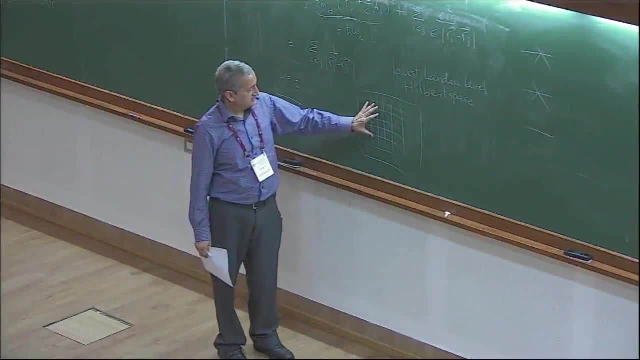 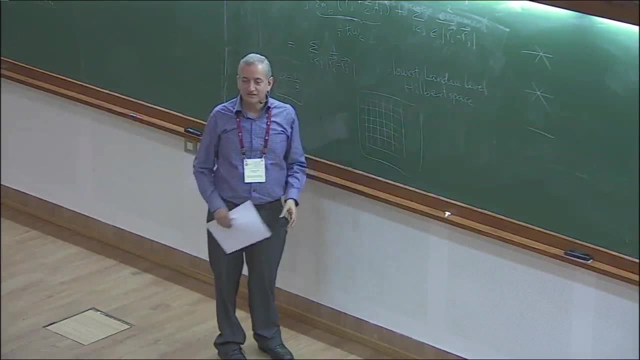 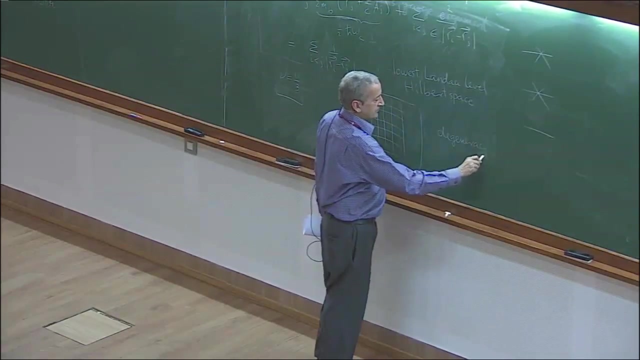 this earlier. So at filling factor one-third, the total number of available single particle states is 3N. okay, I have three times as many states as number of electrons and therefore the degeneracy of many body states. So I should say distinct number of many body states. 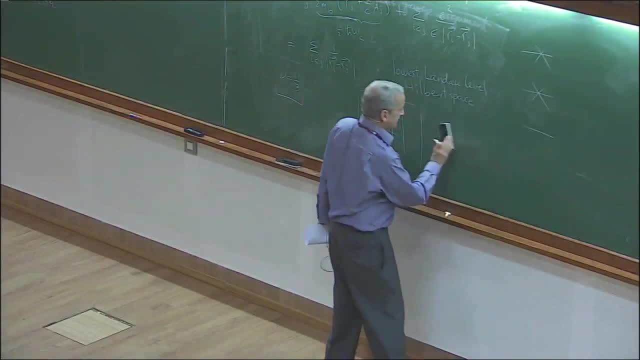 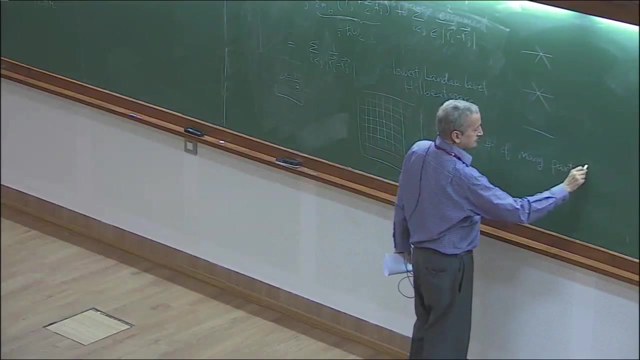 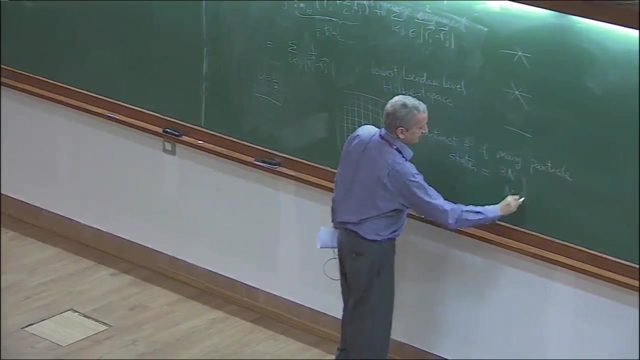 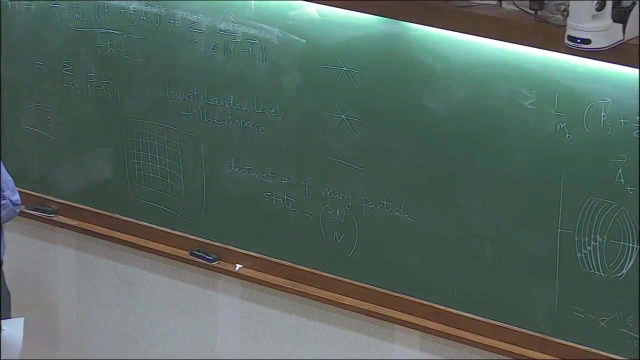 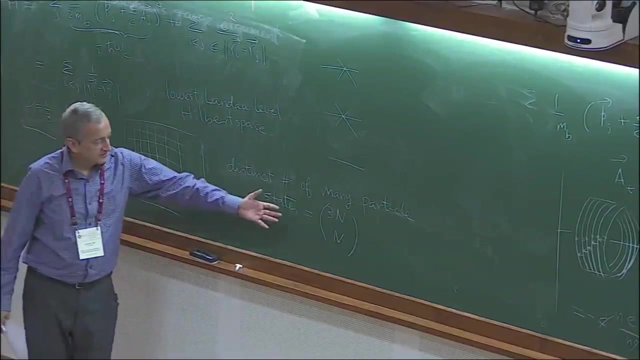 I should not say degeneracy, It's a… It's 3N chosen. And if you, you know, if you take N to be, you know, a number, a typical experimental number, which is like a billion, this number, 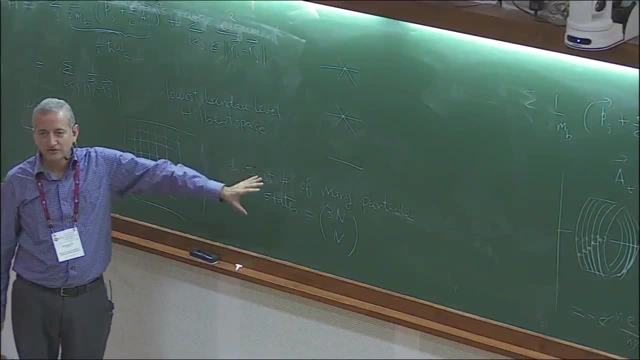 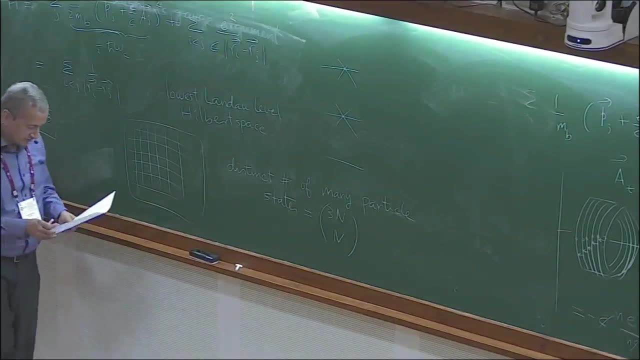 is enormously huge. okay, It's exponentially large, So we have a huge number of possible states. So the question is how to start to think about this problem. I mean, another thing we like is small parameters. So Landa famously said in one of his papers that the job of 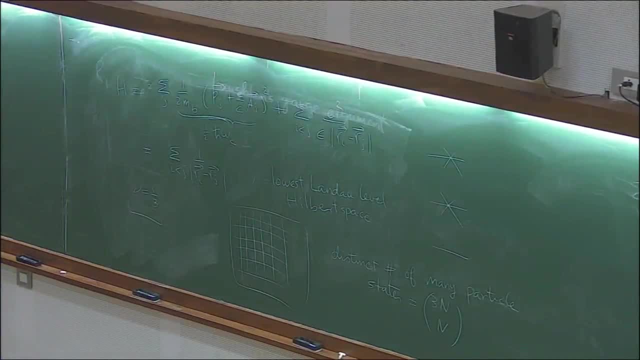 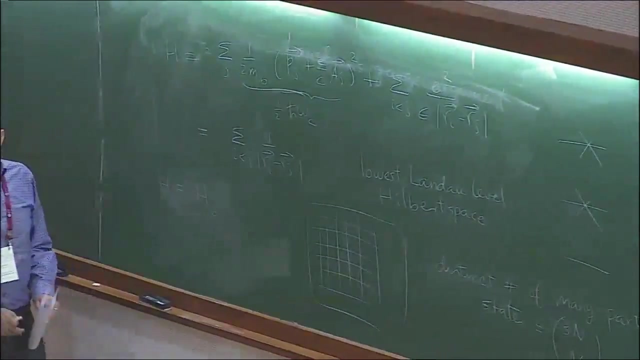 a theorist is to find a small parameter, because once you have a small parameter you know how to do perturbation theory. So typically, all the problems that we encounter, we want to write it as a sum of two Hamiltonians: one that we know how to solve plus something. 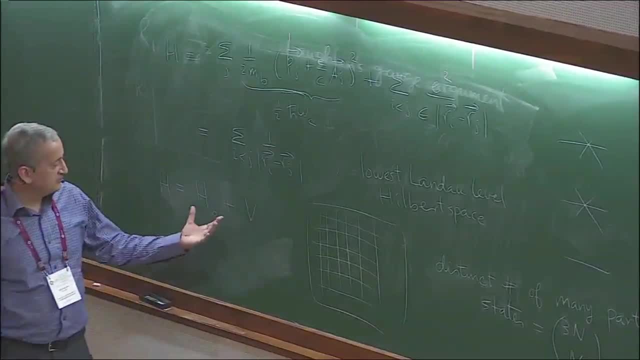 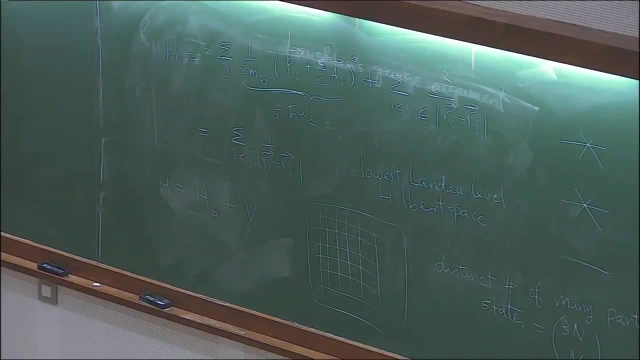 that's small, So we can do. we can do perturbation theory around this, but we don't have that. we don't have that here. So we I mean this: there is no H naught for this problem, So 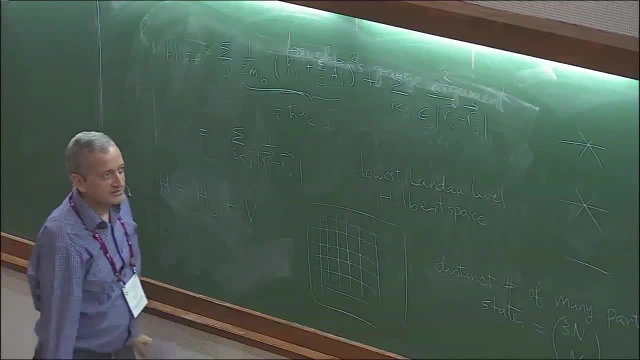 how to proceed So well. the method that Laughlin used is the Feynman method. You stare at the problem for a long time and you start to think about it. And you start to think about it for a long time and then you write down the solution. You have no idea how you 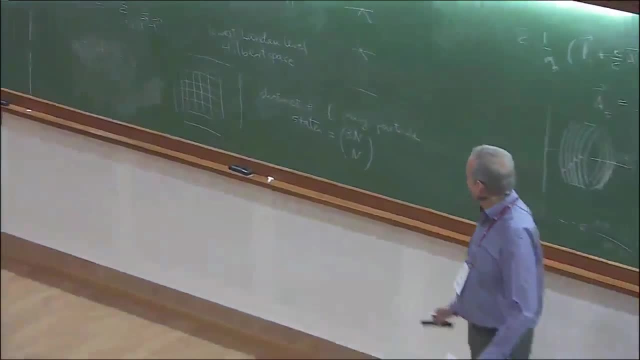 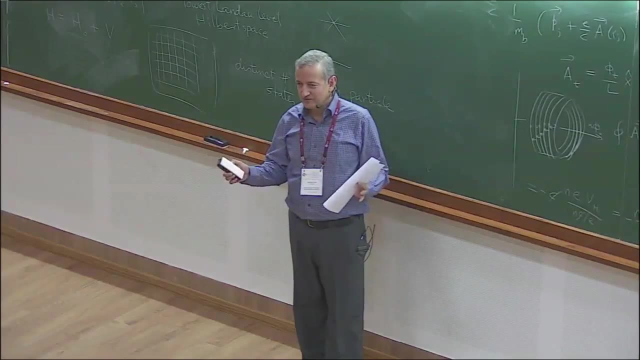 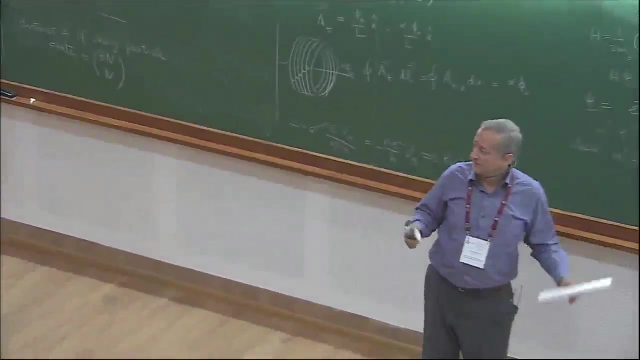 got the solution, but then you test the solution, So. so that's pretty much the approach in actual Hollywood. You have to look at the experiments, or by intuition you try to guess a solution and then see whether it really works. So Laughlin's approach was as follows: 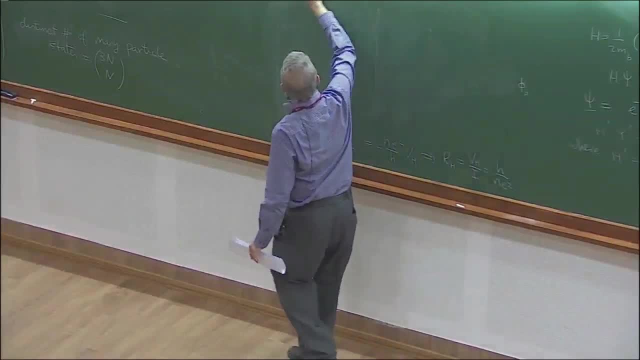 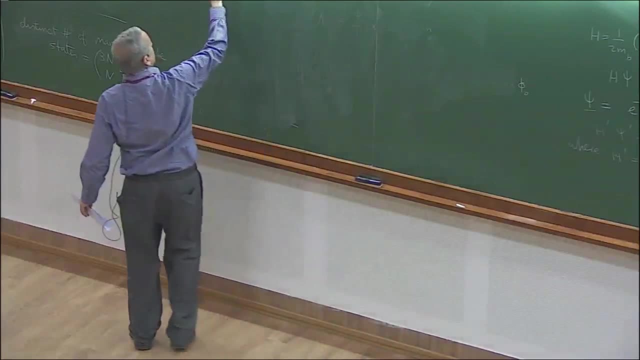 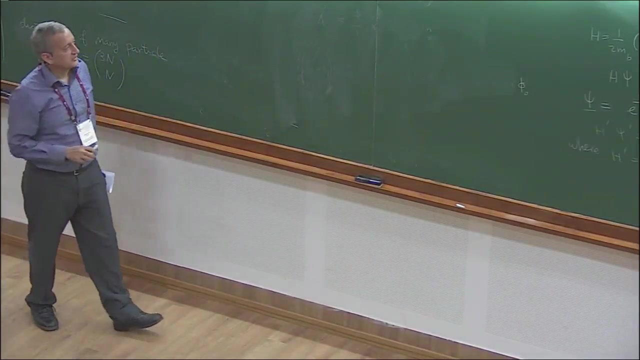 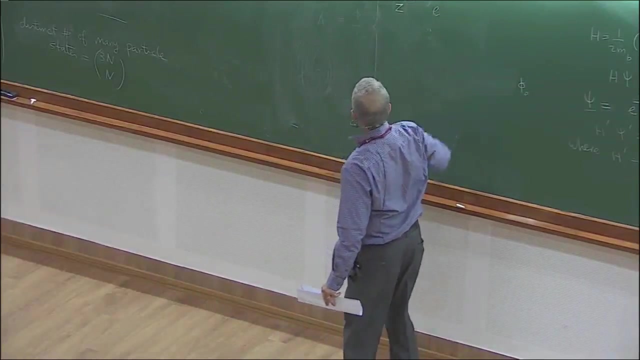 Okay, first of all he said that any wave function- so remember a single particle wave function- has the form z to some power times, a Gaussian factor. So the point was that in the lowest landed level it just depends. 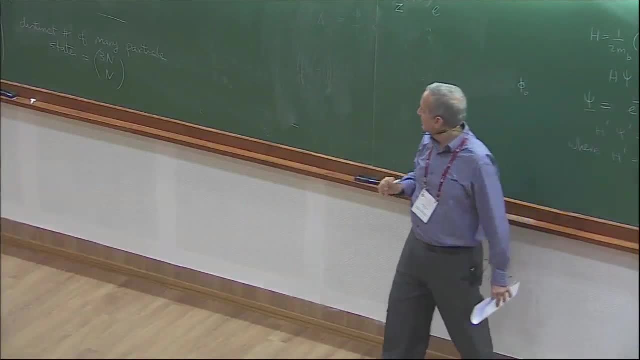 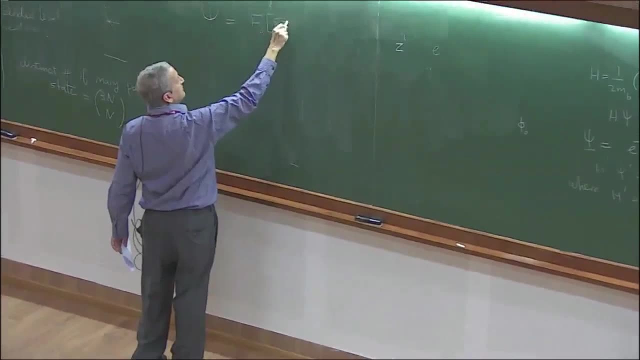 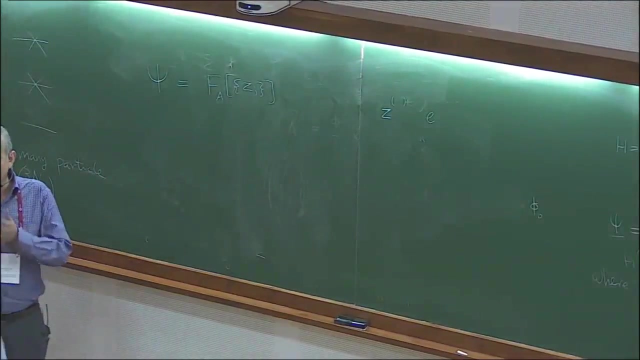 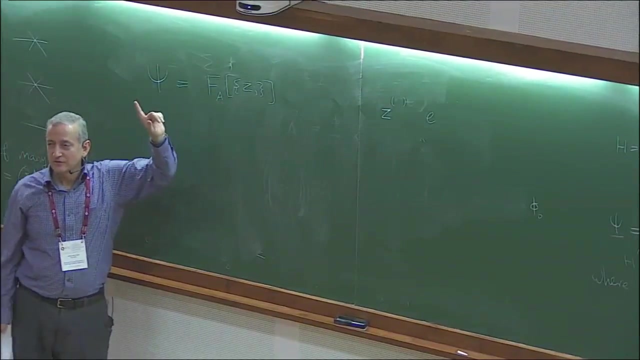 only on z. There is no z or r. So any wave function should be against constant fairence. function should be expressible times the Gaussian factor. I won't write down the Gaussian factor explicitly, So any wave function is some polynomial of the z's, no z powers. 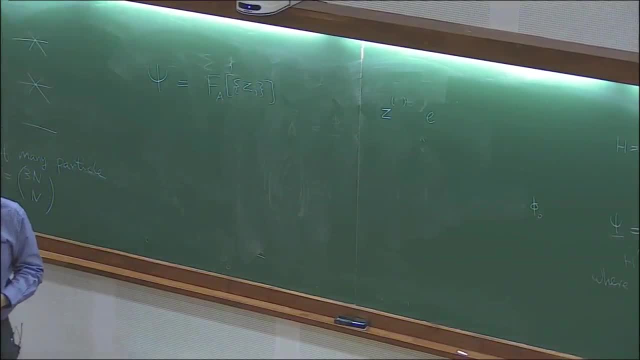 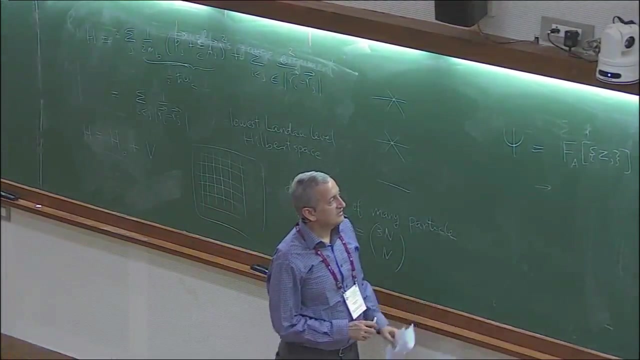 So that's an exact statement for any lowest land level wave function. Now, the main assumption that was made was to say that this has a Jastrow form. Now, Jastrow form is something that has been used in nuclear physics. it's used in helium physics, and what it says is: 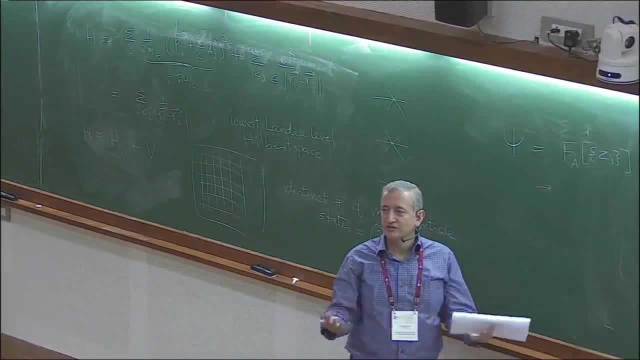 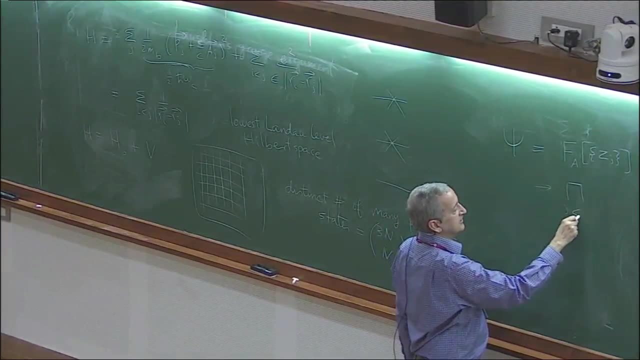 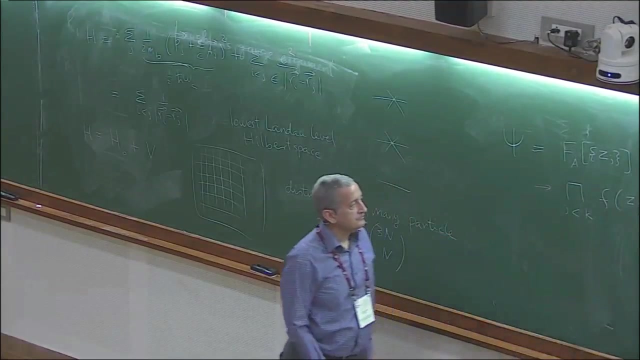 that the I mean. so we have to include some correlations between particles and we are going to do it air wise. We are going to say that this wave function has the form and we are going to say that it has a Jastrow form. It's an assumption And we will see. 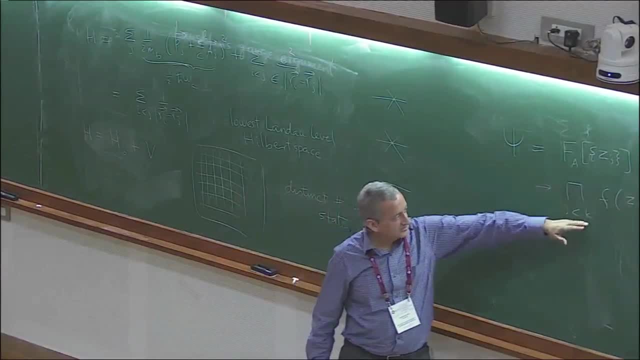 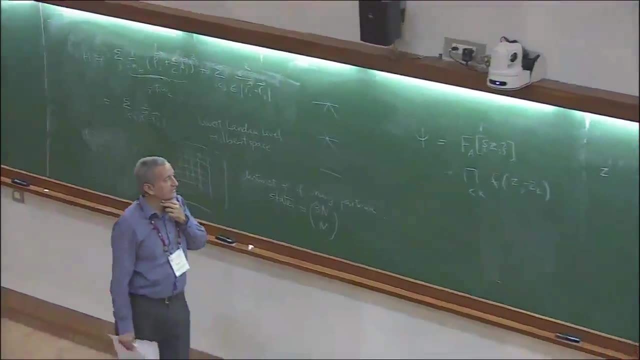 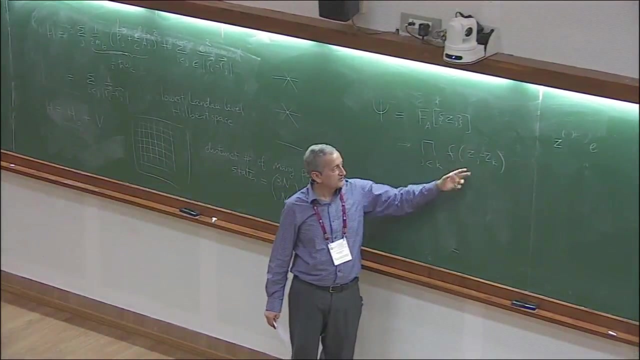 that in general, general fractional Hall states cannot be written in this way. They have much more complicated structure, But we'll see that at least some fractional Hall states can be written in this way. Is this clear? So I'm trying to build correlations, air wise. 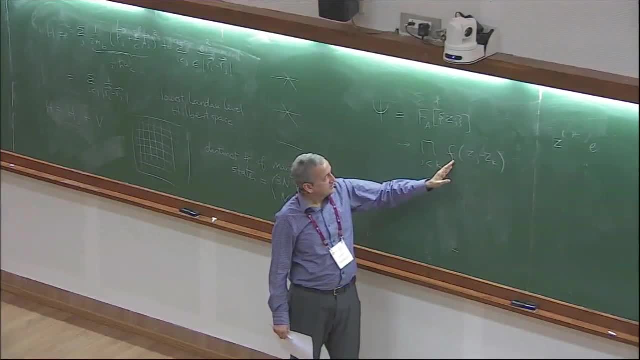 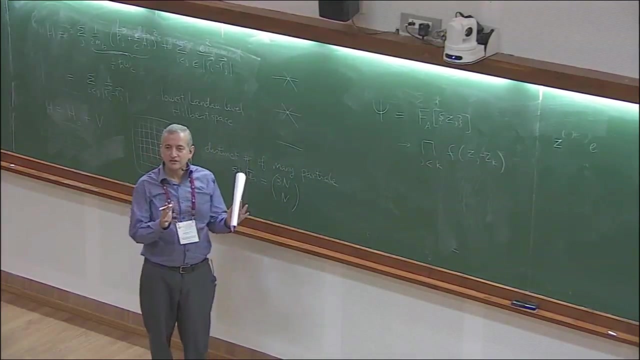 I take all pairs And write some wave function for each pair And then take product of all those. Now the third assumption, or it's not an assumption. it's really saying that we want to make sure that the, that the wave function is an eigenstate of the total angular momentum. So what does? 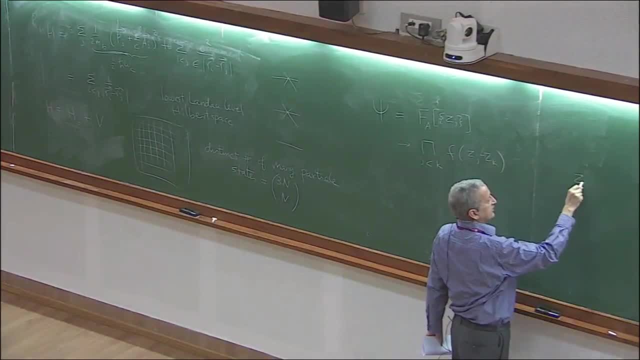 that mean, Remember, z to the power m has angular momentum m. If I have two particles and let us say I want angular momentum 4, I can write z 1 to the power 1, z to the power 3 and I can couple it to z 1 to the power 0, z to the power 4. 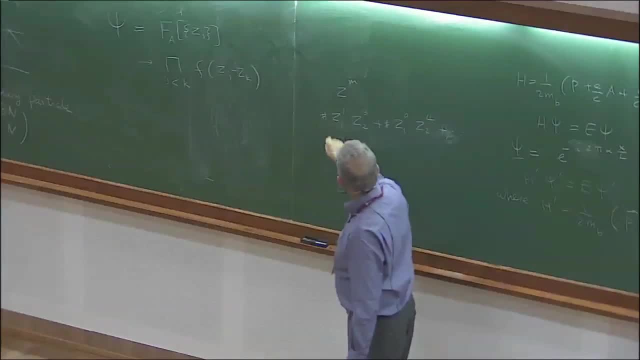 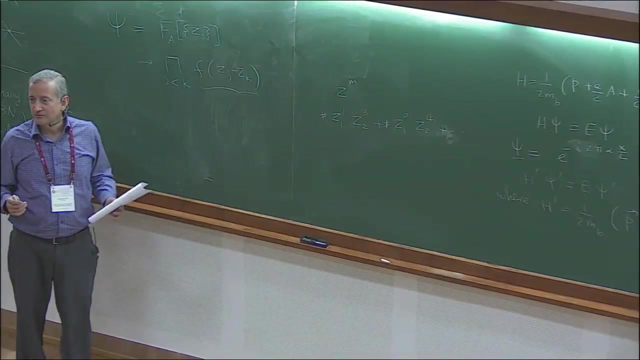 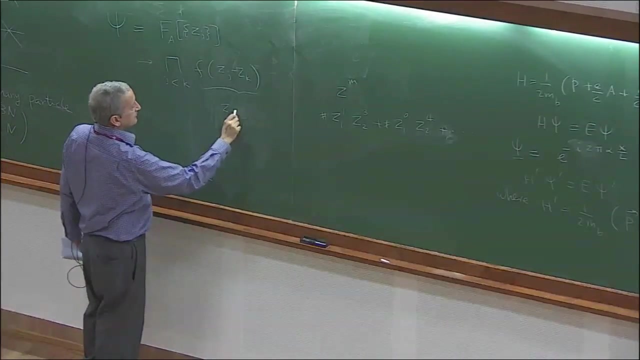 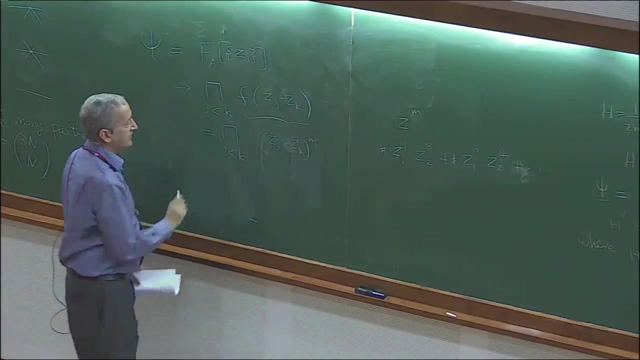 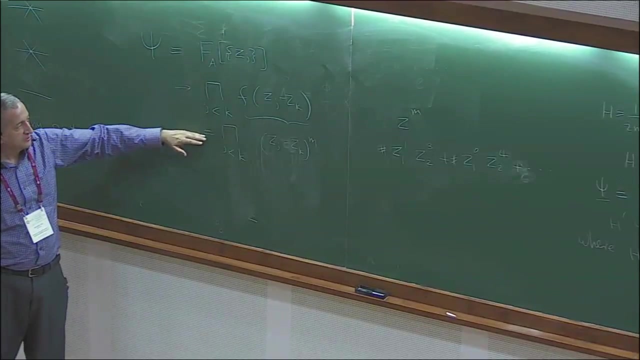 and so on, with some coefficients. So the total degree of the polynomial must be the same. What that means is that each of these guys should also have a well defined angular momentum. So therefore, the only possibility you have…. So the first step follows, by assuming that it has a gesture form. The second step follows. 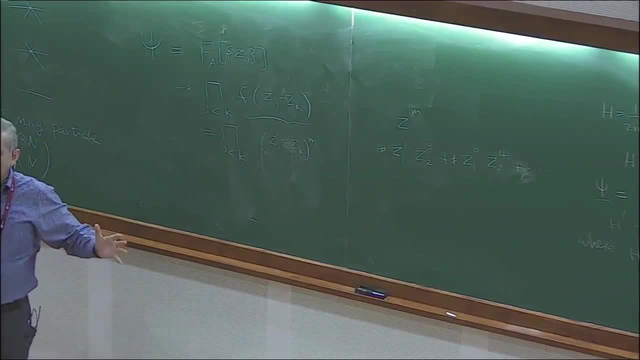 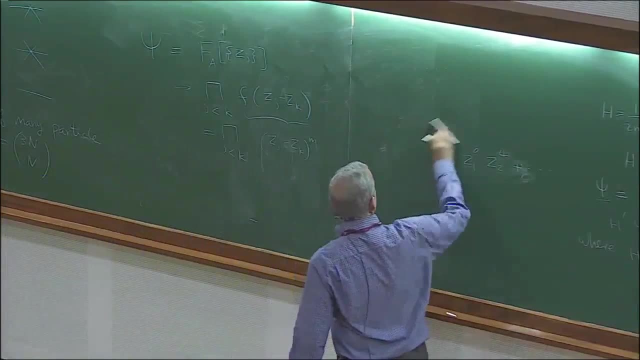 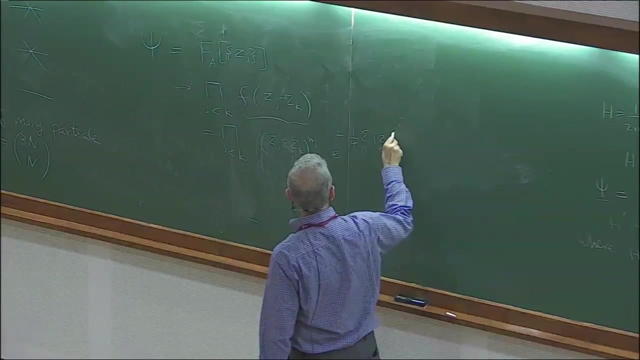 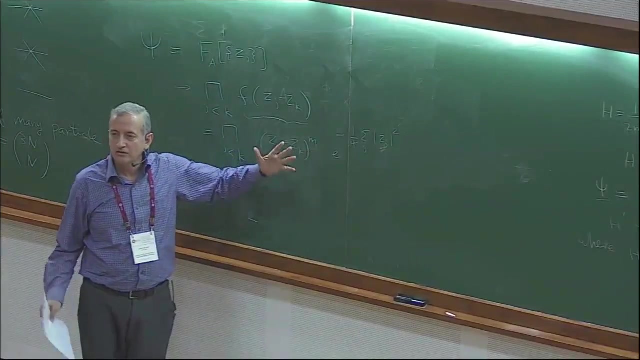 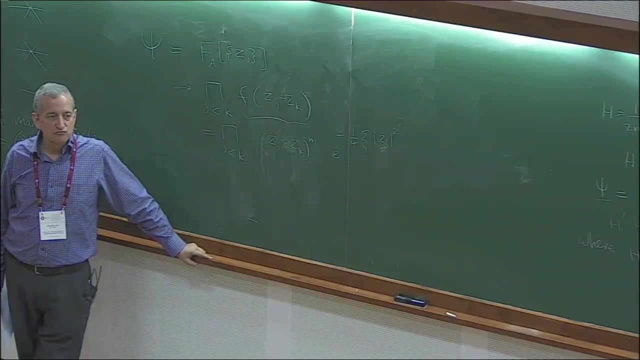 … by assuming that you want the total wave function to be an eigenstate of the total angular momentum. And let me put back the Gaussian factor. And then you ask the question: what is this m? Is there a constraint on m? What values can it take? 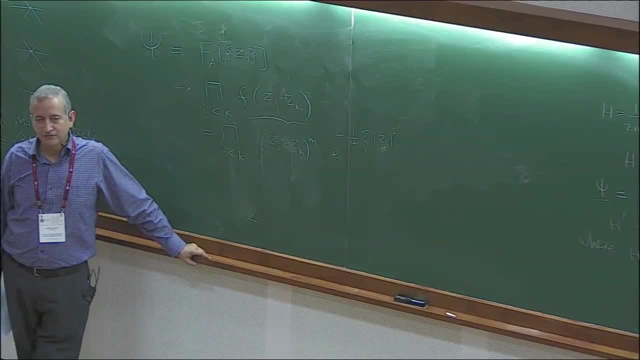 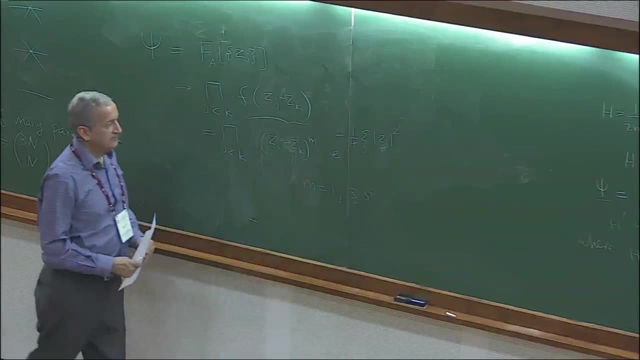 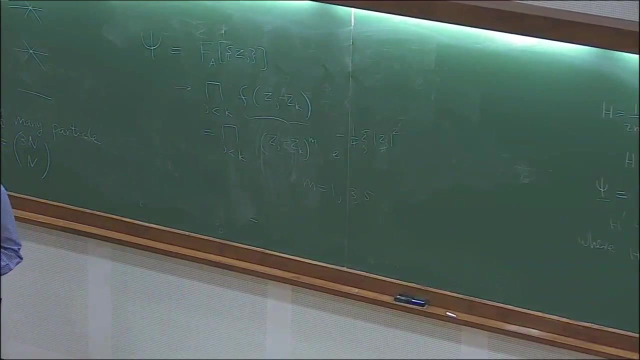 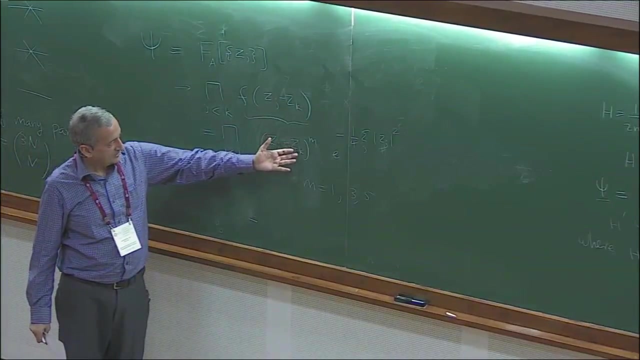 m must be an odd integer, So m can take values 1,, 3,, 5.. If I put m equal to 1, does it take and describe any state Filling factor 1.. So Laughlin said we can put m equal to 3,. 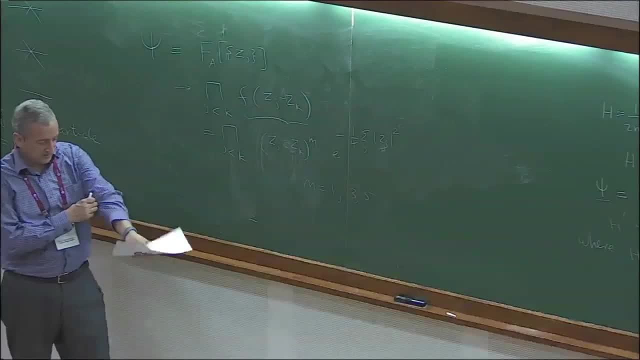 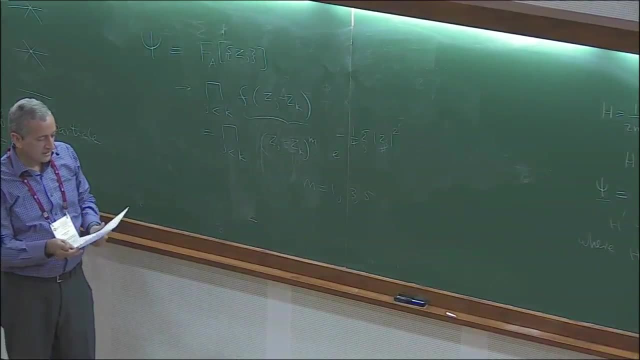 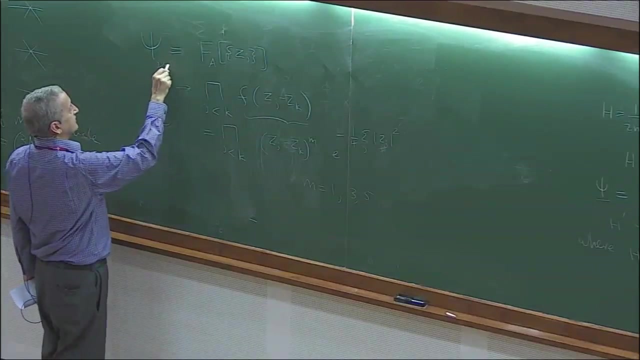 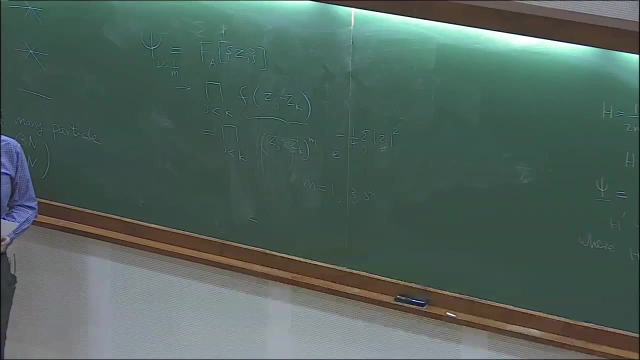 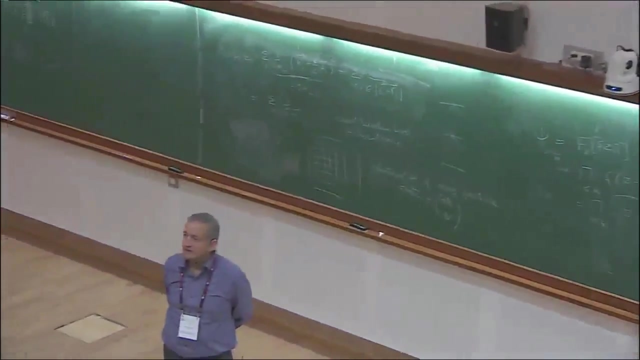 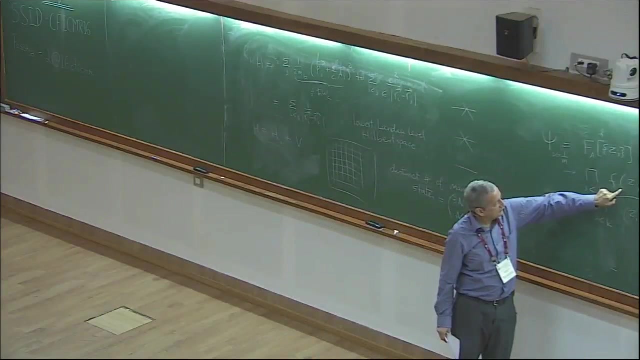 m equals 5, and so on. And tomorrow I'm going to show that this state actually describes a state at filling factor 1.. Filling factor 1 over m, In fact, let me let me, yes, So what we assume when we write Jastrow form? we assume that this f is the same for all. 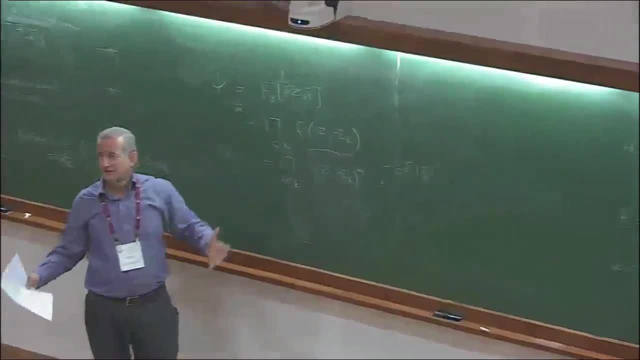 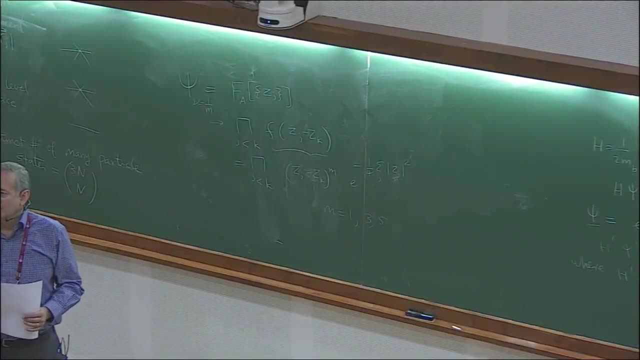 pairs. OK, So that's Jastrow. Is it the same for all pairs? No, because you have to assume that. I mean there is indistinguishability, so all pairs have to behave in the same fashion. So if you play with this, you will realize that. 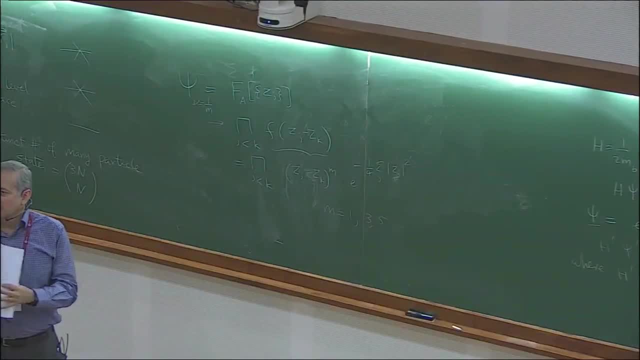 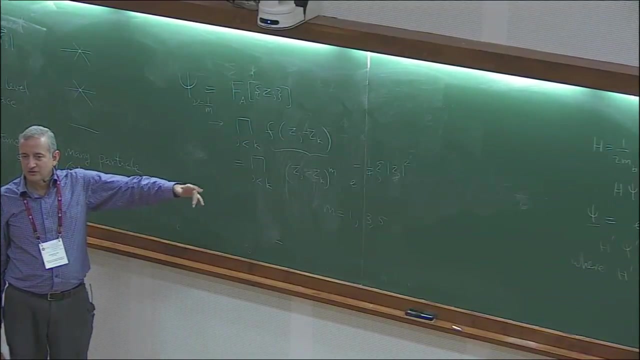 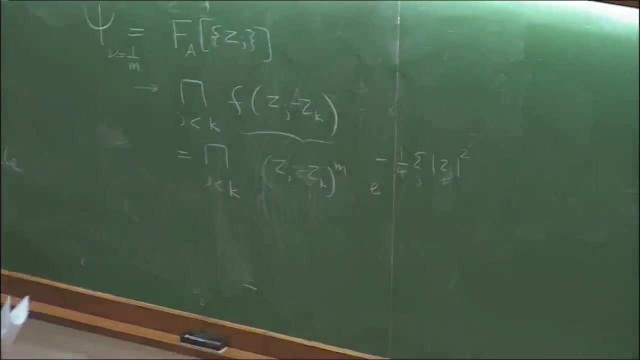 it doesn't work. OK, let's let me just calculate the filling factor very quickly in a cheap way, and then we can go on to some problems and solutions. So the answer is yes, we can. OK, So I am going to assume that this wave function is uniform. I have not shown that. I am going 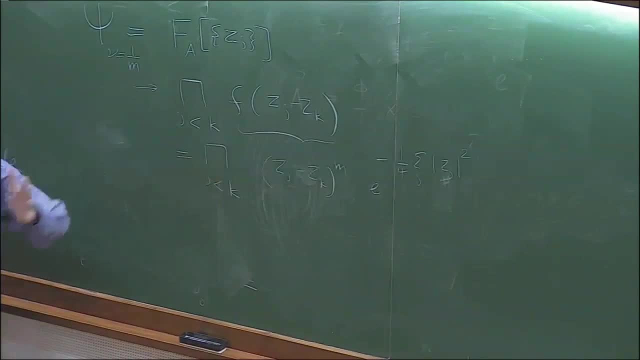 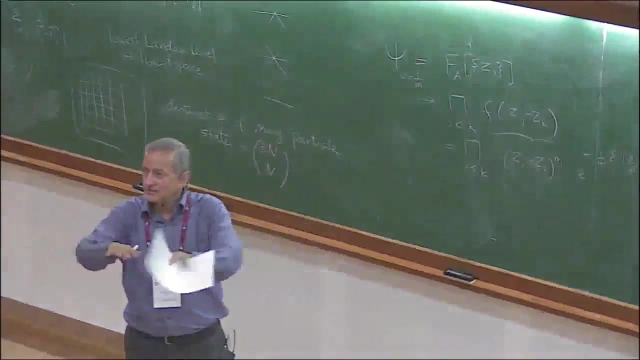 to assume that if you plot the density of this, which you can do on the computer, then it is going to be uniform density modulo edge effects. So it is going to represent a disk of some radius, okay, but inside it is uniform, Density is uniform. So let me assume that. 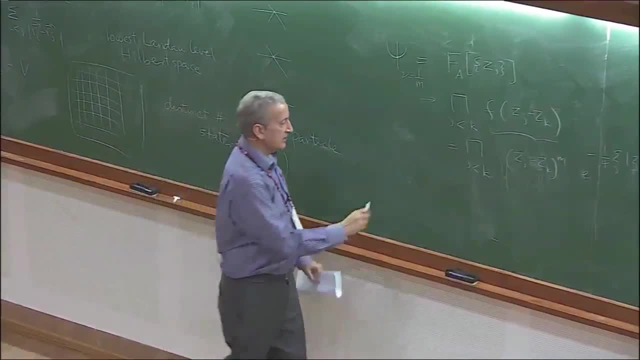 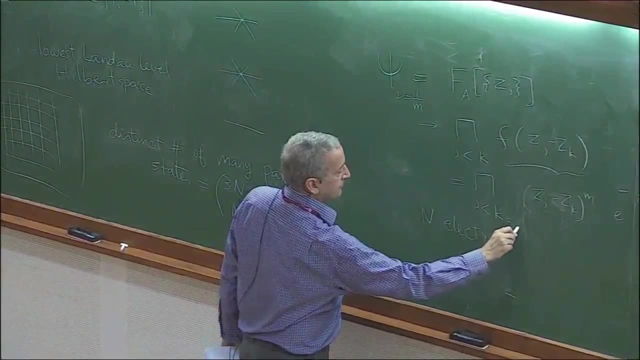 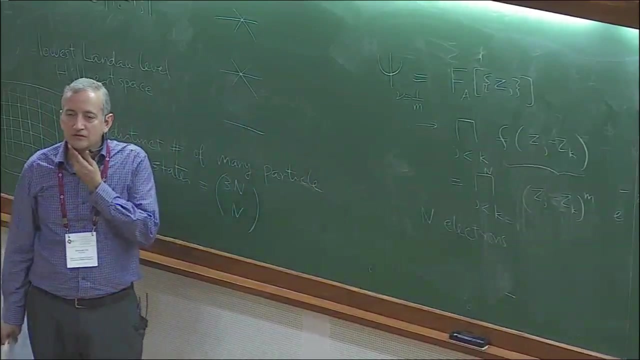 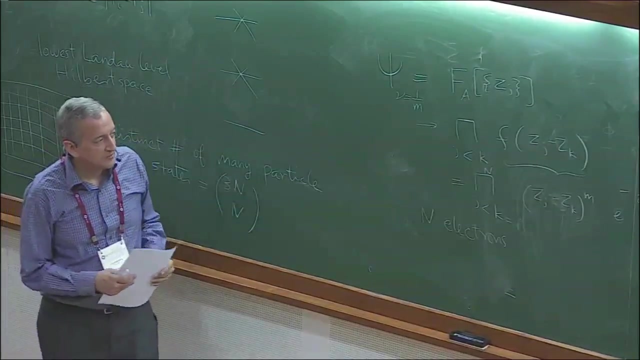 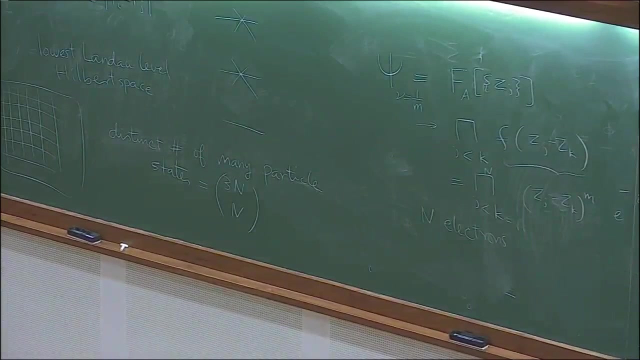 Then how do I calculate the filling factor? So let me assume n electrons. So can someone tell me how many states are there in the disk? Okay, let me give you a hint. So let me just do the problem, because if I give you, 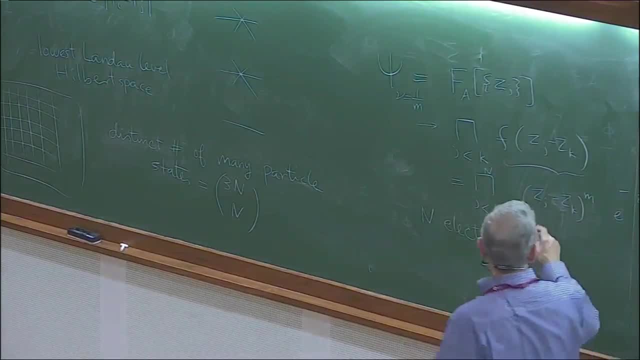 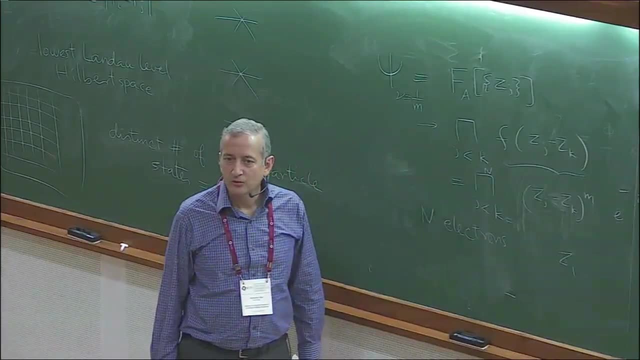 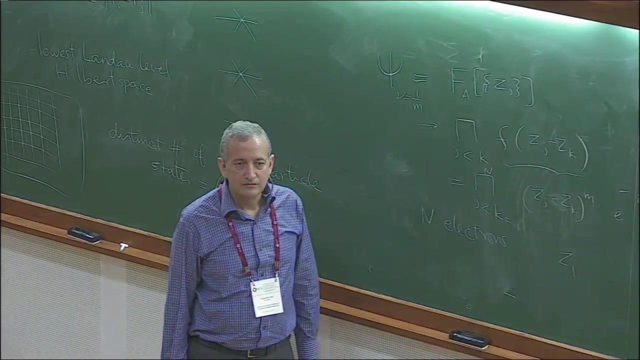 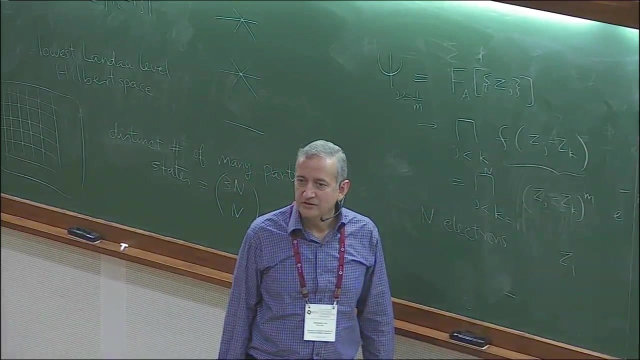 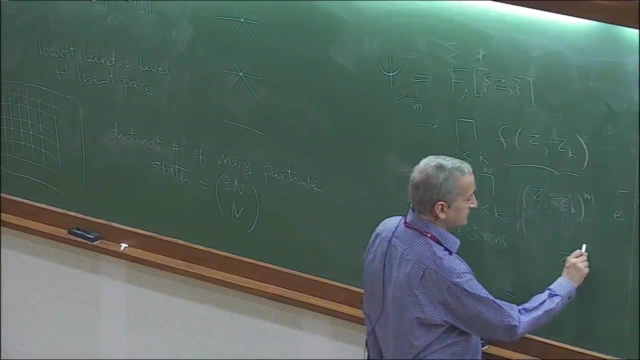 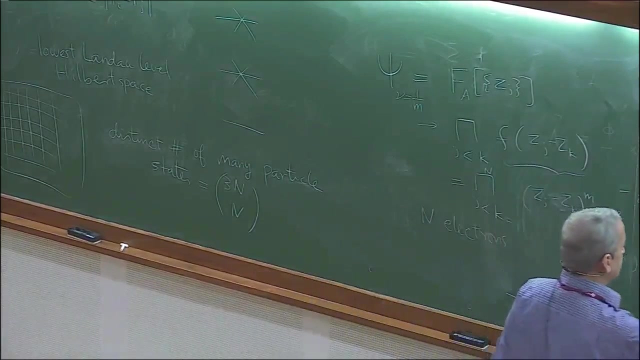 a hint, I will effectively have done the problem. So look at the largest power of, let us say, z1.. What is the largest power of z1?? Sorry, speak up N times m. This is correct. So because you can see if I write all the. 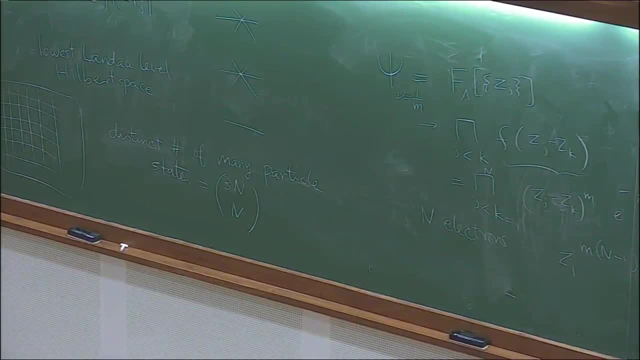 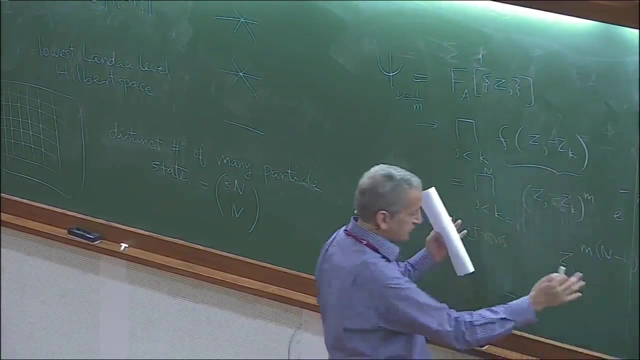 terms which include 1.. So from this you can see, largest power of z1 is. So there are n minus 1 factors and you can get. So the largest power is m times n minus 1.. So the total number of states. 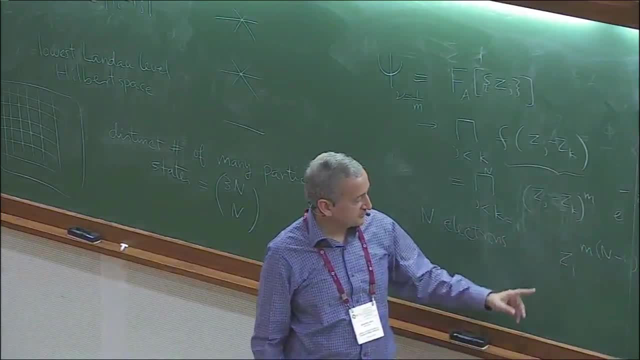 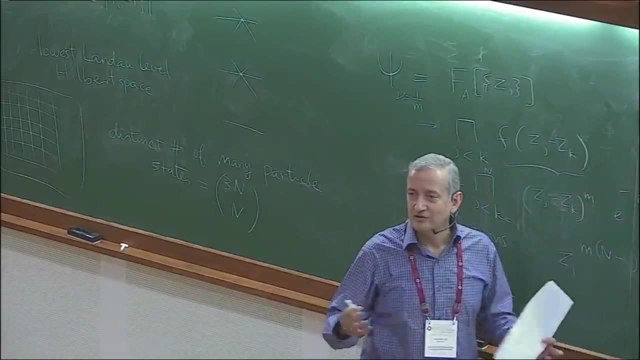 in the disk. So the smallest power is of course 0. So the total number of states is m times n minus 1 plus 1.. Okay, counting the 0. So the filling factor is equal to the number of particles divided.